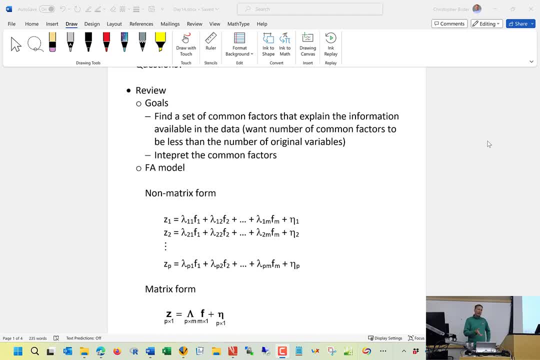 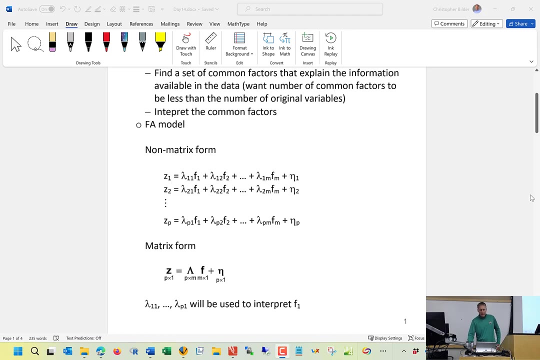 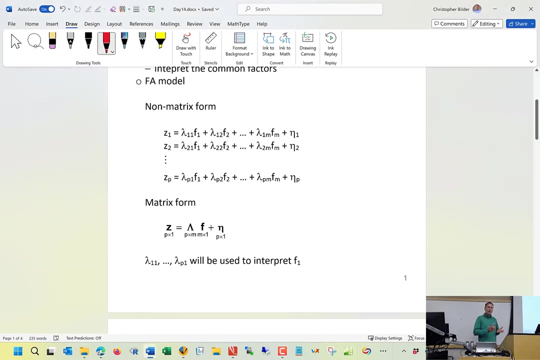 And then also, we want to be able to interpret these common factors. So we can see that we have goals that are very similar to what we had with principal component analysis. How we accomplish these goals are different, And so we set up the following model, And again, I presented to you a few different representation of the model. Here's just the most widely used representation where on the left side of these equations here we have our standard. 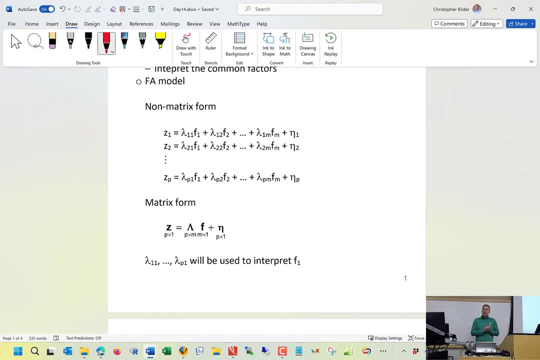 standardized variables And on the right side is our assumed structure about. how did these variables, how do the variable values, actually come about? So if we take a look at our first- let's call it original- standardized variable Z1,, we're saying that's equal to lambda 1: 1, which is a constant. It's a parameter that we want to estimate. 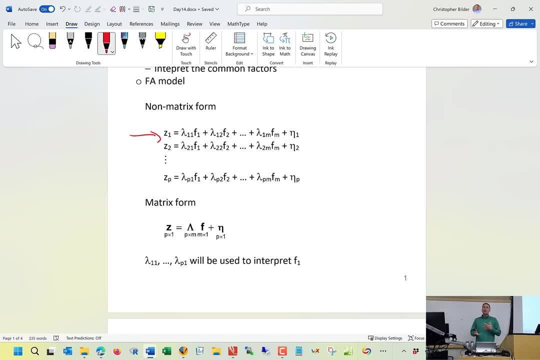 Times, F1, which is our first common factor, Then plus another constant, lambda 1, 2.. These constants are called factor loadings Times, our second common factor, F2.. And let's say just to be general, we go all the way up to the m-th common factor. 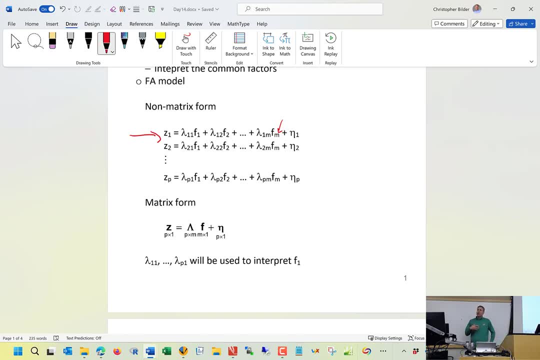 And then, finally, we add eta 1, which is called a specific factor, to it. And so if we knew those lambdas, if we knew those Fs, if we knew those etas, we know what's going on. z1 is, and then we also have a similar equation for the second standardized 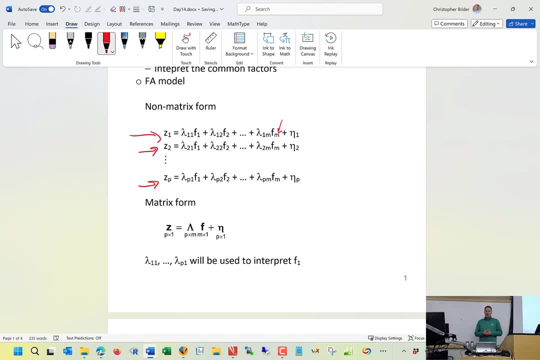 variable all the way down to the P standardized variables. and if we look at just one of those equations, we can see how this is very similar to what we see for regression model. the differences: well, let's talk about the similarities first. these lambdas are kind of like what we think of as our betas for 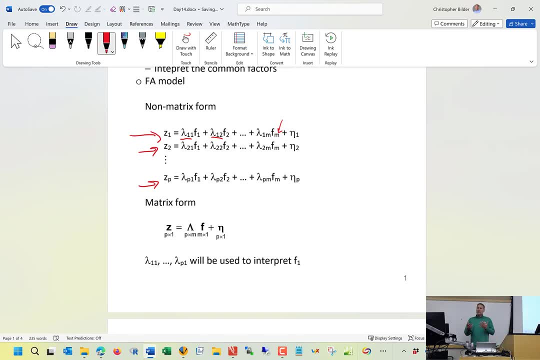 regression model. we want to estimate them. these lambdas give us a lot of good information about what these F's actually represent. so if a lamb, if lambda 1, 1 was equal to 0, and that says there, there's essentially, essentially that F 1 does not have an effect on z1. if lambda 1, 1 was positive, says it F 1. 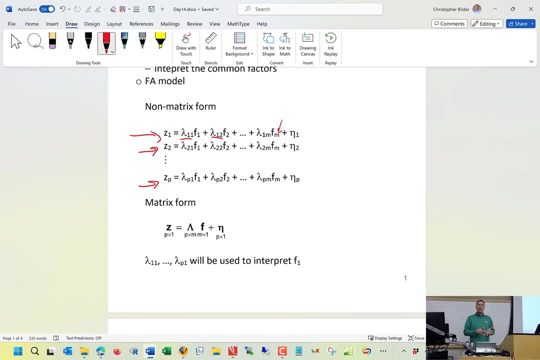 has a 1, 1 has a positive effect. if lambda 1: 1 is negative, says that F, 1 is has a negative effect and the also, then the a. that kind of plays the role of our epsilon or air term in a regression model. now continually talking about this. 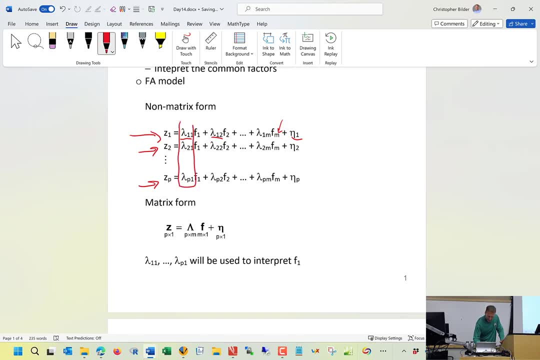 interpretation idea now, since we actually have P different equations and notice how F 1 is in each of those P different equations. that's what's called a common factor: common, all the original variables. to interpret this F 1, all we need to do is take a look at its corresponding lamdas. 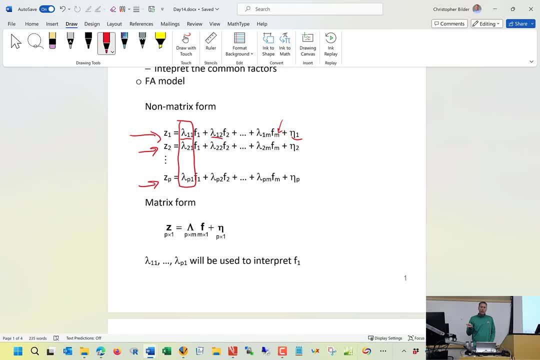 and so, for example, let's say, if lambda 11 was 1, lambda 21 was negative 1 and all the other lamb lambdas corresponding to F 1 was 0, then we would say, okay, well, F 1 is represented is essentially a comparison of our 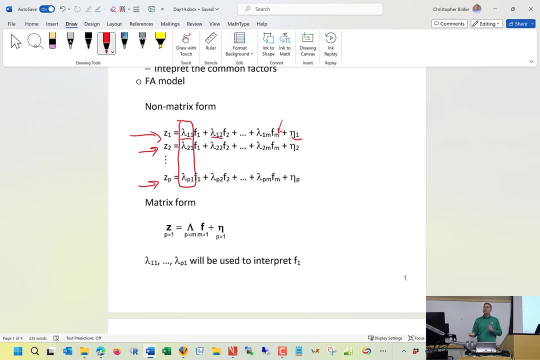 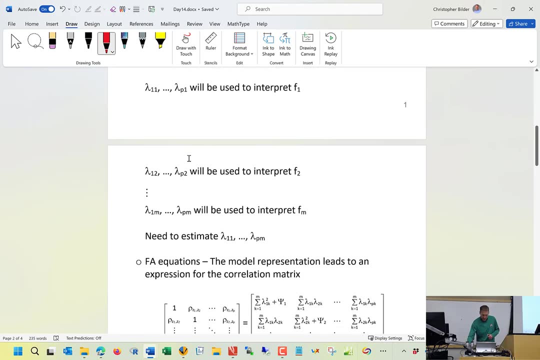 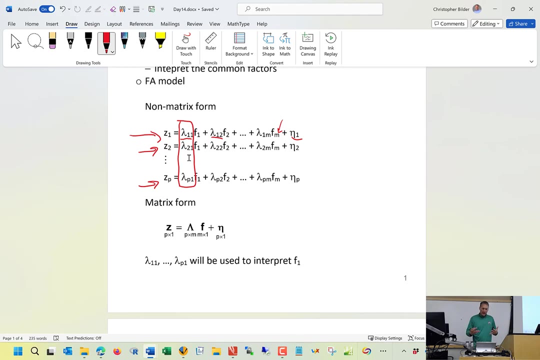 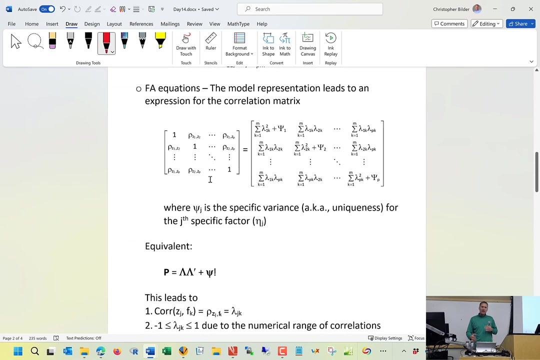 contrast between z1 and z2.. Let's see if I talked about all that Yep, And so we can also put this, these p different equations, into a matrix like form as I show there, And because of this assumed model structure we can actually come up with a representation for our 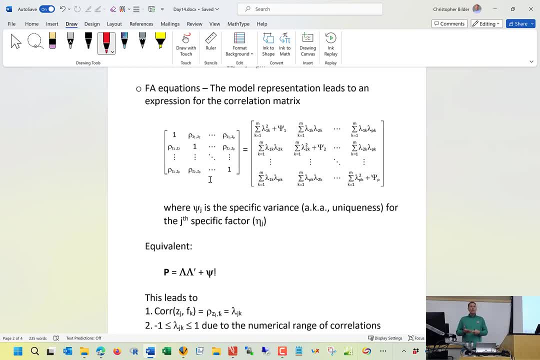 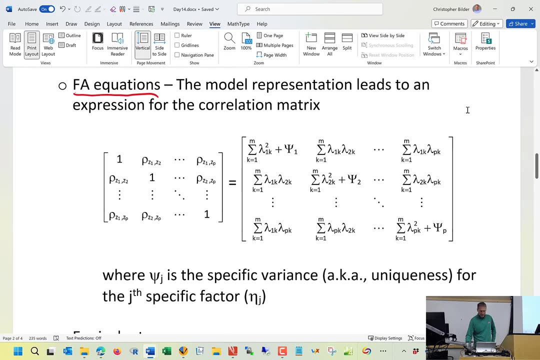 correlation matrix or, equivalently, our covariance matrix for the standardized variables. This expression, for this correlation matrix, is what's called the factor analysis equations. Let me make this a little bit bigger so we can zoom in. And so- and you're not- not responsible for the derivation, about how this comes about, but you are. 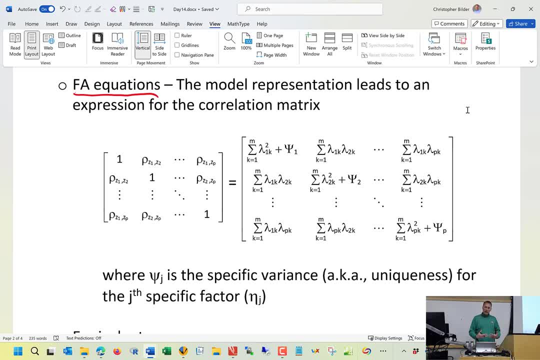 responsible for understanding the components of this expression. So, for example, if we look at rho, sub z1, z2,, this represents the correlation between the first standardized variable and second standardized variable. This expression says it's equal to the sum of the product of some lambdas. 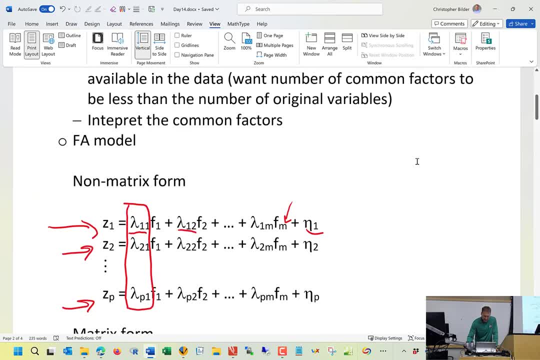 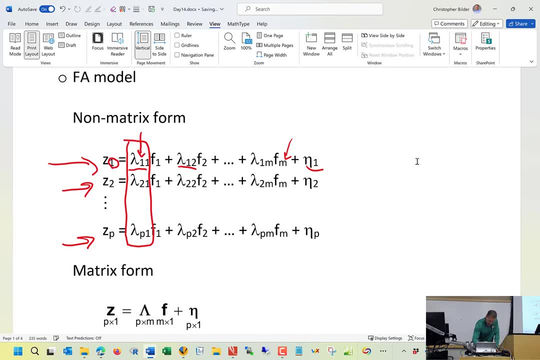 Now let's go back to our model. Which lambdas are they? Notice when I have a 1 here for z. I always have a 1 in the first subscript for the lambdas. Look at this subscript 2, notice in the first subscript for the Lambdas I always have a 2.. 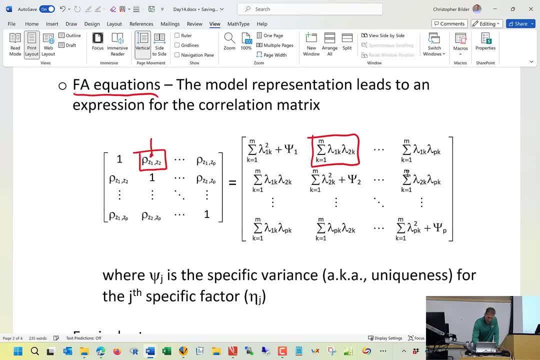 And so notice I'm looking at z1, z2, so that means Z1, ز2, XZ2, by Z toward This key. here Now you can see that the symbol J denotes the number of theкон的All of them. 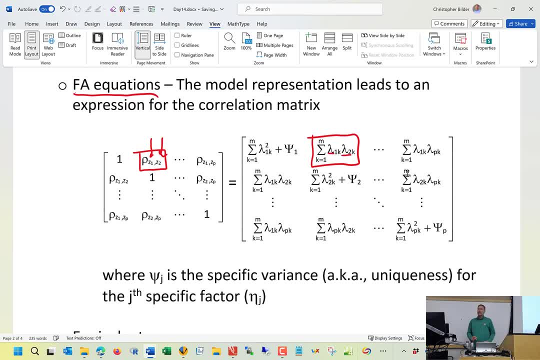 And so we're going to talk about means. I'm taking the product then of those corresponding lambdas for z1 and z2. that represents the correlation between them. then on the diagonal elements of the correlation matrix, of course we would always have one there. why again think about it in terms of the covariance matrix for standardized 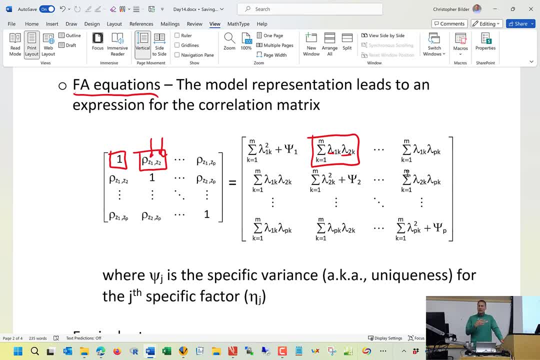 variables. covariance, yeah, covariance matrix for standardized variables. remember that the variance of each standardized variable is 1, okay, so look what we have here. so this is kind of like you could say, the correlation between z1 and z1. of course it's 1 and so notice, you know, comparison to what we. 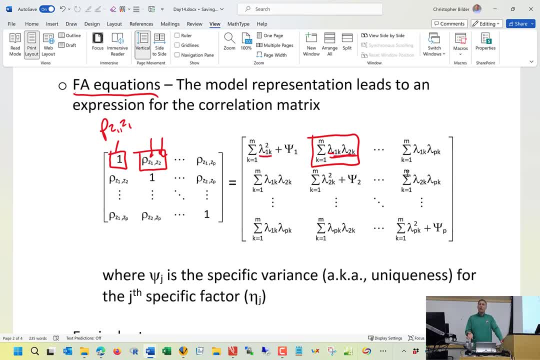 have before. now we have, let's say, a lambda 1 K times a lambda 1 K. that was lambda 1 K squared. but now we also have an additional component, you, which is the variance of a to 1. we again lots of notation, lots of terminology. 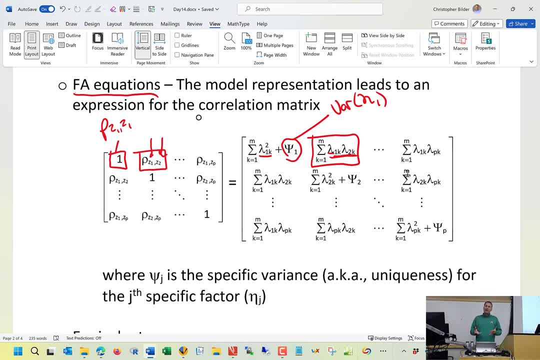 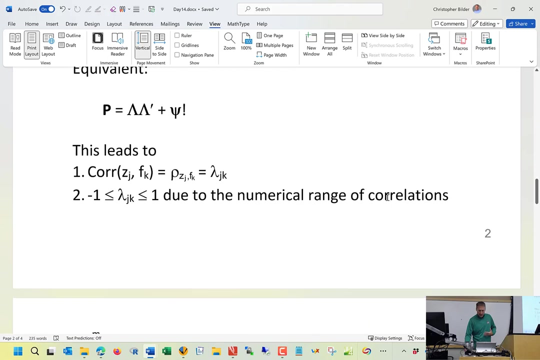 size of 1 represents the variance of a to 1. this is called the specific variance for the specific variable. some people even also call this the uniqueness as well. and secondly, you have this super the we have then, because of our soon model structure, we have this representation for our correlation matrix in terms of 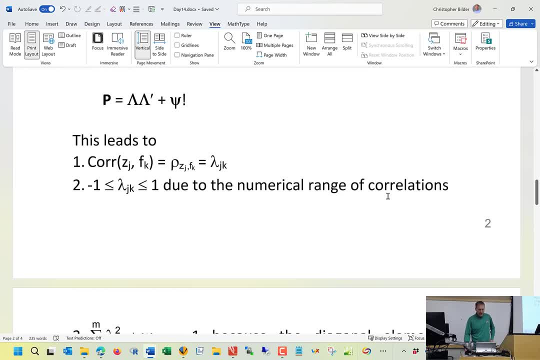 the Lambas in the size, some other, and we'll be using this very, very shortly here. now something else. we looked a little bit at a derivation of a. what's the, what's the correlation between zj and FK? in other words, we'll use these as: 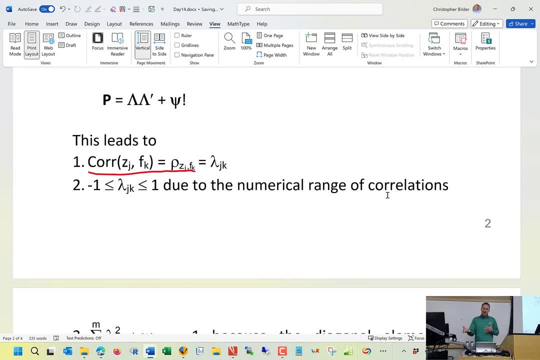 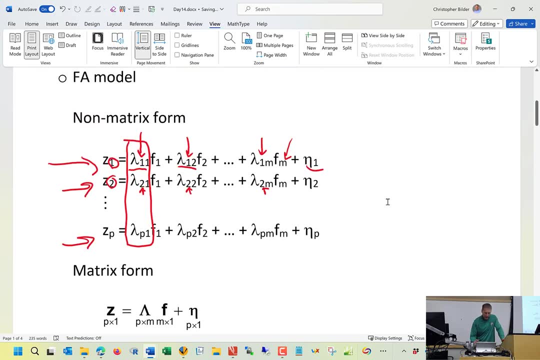 words original variable and one of these common factors. what's that correlation? it ends up being lambda JK. so if we go back to our model, what does that mean for us? we actually do a little bit of erasing again. when we're looking at common factor one, we look at the course by lambda to try to interpret it. but now 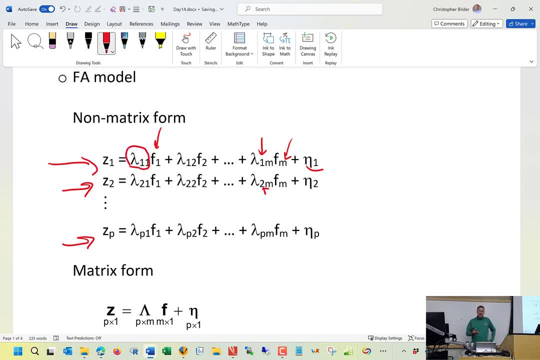 we have another nice way to think about this, that the correlation between F: 1 and Z: 1 is lambda: 1: 1. so again, if a correlation is zero, we know that there is no relationship. correlation is positive. it means that we have a positive dependence. also what this means for us. 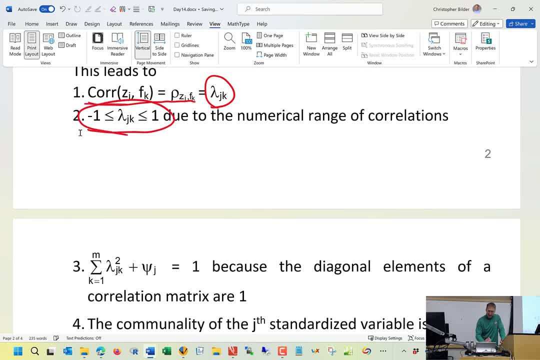 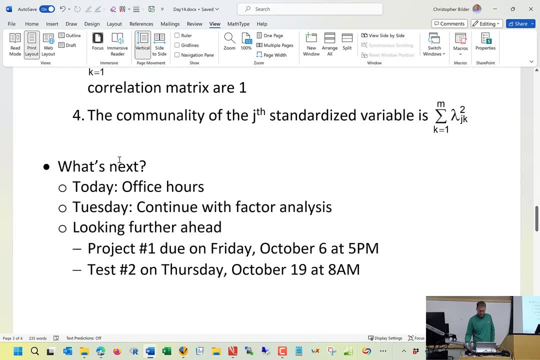 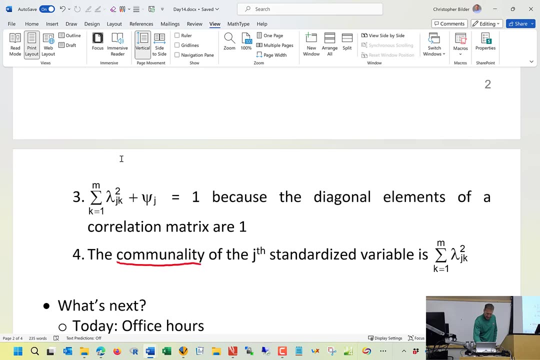 since this is a correlation, each of these landers has to be between negative and positive, one and more. And lastly, just another term. there's something called a communality that we talked about before. The communality of the j-th standardized variable is the sum of the lambda squared. 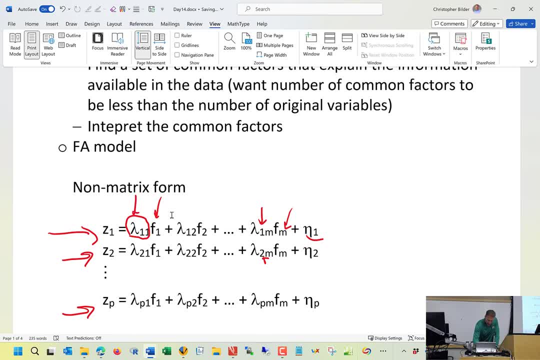 What does that mean? In other words, you take this lambda squared, this lambda squared, this lambda squared and add them up, And so think about that word commonality. What this is essentially measuring is how much information is the common factors explaining? 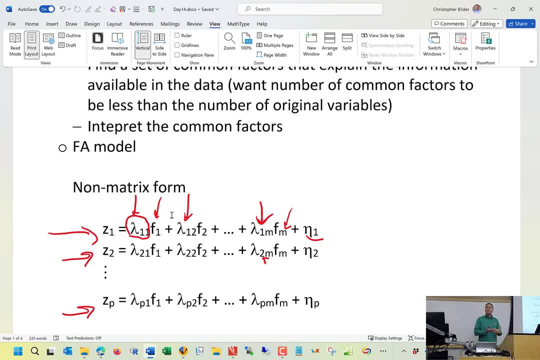 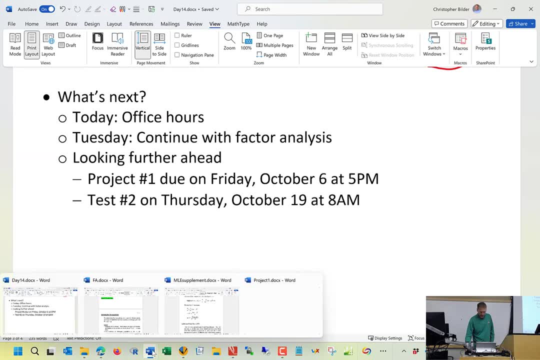 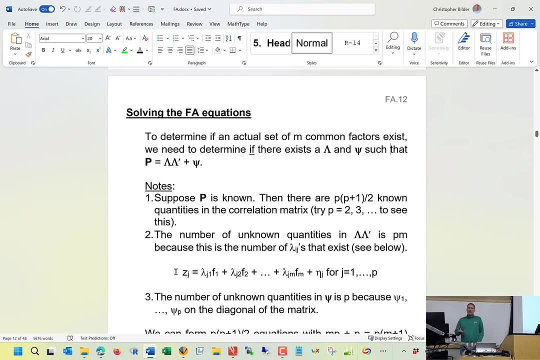 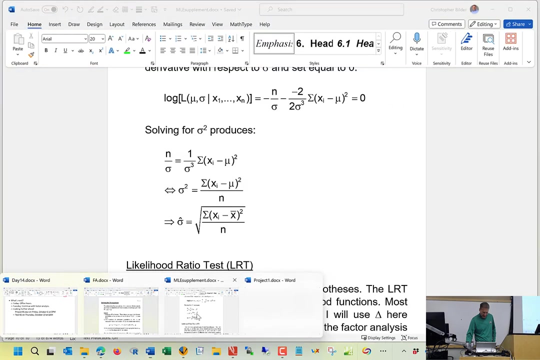 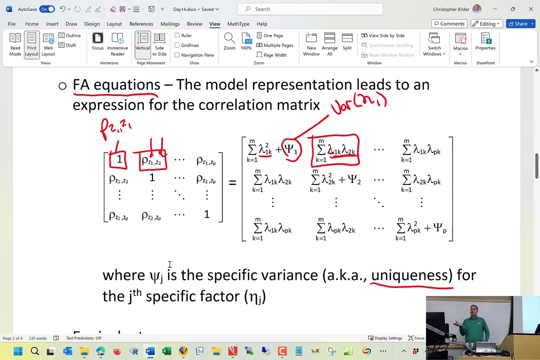 about a particular original variable. Okay, Now let's go on to our new material. We want to be able to eventually estimate these lambdas Because of this relationship that we have with that correlation matrix that tells us that If I happen to know the correlation matrix, I have a way maybe to find out what those 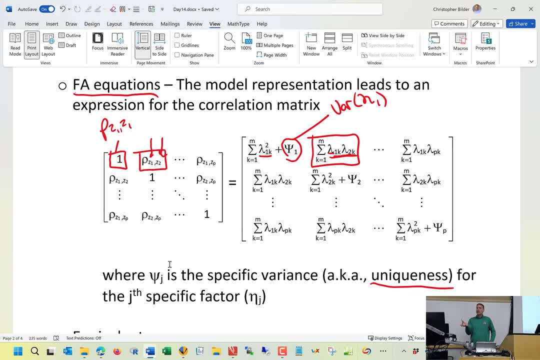 values of the lambdas are what these sides are, As you might be expecting, then is that? well, what if I just replace this correlation matrix with an estimate, And then I can solve for the lambdas, solve for the size, and voila, I have now my parameter. 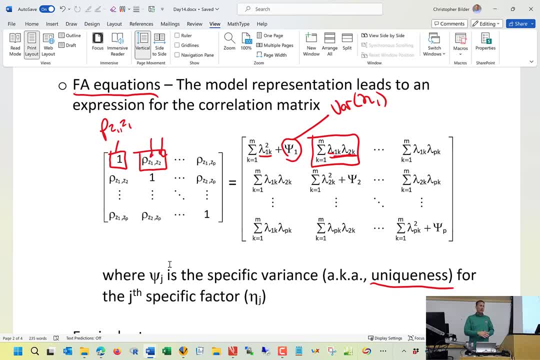 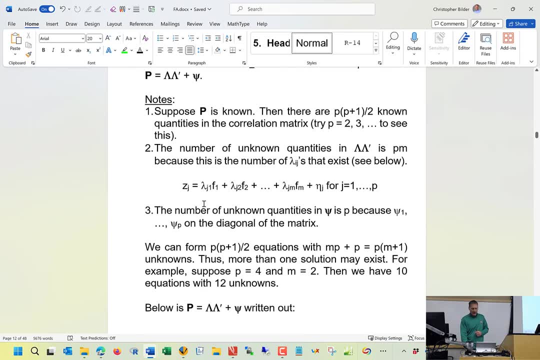 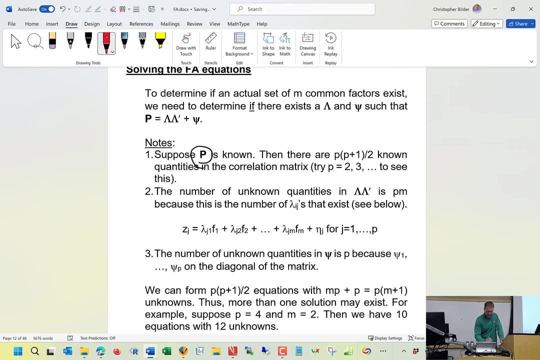 estimates in terms of our model structure. That's essentially what happens, But unfortunately, Unfortunately, things are not as easy as they may appear. Okay, So our correlation matrix. we use the symbol P to always represent our true correlation matrix. Remember, the estimate is represented by capital letter R. 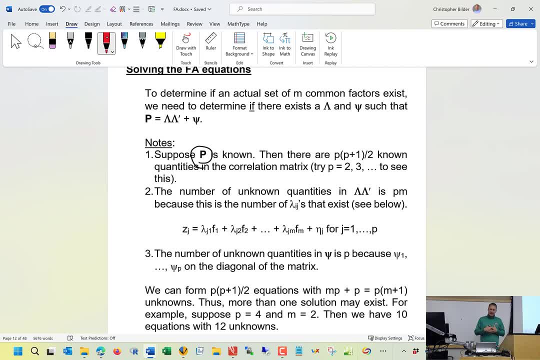 With the correlation matrix. let's say, if it was known, Then essentially we have P times Okay, P times P plus one divided by two quantities known in that matrix. Notice, I'm using a little p there, And that little p is always what we use to represent. how many original variables do we? 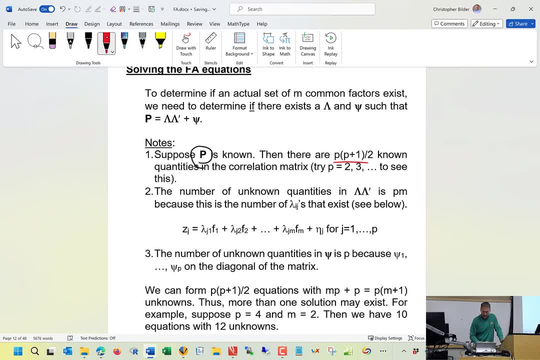 have. Now you might be wondering: well, how does this come about? Well, let's say that P was equal to two. That means we have two times two plus one, divided by three, I'm sorry, divided by two, which is equal to three different known quantities. 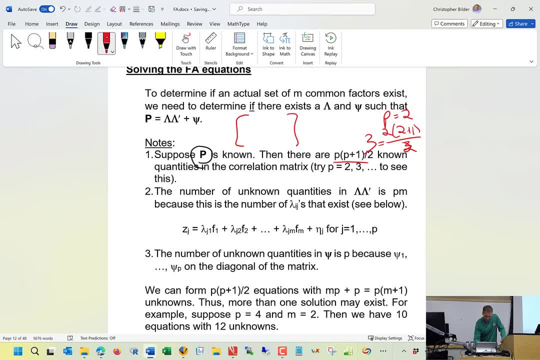 Okay, And if we actually write out that correlation matrix, this is what we have, So I would know this one, I know this and I know that. Notice, the one element of that matrix I didn't highlight is what we had before, because of 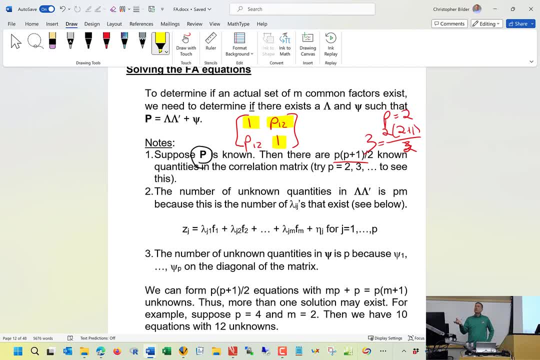 course, I'm sorry, what we have in the one, two element, because the correlation matrix is symmetrical. So that's why we know three quantities, So we have three known, Known values. This right here should be row two, one, But the thing is the matrix is symmetric. 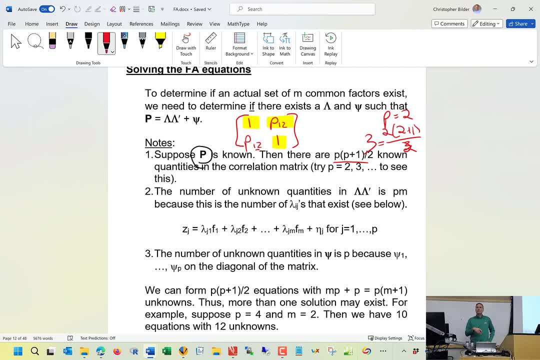 So that's why I can write that as row one two as well. In other words, what's the correlation between z one and z two? Well, it's exactly the same as the correlation between z two and z one, And so that's why I wrote it like that, because the matrix is symmetric. 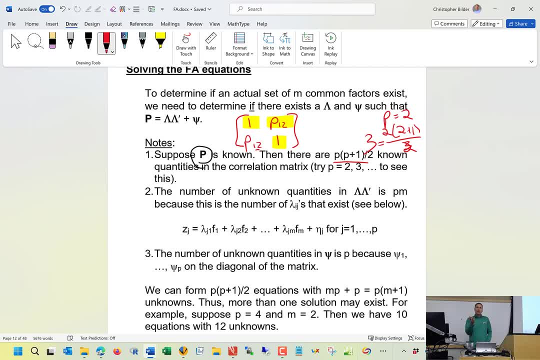 So in the end, we don't know four things, we only know three things, Because these are duplicates. Whatever is in the one two element will be in the two- one element. Okay Now, these lambdas are unknown to us. 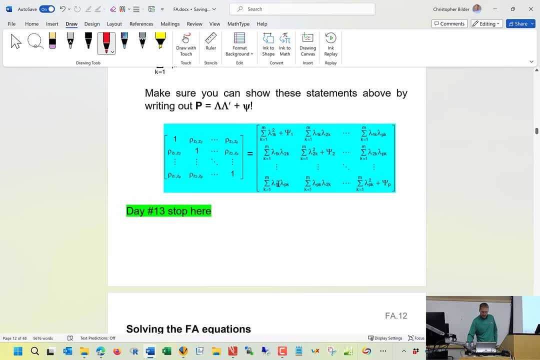 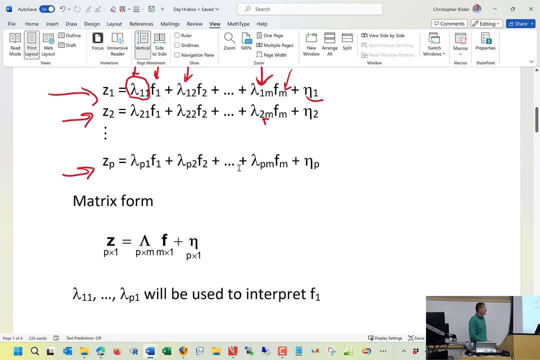 Well, how many lambdas are unknown? Actually, let me go back to what we had here. Go back to our. I think it's easier to see it in this form. here I have p rows or p different equations. I have m- common factors. 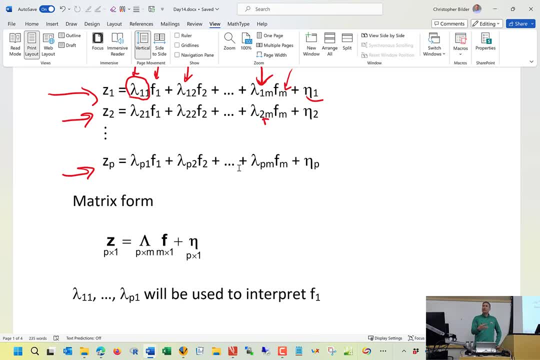 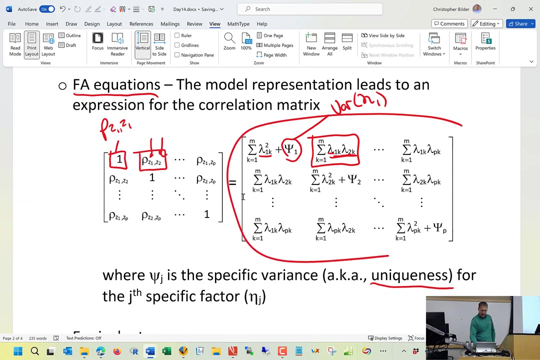 So that means I have p times m different lambdas that I want to get at. Okay, Also remember, with these adas they each have a particular variance that's unknown to us. So we have p variances that are unknown. So in total, on the right-hand side, let's say, of our factor analysis equations, we 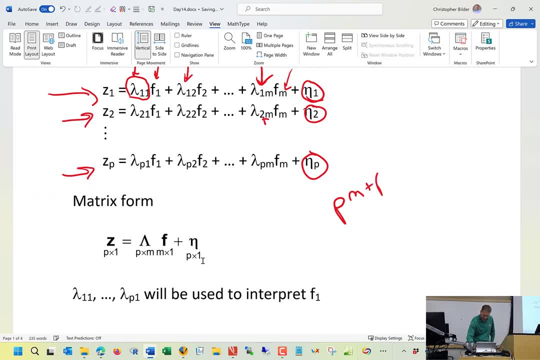 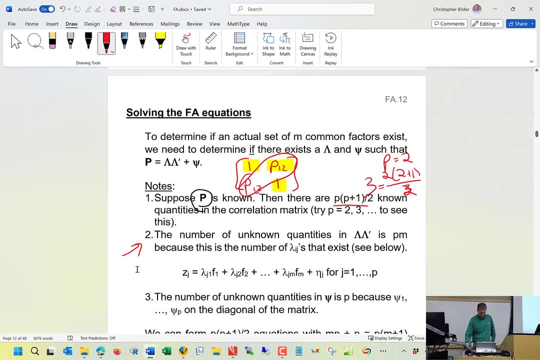 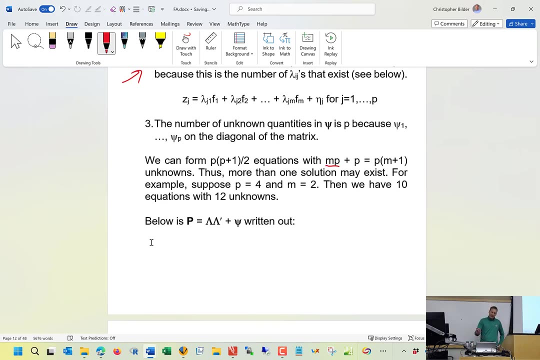 have how many unknowns. P times m plus p. Okay, Okay, For some reason I just wrote it as m times p in a note, but it's p times m as well. So think back to your algebra days, where you had a system of equations. 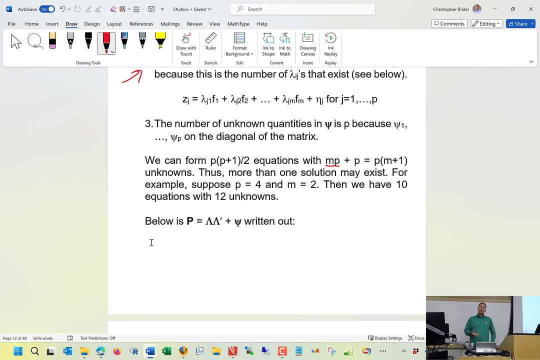 And you had, let's say, maybe you were trying to solve for, let's say, two unknown quantities. You needed to have two separate equations. Three unknown quantities: you needed to have three separate equations. If those numbers don't match up, you can have problems. 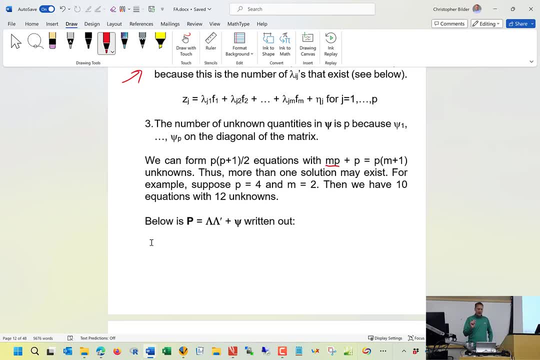 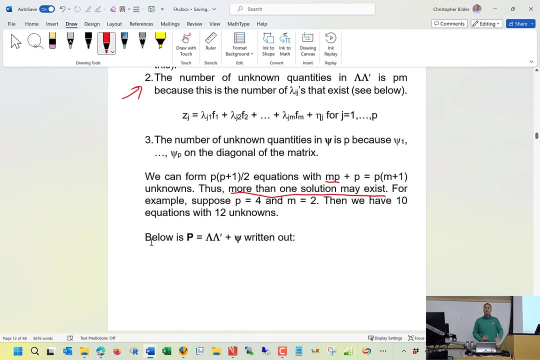 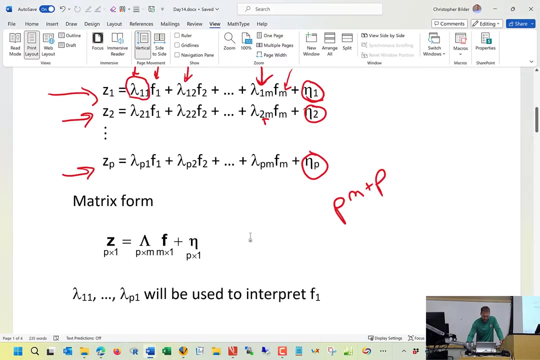 And in fact this is what will happen here. So, for example, more than one solution may exist, meaning that there could be more than one set of lambdas that actually satisfy our system of equations. Now I just want to emphasize something, sorry. 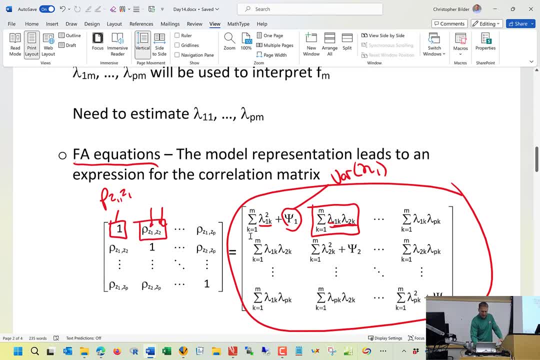 So when I say we are going to have a system of equations, what you could basically say is this: I'm going to set this quantity equal to that. I'm going to set this quantity equal to that. I'm going to set this quantity equal to that. 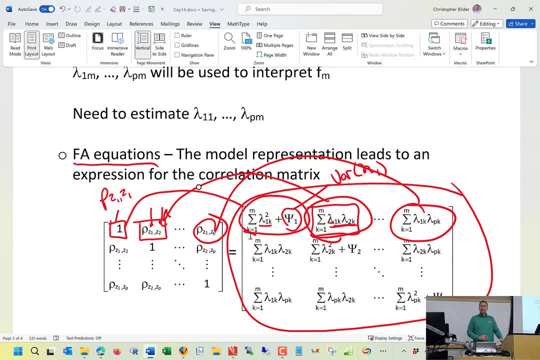 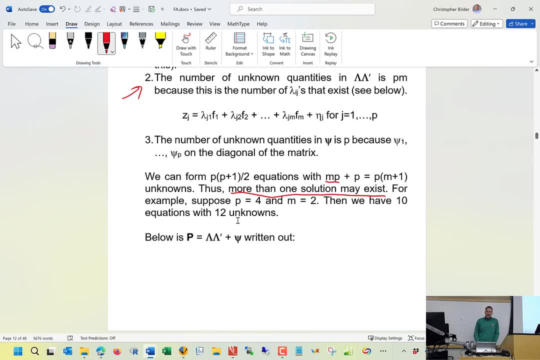 And then solve for the lambdas, solve for the size, Okay, Okay, Okay Okay. For example, let's say that P was four, so we have P. I'm sorry. We have four original variables And we have two common factors in our model. 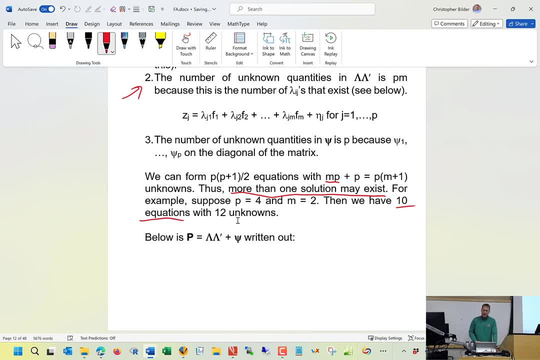 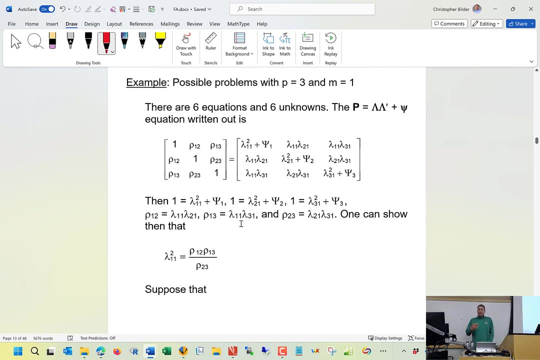 What that means is that we will have ten equations that we can write out, but we have twelve unknown values. So that can be a problem for us. Okay, Okay can be other problems as well. there could be situations where you a solution actually doesn't exist. so previously I just said: well, you can have more than. 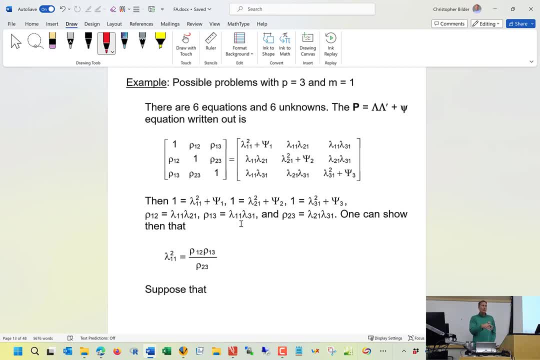 one solution. essentially, you can also have a situation where solution does not exist. so suppose P is equal to 3, M is equal to 1. this corresponds to a situation where you have six equations and six unknowns. hey, that's great. and so here I just wrote it, wrote out the corresponding matrix, and so again, what? 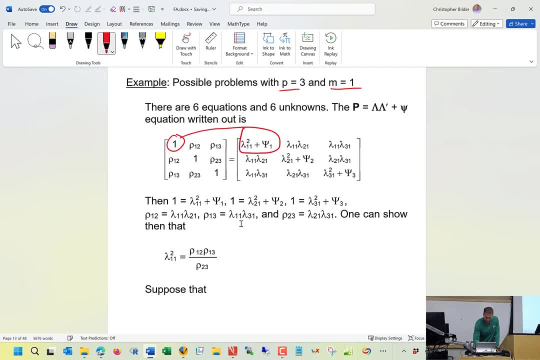 that means is that 1 is equal to this, row 2, 3 is equal to this. I write out six equations, and that's what I actually did here. now, with a little bit of algebra, you can get an expression for lambda: 1, 1 square. how did I do that? 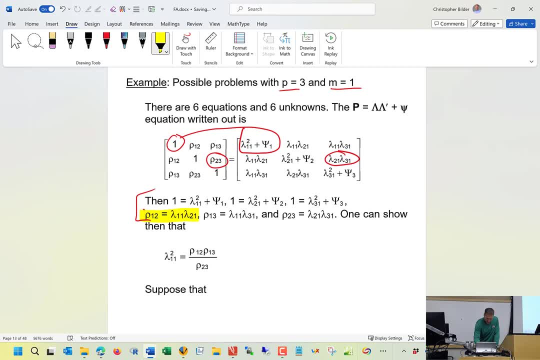 suppose in this, let me highlight, suppose in this equation here solve for lambda 2: 1, in this equation here you solve for lambda 3, 1, then you go ahead and you plug those two values for lambda 2: 1 and lambda 3: 1 into that, into the. 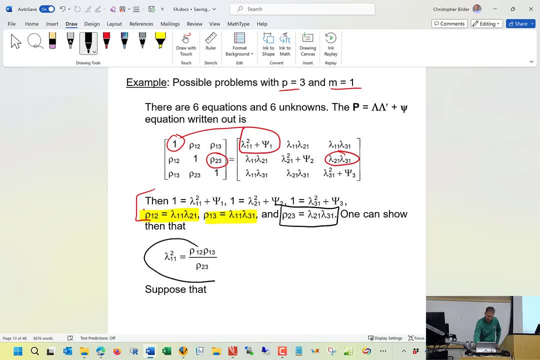 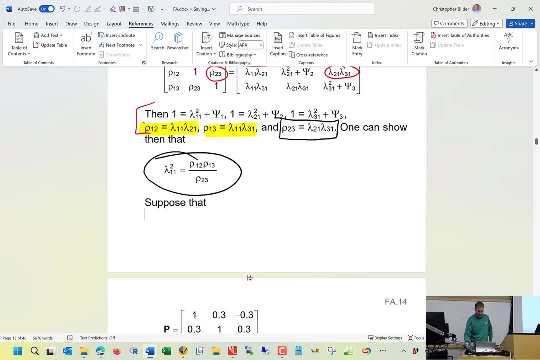 last equation there and you will get this. okay, here's the problem that can occur. so if I put in, you know, you know, row 1, 2 is 0.3, row 1- 3 is negative 0.3. rows of 2: 3 is 0.3. so I get negative 0.3 in the end. for what lambda 1: 1 squared is equal. 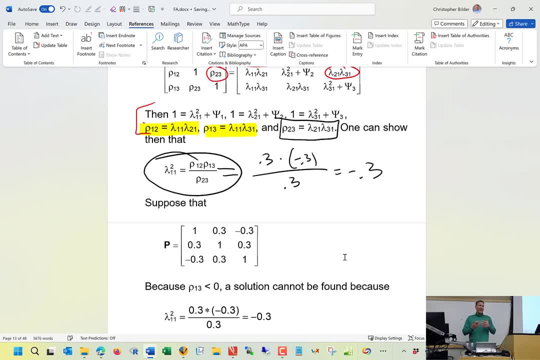 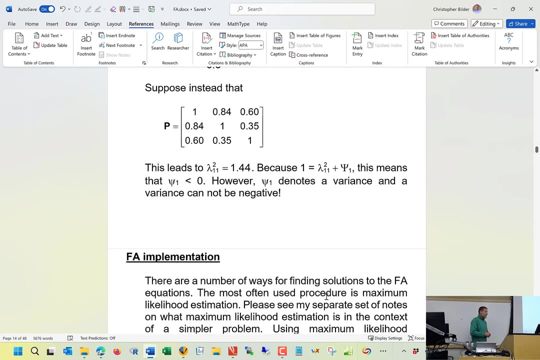 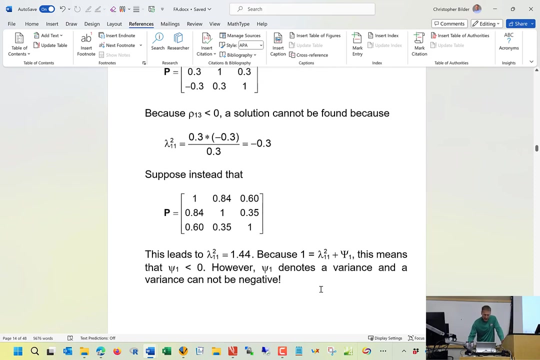 to, but you can't have a squared value be equal to a negative, so a solution does not exist with this correlation matrix. here's another example. suppose that this is my correlation matrix as well. so now I don't have any negative values, and if you go through the same same way of 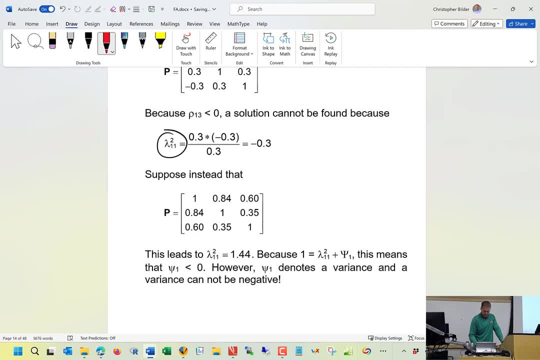 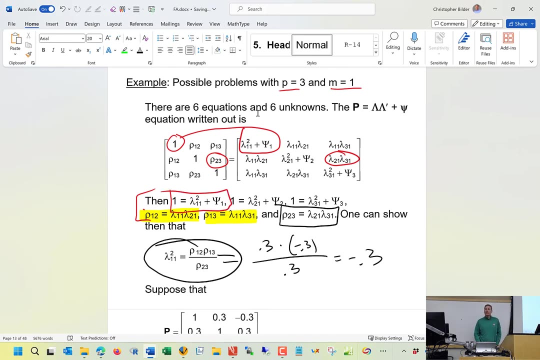 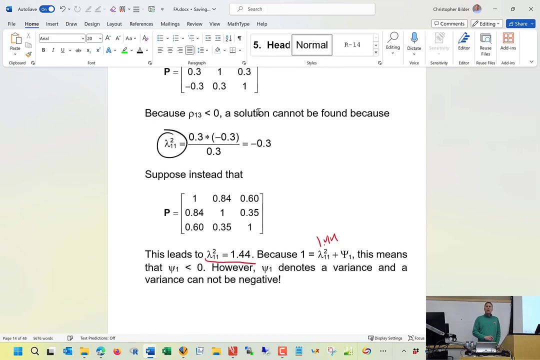 finding what lambda 1- 1 squared is, you get lambda 1- 1 squared to be equal to 1.44. now, remember, we have an equation, though that's up here, that says 1 is equal to Lambda 1, 1 squared plus psi 1, so what you could do is simply put in that one point four one there. 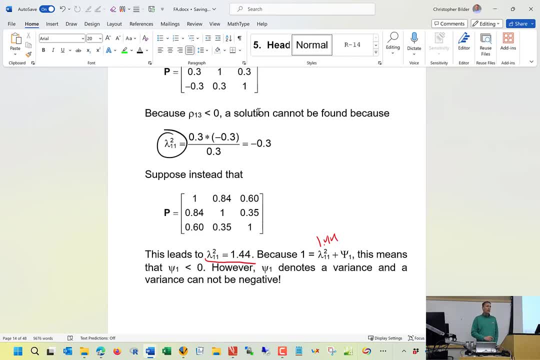 psi1, then would have to be negative. point 4: 4. but psi1 is a being you can't use a hearings in random situations. it's not like measures are zero information, it's just an expression, if you have any. So now we have another problem here. 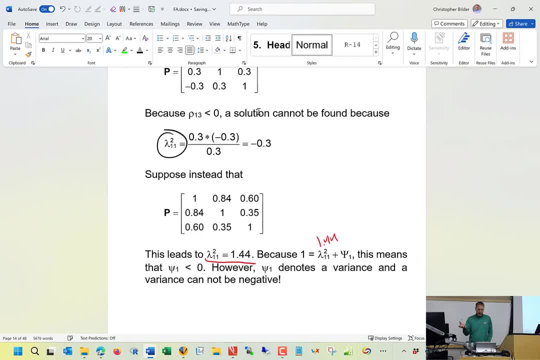 So once we get into actually formally doing the estimation, you will sometimes have R tell you: uh-oh, a solution doesn't exist, And it could be for the reasons that I just told you here. So we have to be on the lookout for that. 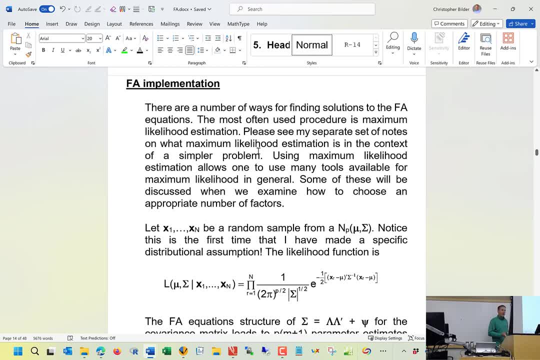 So now we're getting into. now. how do we find these parameter estimates formally? There's a few different ways. I'm only going to talk about the most prominently used way, which is what's called maximum likelihood estimation. Now, maximum likelihood estimation. 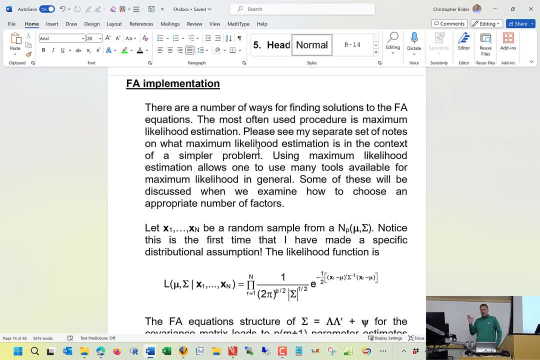 is something that is widely, widely used in statistics, But I also understand that students, when they come into this class, they may not have seen this before, So I'm going to go to a separate set of notes, which are called my MLE Supplement. that was on my website. 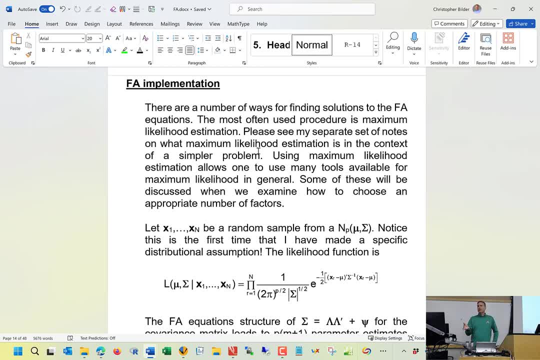 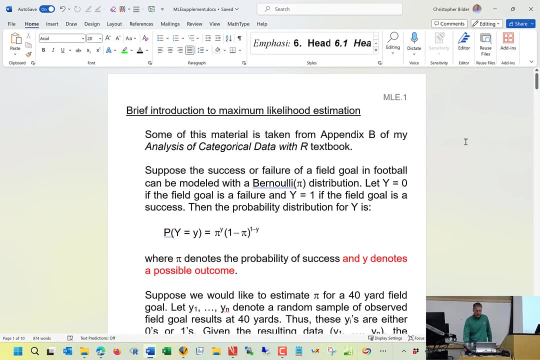 that briefly explains what maximum likelihood estimation is, so that we can apply to this particular problem. So So the way that I like to explain it. if I'm not doing this, like to explain maximum likelihood estimation. well, let me back up a second. 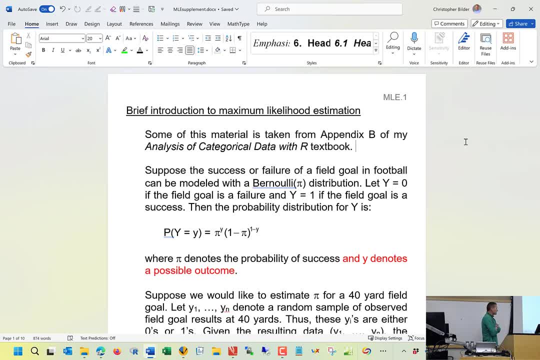 if you, if you want a little bit longer explanation, you can take a look at appendix B of textbook that I wrote for our categorical data analysis course that we- that I- primarily teach here at this at the University. I also talk about maximum likelihood estimation. then, whenever I do a mathematical in terms of 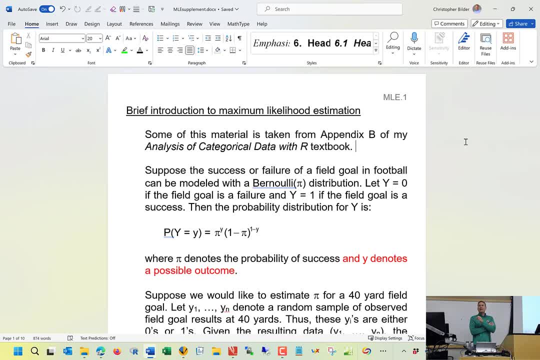 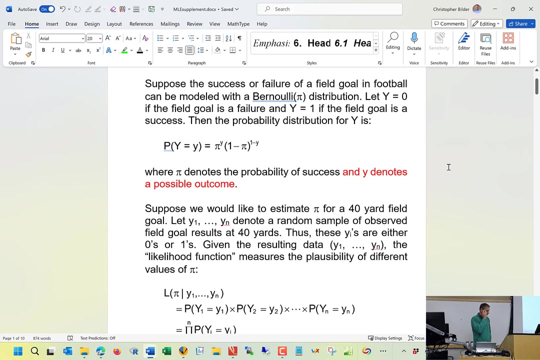 I also talked about maximum likelihood estimation in terms of an introduction whenever I do a mathematical statistics course. so if you look at my step 880 notes, you will see another explanation there as well, and the way that I often like to introduce maximum likelihood estimation due to students is through. 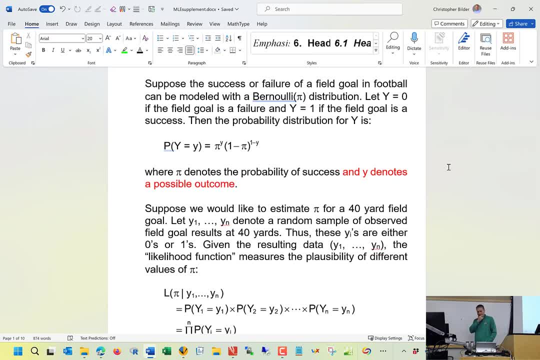 kind of an intuitive example, and this deals with the- the success or failure of a field goal. Now, in your very first stat course, you'll learn about the probability distribution, called the Bernoulli probability distribution. that's used in situations where you essentially have two possible outcomes for your random variable. 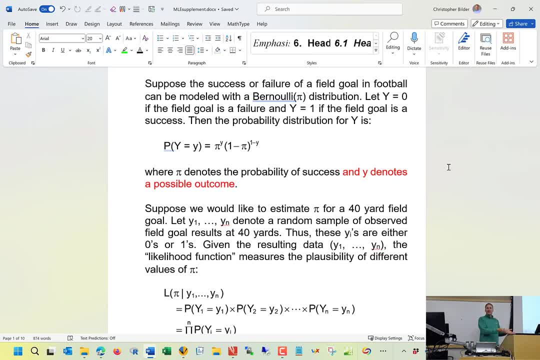 which we often say is a success or failure. A success for a field goal, failure for a field goal. This is one way to write out this probability distribution, which should at least have some similarities to what you've seen before. Let's say, my random variable. 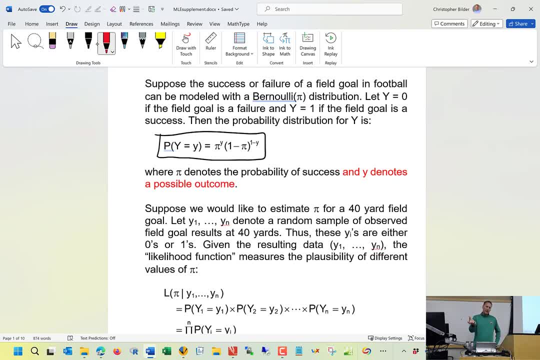 y represents the success or failure of a field goal. For y equals zero. for a failure, y equals one for a success. I'm going to be a little bit more formal in my presentation here, where I use uppercase letters to represent random variables, lowercase letters to represent: 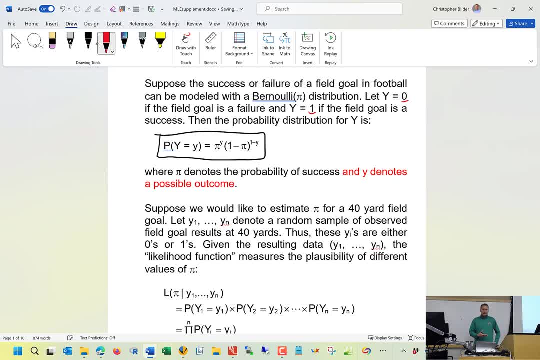 values that they can take on. If you have seen that before or if you're not comfortable with it, here's simply a really brief explanation. So my random variable would be zero or one, And sometimes I want a symbol to say, well, it's zero or one. 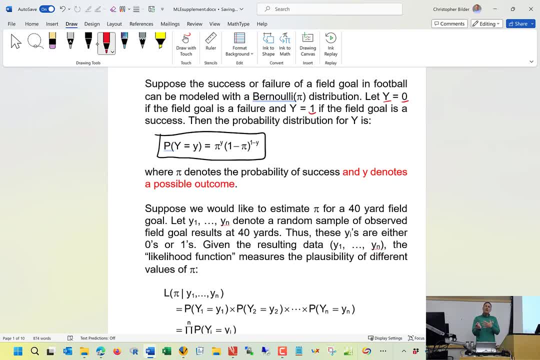 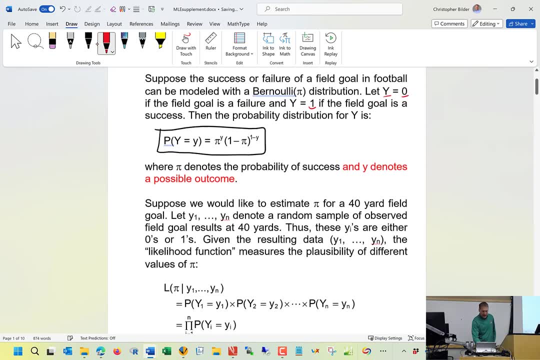 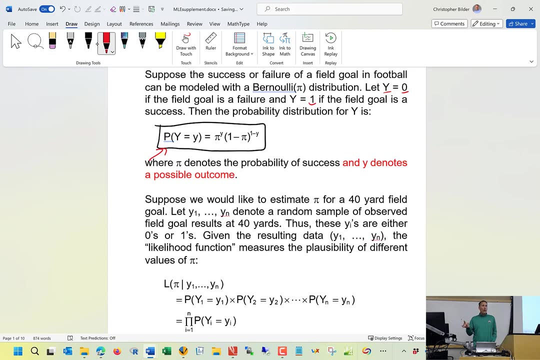 but I don't want to necessarily always write out zero or one in there, And so in those particular situations we use the lowercase letter y to represent that. So here's my probability distribution: the probability that my random variable y is equal to either zero or one. 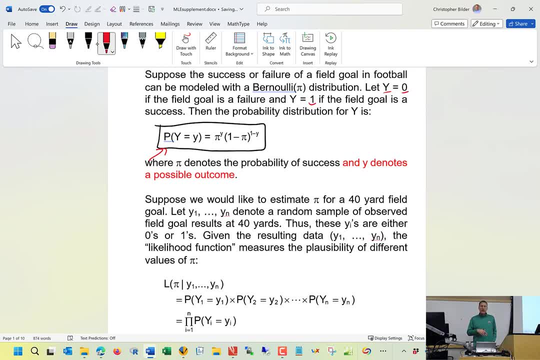 which I denote as simply little y or lowercase y, is equal to, let's say, the probability of success for a field goal is pi, the Greek letter pi, And we have pi raised to the y power times one minus pi raised to the one minus y power. So if I simply write this out, 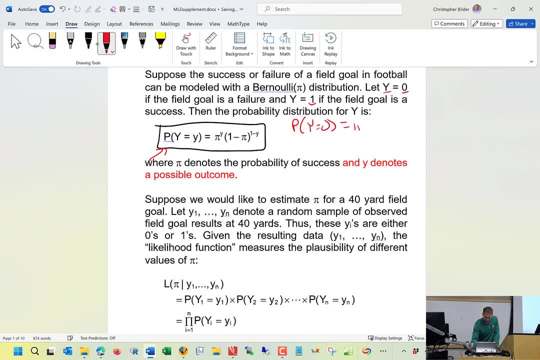 it's the probability y is equal to zero. This would be pi raised to the zero times one minus pi raised to the one minus zero, or in other words, one minus pi. Probability y is equal to one is equal to pi raised to the one. 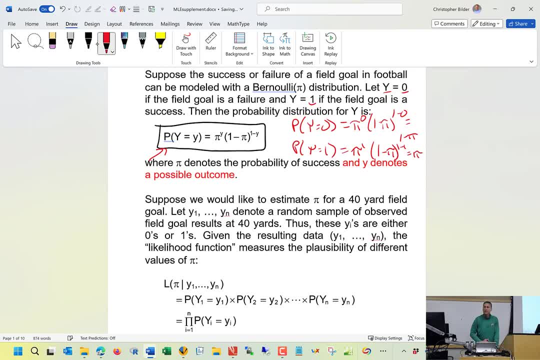 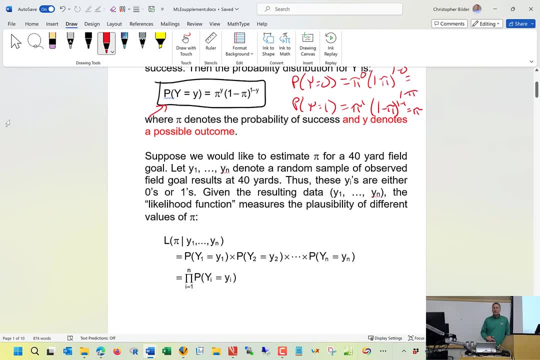 one minus pi, raised to the one minus one or just pi. And let's say that you know I go out to Memorial Stadium and I decide to: you know, try to estimate my probability success for 40-yard field goals. And so what do I do? 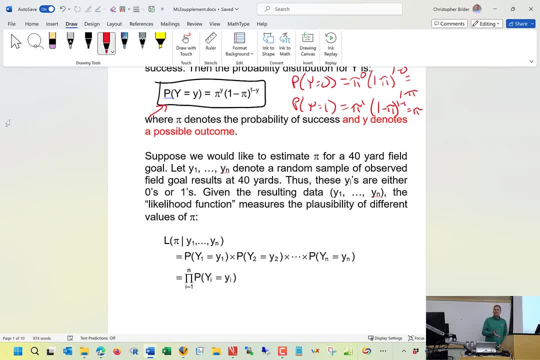 I take a sample of me kicking the ball. you know, in general, in a general way, let's take a sample size of n, or eventually we'll say how about we just do it 10 times? you know, Perhaps I was well. did anybody go to the game on last Saturday? 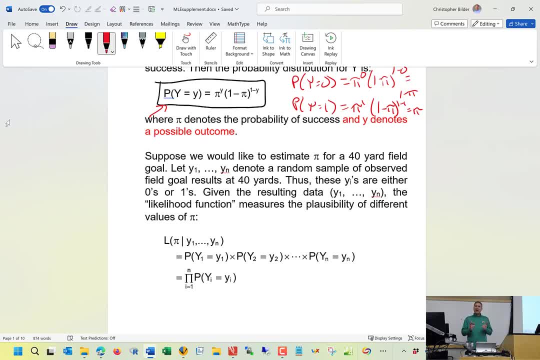 You didn't miss much. The best part of the game was actually- I think it was in the first quarter, when the teams were. there was like a TV timeout, So the teams are off the field And so always in the first quarter they have this contest where, let's say, a randomly chosen fan comes down on the field and they try a field goal And if they make it they win $5,000.. And the guy made it. That was like the best part of the game. 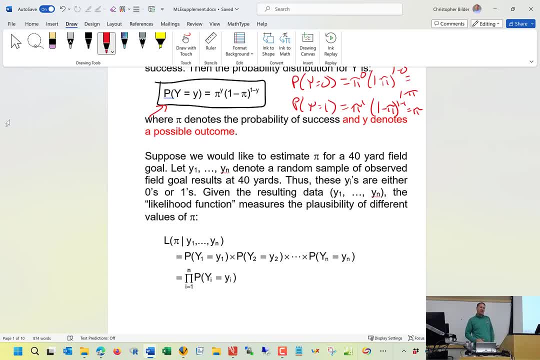 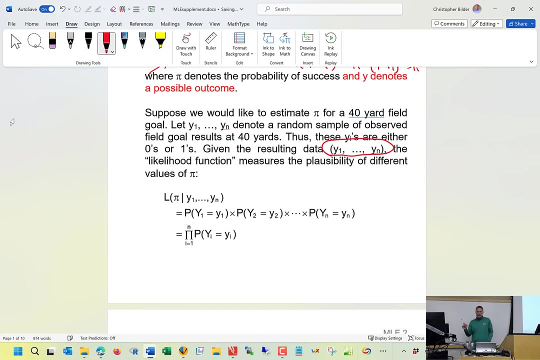 And so I don't know, maybe he was using statistics to try to figure out how best to kick that field goal And so anyway. so Y1 through YN, where I'm using lowercase letters there, represent, let's say, a general way to represent my actual sample that I got. 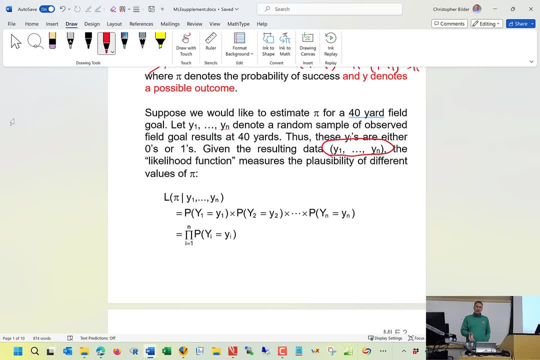 You know, maybe you know, the first kick was a failure, so I have a zero, So that would be like little Y1.. Second kick was a success. little Y1,, I'm sorry, little Y2 would be one. 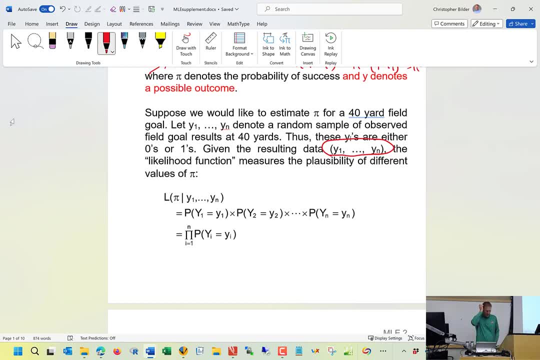 And so, given this information, I like to estimate my probability of success, And a formal way to do this in statistics is to start with what's called a likelihood function. And all that a likelihood function does: it measures the plausibility of different values of pi. 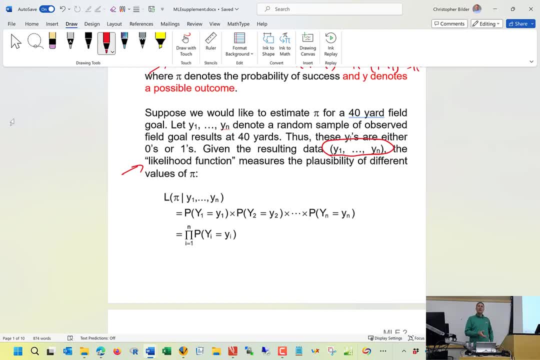 So is pi equal 0.1 a plausible value for, I'm sorry, is 0.1 a plausible value for pi? Is 0.6 a plausible value for pi? And it's formed in a rather intuitive manner here. So, first of all, in terms of notation, the likelihood function is a regular mathematical function. 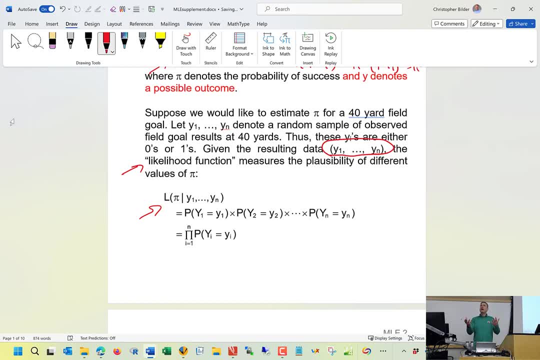 We call this likelihood function L, L of pi. it's a function of pi. We use the vertical line here to represent the word given L of pi, given my data, given my information, that I observe And all that I observe is a function of pi. 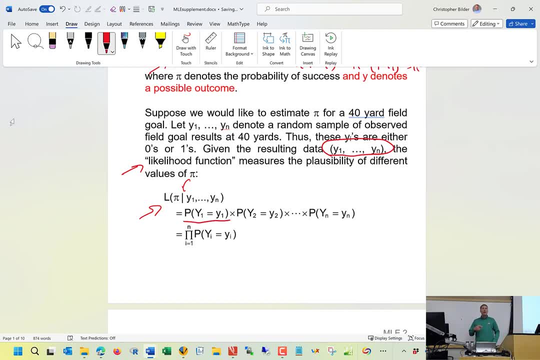 And all that I observe is a function of pi, And all that I observe is a function of pi And all that it is. is this: The probability for my first field goal that I attempted: the probability that's either a success or the probability that it's a success. 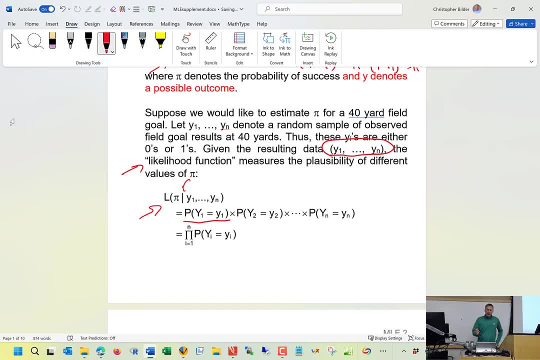 I'm not saying that very well. The probability that Y1, capital Y1,, which represents what happens on my first field goal, is equal to either 0 or 1.. Times: same thing for the second field goal. times all the way up to the nth field goal. 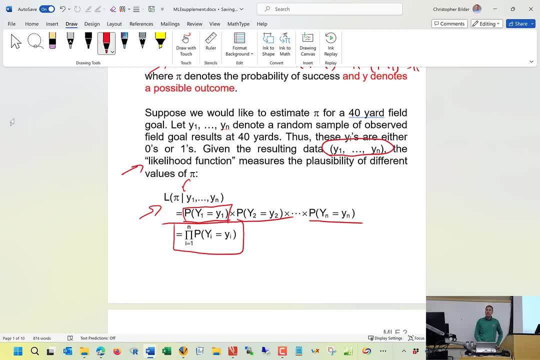 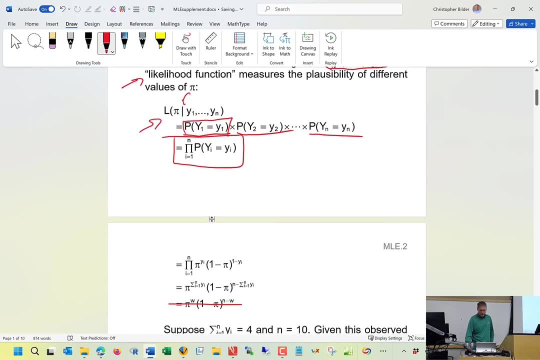 And so I could write this more compactly in product notation, where I take the product from: i equal 1 to n of the probability that capital Y sub i is equal to little y sub i. Then we can plug in our Bernoulli probability distribution there. 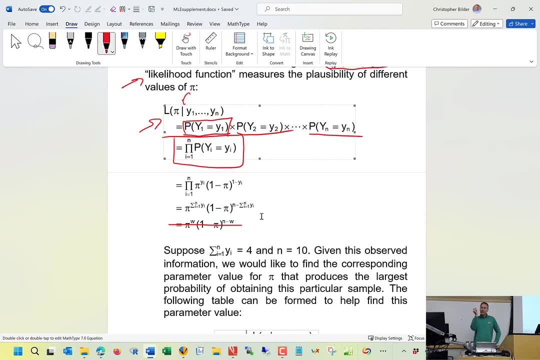 So the distribution that we had before. the only difference is now I say okay, this is for y sub i instead of just y in general. Then I can use properties of working with exponents. So just to make sure you see this. 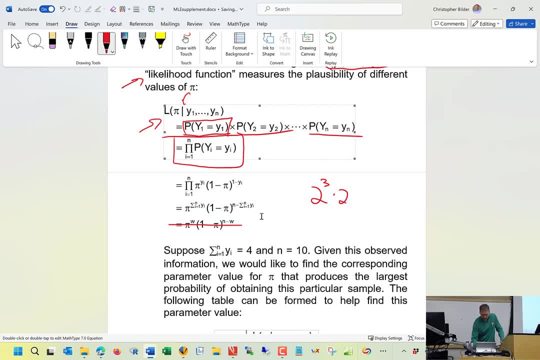 So if I had, let's say, 2 to the third power times 2 to the seventh power, that would be 2 to the tenth power. I just add the stuff that's in the exponent. So that's why I have the sum of the y's and n minus the sum of the y's there. 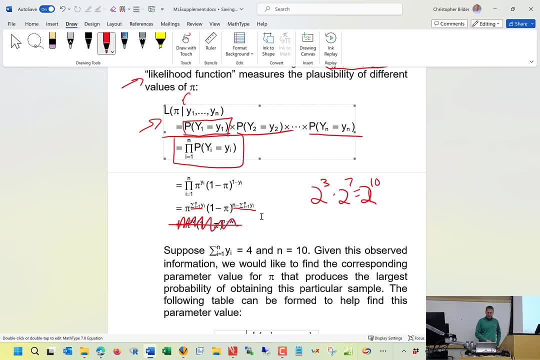 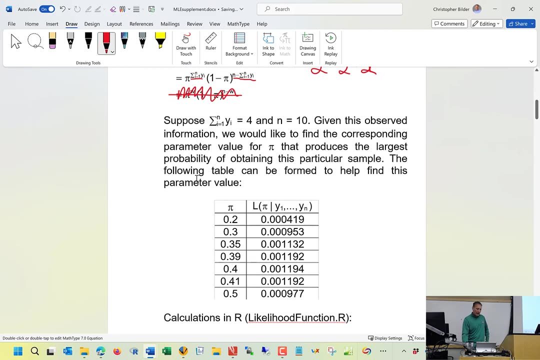 And you can just delete that very last line of that equation. And so let's say that I actually observed four total successes out of ten different times that I kicked the field goal, And then what I could do now is use this data, use this information. 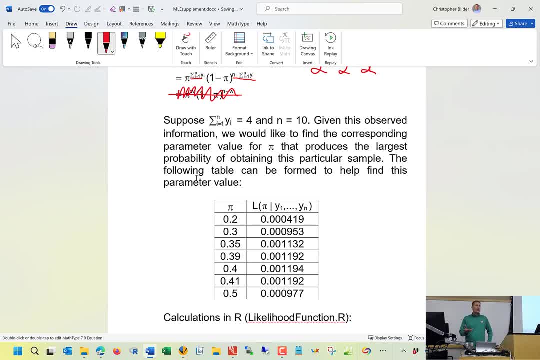 to evaluate what my likelihood function would be at particular values of pi. Again, we are using this function to evaluate the plausibility of different values of pi. The larger this function is in numerical value, the more plausible the corresponding pi will be. 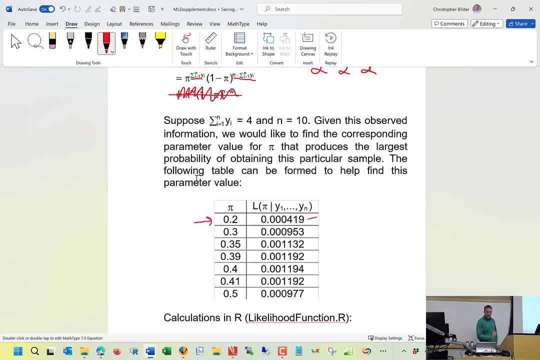 And so I could put pi equal 0.2 there, and I get 0.000419.. I could put 0.35 in there, I get 0.001132.. So in terms of this likelihood function, 0.35 is more plausible than 0.2.. 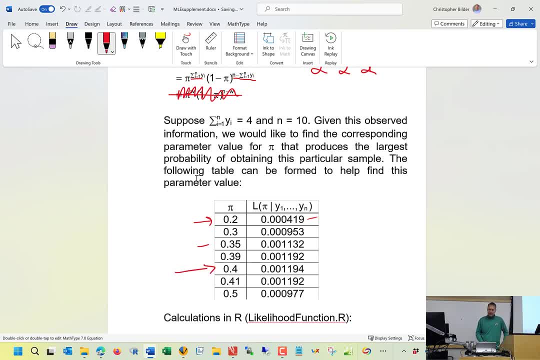 And eventually you can get to a point where you see that 0.4 has the largest possible value of the likelihood function And therefore we would say that this is the most plausible value of my value, the most plausible value for pi, And so what we have just found here is what's called a. 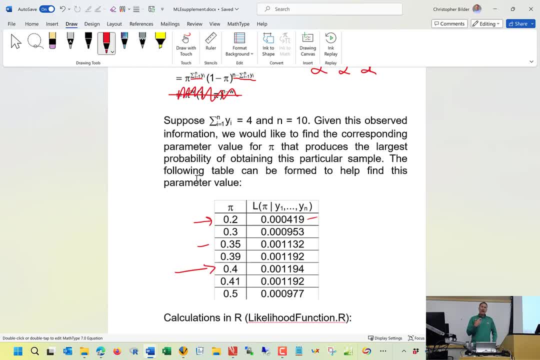 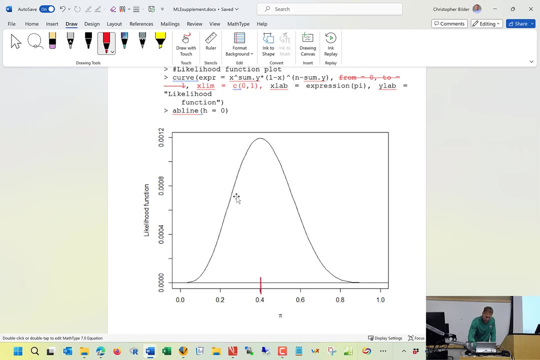 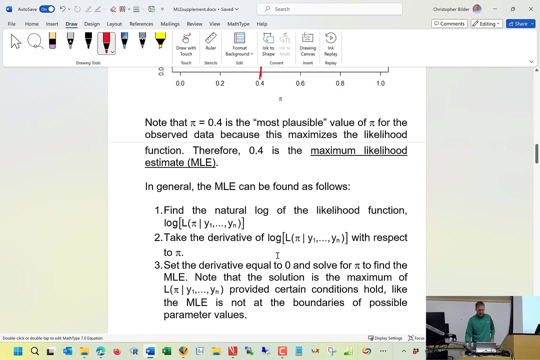 maximum likelihood estimate And pi equal 0.4 maximizes my likelihood function. One could actually plot it out And you can see that at pi equal 0.4, indeed that's where my maximum is reached. I'm sorry, could you repeat that please? 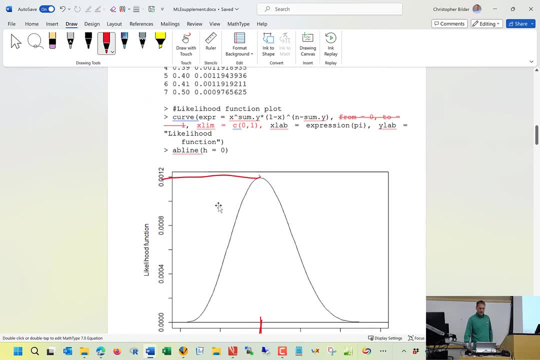 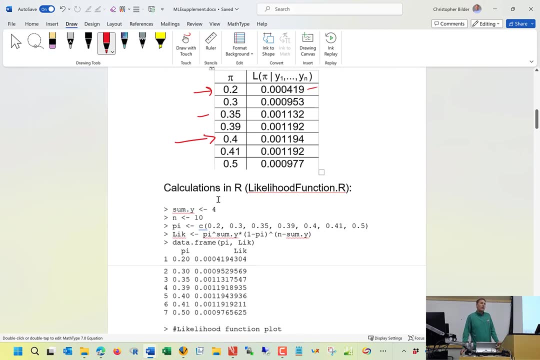 Say that one more time, please. This table: You calculate the values with r In the end. well, you in the end. I did yes, Yeah, not with your hand, And we don't have to do this with our hands. 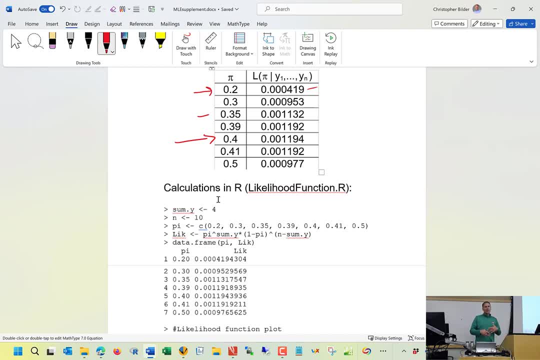 No, So I skipped over the r part here because I feel as though that's not as important. I mean, anybody could do it on a calculator too, And this is more background information so that we can apply it with respect to factor analysis. 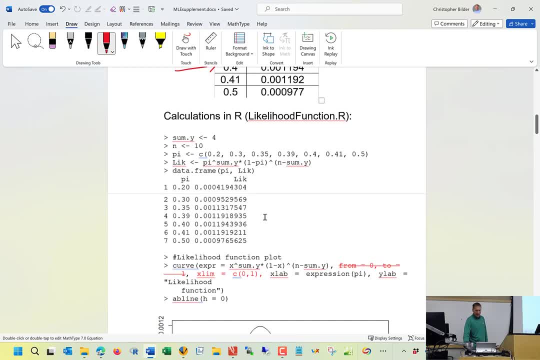 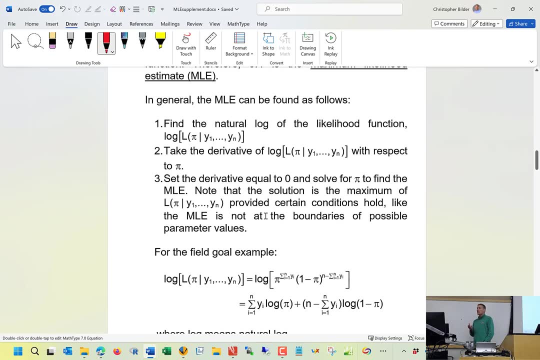 But I didn't want to hide anything. That's why I also included the coarse-bind code. Okay, So that's my maximum likelihood estimate, My most plausible value for pi, given my data. Hopefully that's intuitive If I have four successes out of ten trials. my proportion of successes is 0.4.. 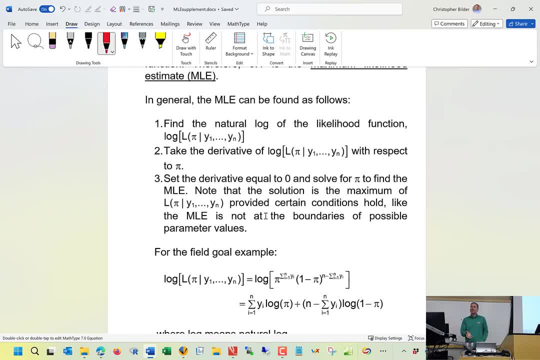 Okay, That makes sense. That's why I choose this example, because it makes intuitive sense. Now, in general, though, the maximum likelihood estimate can be found using tools that you learn about in your, let's say, Calculus 2 or Calculus 3 course days. 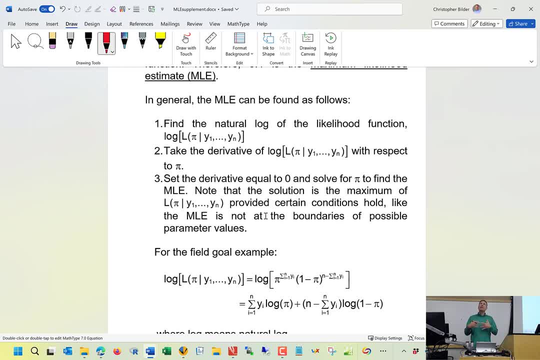 When you talk about how do I maximize or how do I find the value of some function that maximizes it or minimizes it, And so what we could do is as follows: First, we begin by finding the natural log of the likelihood function. 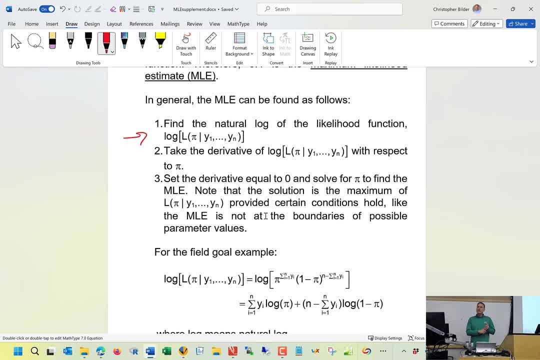 Well, this isn't needed. This is the way that most people will approach it, because then you can come up with a nice mathematical form for the resulting function, as you will see shortly when we apply it to this Bernoulli example. Take the derivative of this log likelihood function with respect to pi. 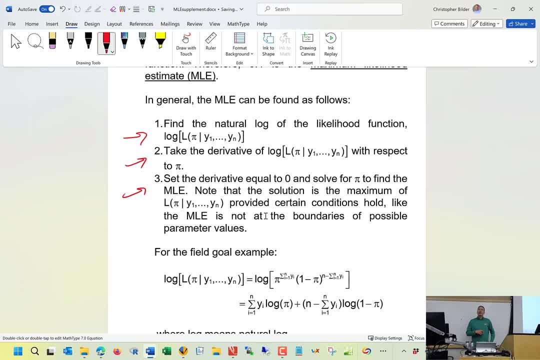 Set the derivative equal to 0.. Solve for pi And along certain regularity conditions that occur, this will be the maximum likelihood estimate One. we should find the log. I mean we usually get that derivative and set it equal to 0.. 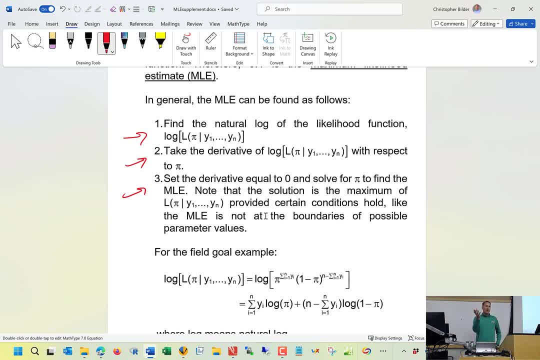 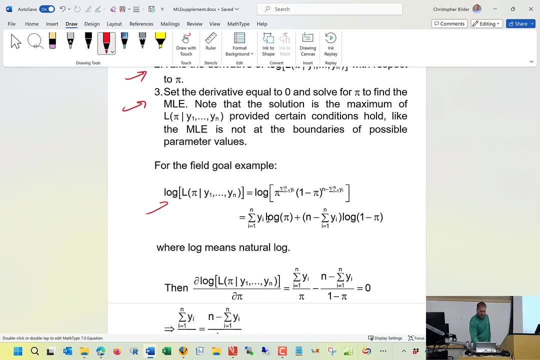 Yeah. So, first of all, using the log is not going to change anything because it's a monotone function, The reason, and I'll just jump ahead. So let's say, if I actually wrote out now the log likelihood function, I should say sorry I didn't say this before. 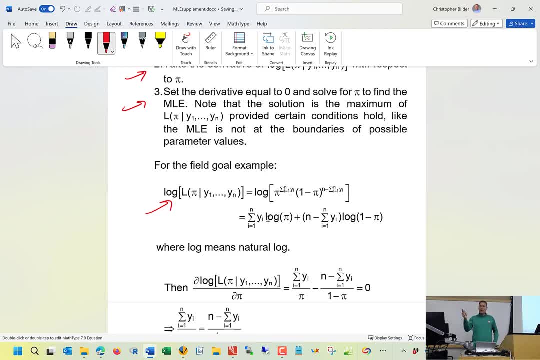 In statistics, typically whenever someone used log, they mean natural log. Okay, So if I take the natural log of the likelihood function there, notice what happens. So if I had, let's say, the log that we'll just talk about in general first. 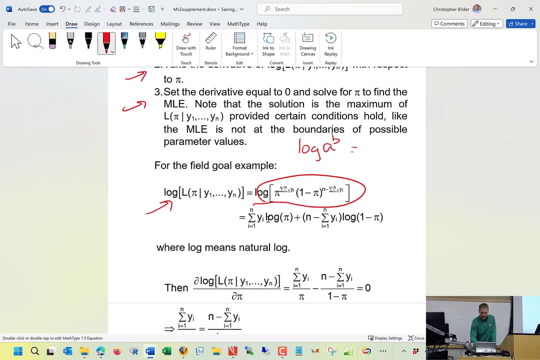 The log of a raised to the b power, This is equivalent to b times the log of a, And so look what happens for us then, And also sorry. there's one more thing I should mention If I had log of a times b using properties of logarithms. 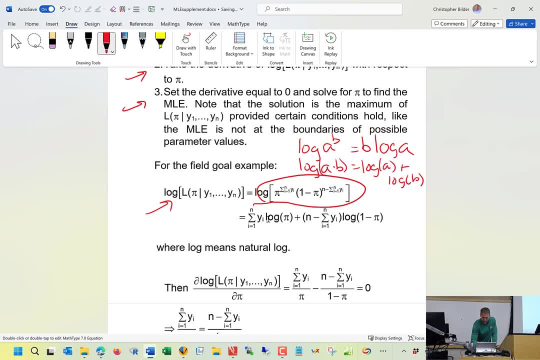 This would be the log of a plus the log of b. So now look what happens with this expression here When I take the log of pi raised to the sum of the y's Times 1 minus pi raised to the n minus sum of the y's. 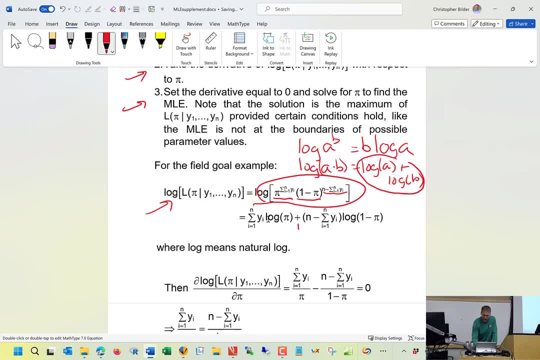 I can first break it up into two different components, so that I have a plus there now, And then, since this is up in my exponent, I can bring that out In front of the log, And so that's why we end up using the log. 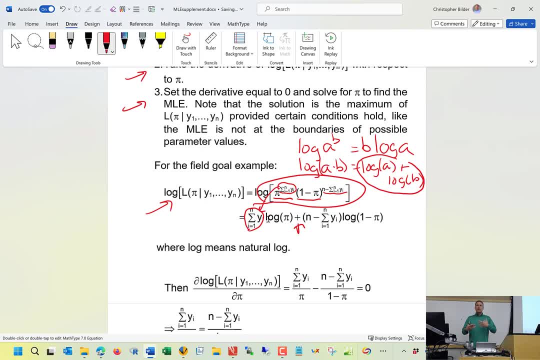 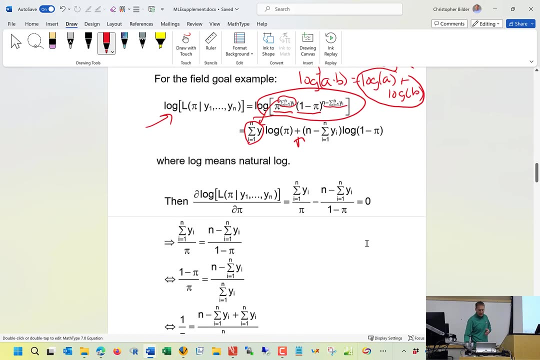 Very many probability distributions have something, let's say, up in the power, And so that's why working with the log is the standard. It can also have some numerical advantages as well. So if I I wrote it in terms of partial derivative. 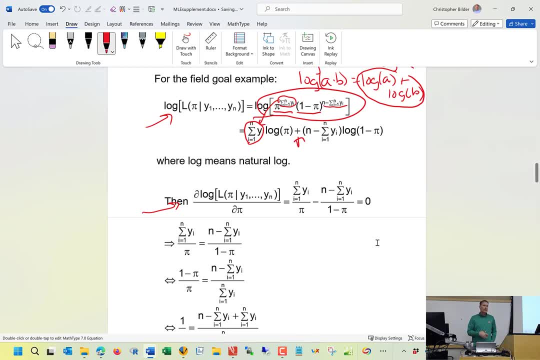 If I take the derivative With respect to pi. So, for example, remember, the derivative of log of pi would be 1 over pi. The derivative of log of 1 minus pi would be negative: 1 over 1 minus pi. Using that chain rule, 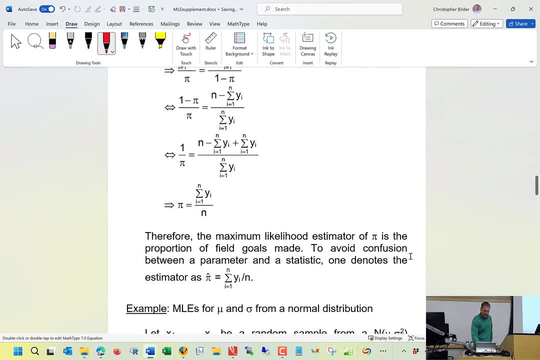 I set this equal to 0.. Do a little bit of algebra And here's my maximum likelihood estimator: The sum of the y's over n, Which is essentially what we had before, When we had 4 successes, 10 trials. 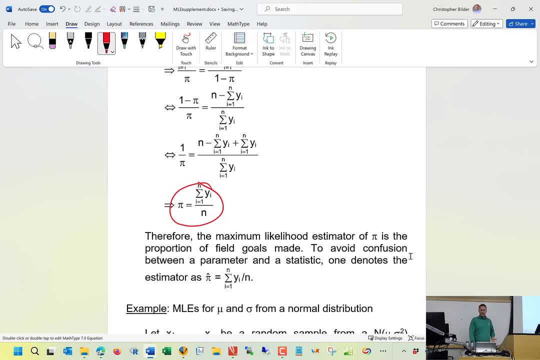 This is just a more general representation, Since this is an estimator. To allow us to calculate an estimate We always put, We always make some kind of symbolic change. Typically we put a half on top of the corresponding parameter that we're trying to estimate. 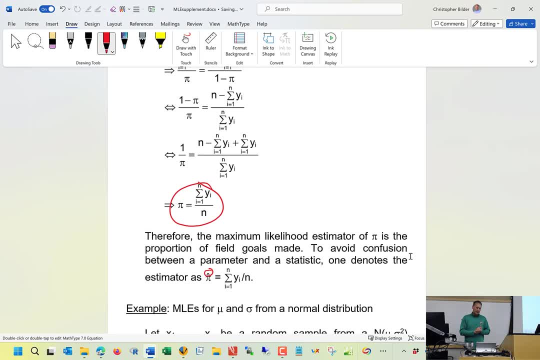 To say, hey, this is my estimate, Rather than a true value. Okay, So that's a very basic explanation of what maximum likelihood estimation is. We will never need to do anything like this by hand, But it's good to have an intuitive feel for how this comes about. 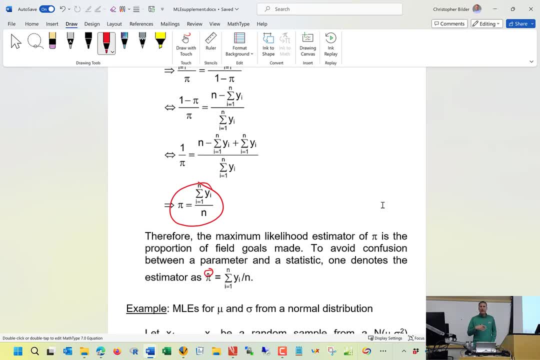 R will actually have a function for us with respect to factor analysis That will automatically find the estimates for us, If they exist. Later in the semester there will be two sets of notes Where we have to use maximum likelihood estimation again And again. R will have functions available to us. 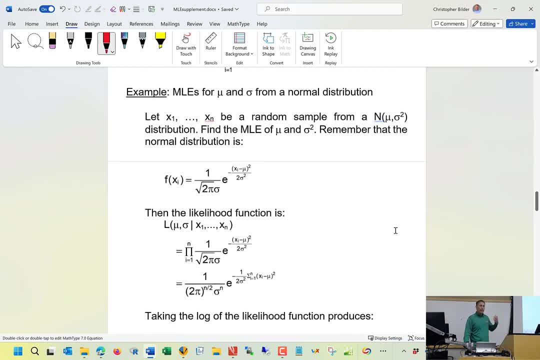 That automatically does the calculations. If, by chance, you were interested in seeing a little bit of a more complicated example To find a maximum likelihood estimate Using working with derivatives and stuff, Here's how you can do it with a normal distribution Where you're trying to find the estimates for mu. 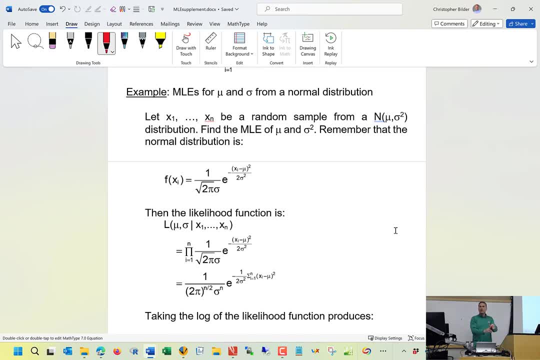 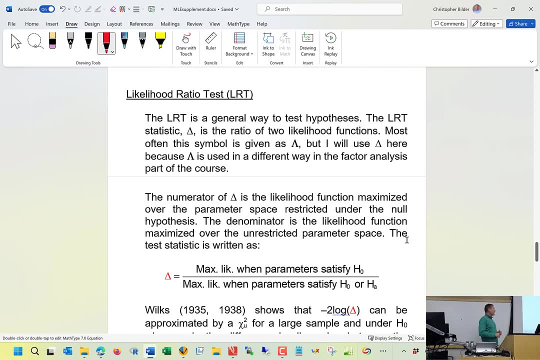 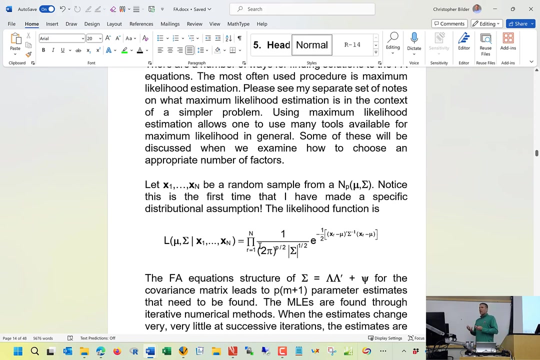 That mean Sigma, the standard deviation. Also in these seven notes I have a little bit of a subsection on likelihood ratio tests. We will come back to that, But for now Let me go back to the main part of the notes. So in our particular case the likelihood function is much more complicated. 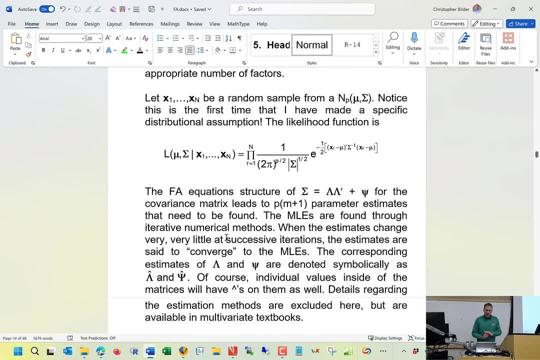 Than what we just saw with the Bernoulli distribution. You know, for our case We have a random sample That results in vectors. For each observation, We have X1 through Xn And Previously, when I introduced factor analysis, I said okay. 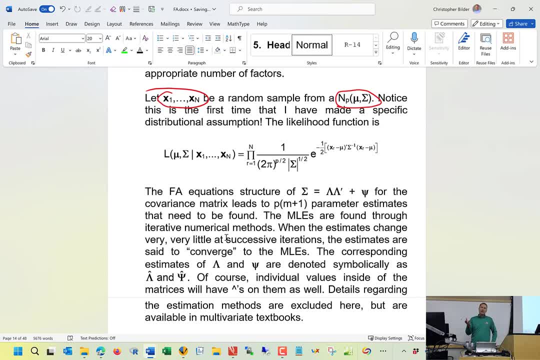 We have something, We will have something like this, And we can assume that it comes from a population that has some Mean vector, Some covariance matrix Defining maximum likelihood estimate. Now we have to assume we also have a probability distribution like this: 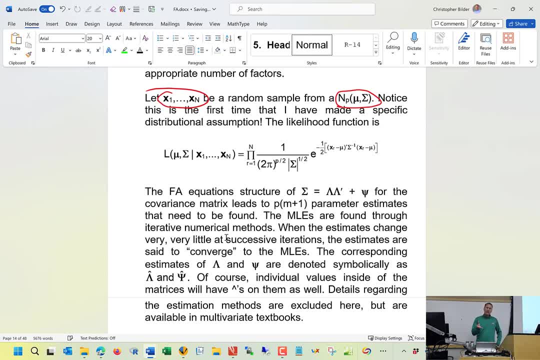 And what is done in factor analysis Is we assume that we have a multivariate normal distribution. So that's why I have the big N there, With a little subscript P, Meaning it's a, The X's have P, It's P by one. 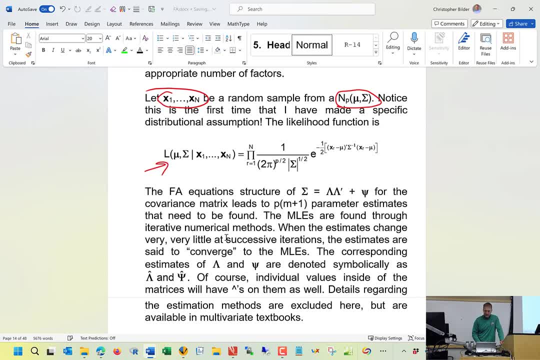 And so now my likelihood function becomes this: Here's my Parameters. And think of the factor analysis model, first written in terms of the X's. Okay, Here are my parameters. I have Capital N different observations, So that's why I'm taking the product from R equal one to N. 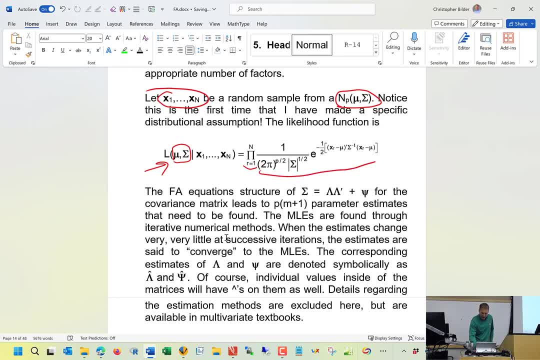 And then I just write out my multivariate normal distribution Where I put a little subscript R On the X To represent For the R Sample value. Now, from looking at that you might be thinking, okay, well, wait a second. Well, where's our 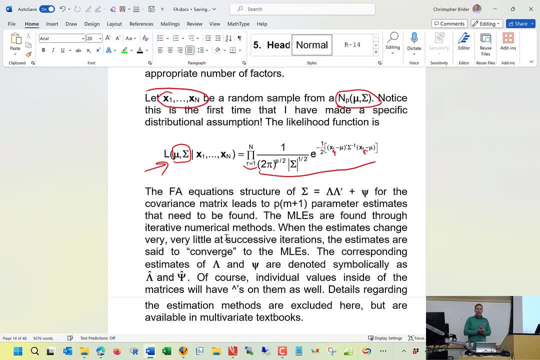 How's our factor analysis model represented in there? Where's my lambdas? Where's those sides that I want to estimate? Well, they're in there. If we think of the factor analysis equations Written in terms of our X's, We have this representation for sigma. 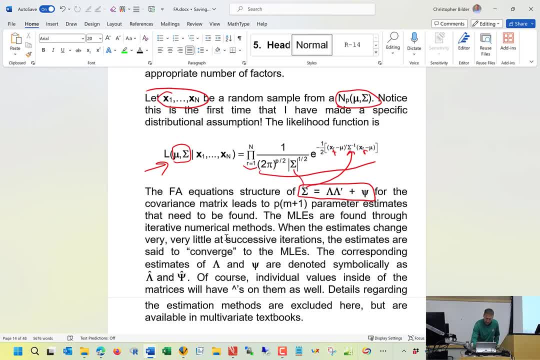 Our covariance matrix, And so that's how we get our lambdas, That's how we get our size In there, And so what we're going to want to do is now Maximize The log of this likelihood function. Find the values of all the lambdas. 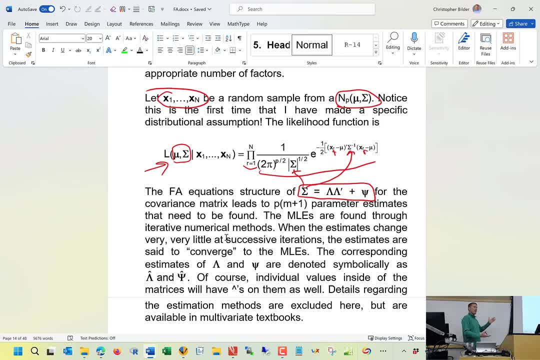 In the size such that this likelihood function is as big as possible, And that's going to be. That will lead us to our parameter estimates, And then we'll actually be able to write out Our factor analysis model With those estimates. Now, if I did have standardized variables. 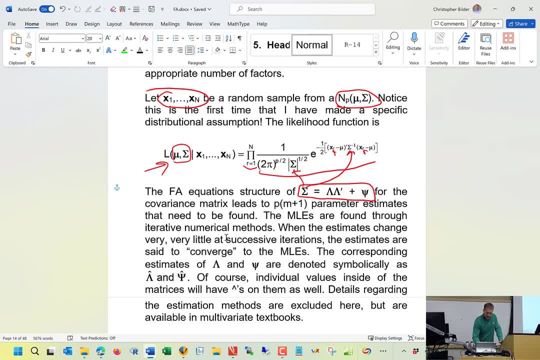 Which we typically will do. Then I just replace the X's With Z's, That mu would be just zero. We would know that The sigma now is going to be represented as, let's say That correlation matrix Is equal to lambda. 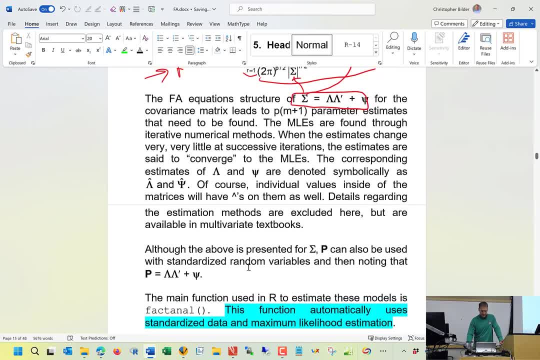 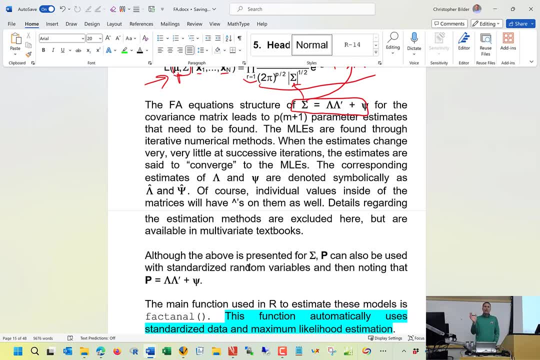 Lambda prime plus sine. Now One Is not going to, let's say, Try to find the The derivatives with respect to the lambdas, Set them equal to zero. Find the derivatives with respect to the size: Set them equal to zero. 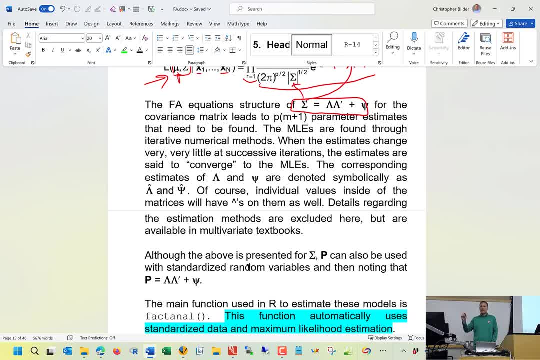 And then come And then solve it all by hand. The reason why you're not going to be doing that Is because it actually takes what are called Numerical iterative procedures To actually find what these parameter estimates are. With that- And probably a lot of you have seen this in other places before- 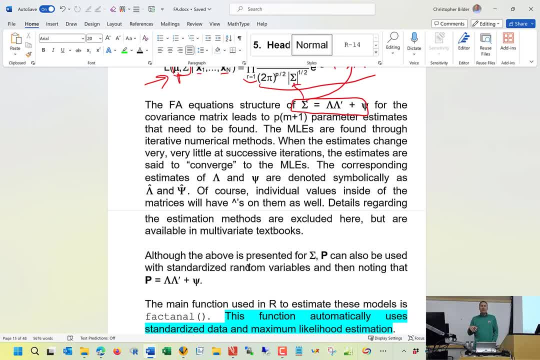 Outside of a statistics course Where, You know, I don't have what's called a closed form solution. You know I can't just say Pi is equal to the sum of the Y's Over N. I can't say that. Instead, what I'm going to do is: 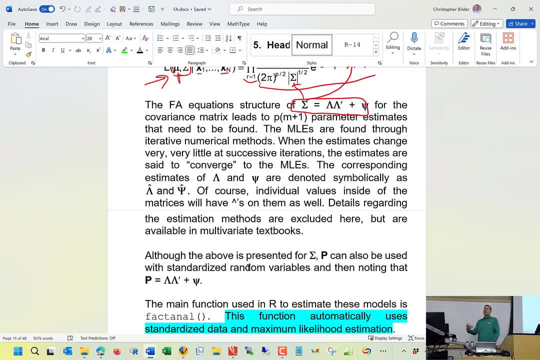 Come up with, let's say, an initial set Of- Let's say, Parameter- estimates, So initial guesses, let's say for the lambdas In the size, And then I'm going to use a Numerical iterative procedure, Maybe for example like: 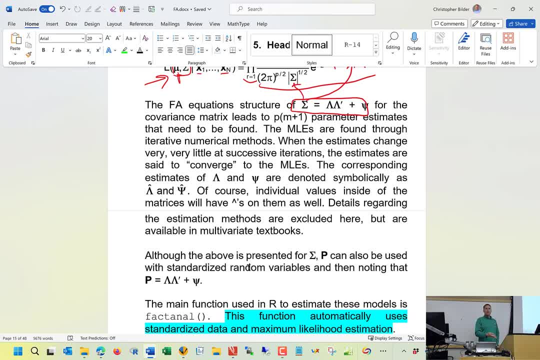 If you've heard of like the Newton-Raphson procedure, Use this procedure to, Let's say, come up with a new set Of lambdas In size That are hopefully going to be better, That are going to maximize Or make that likelihood function bigger. 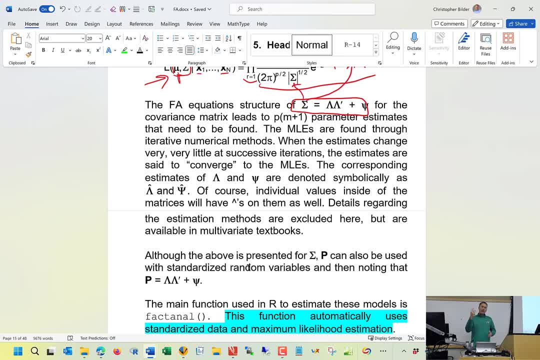 So, And then, After I do that, I'm going to compare these lambdas in size To what I originally started off with. If they are extremely, extremely close to one another, Then I'm going to say, oh, I must have found them. 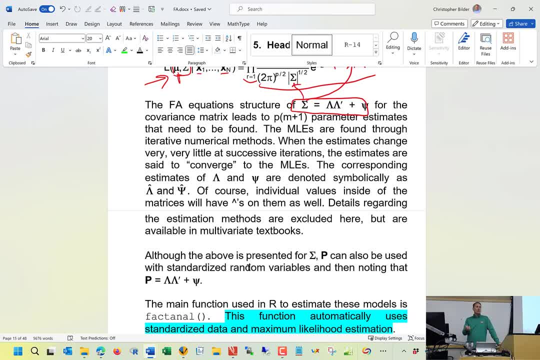 Where that likelihood function has been Maximized, And so now I'm going to use those as my estimates. If they're not close to one another, Then I'm going to put this back into my Newton-Raphson procedure Or whatever numerical iterative procedure that one wants to use. 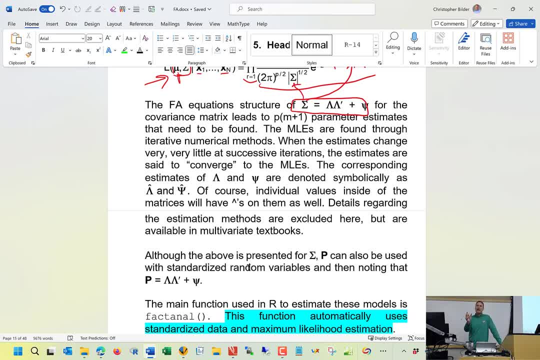 I'm going to put that in there And come up with some even better estimates for the lambda, Better estimates for the size, And then compare them, These better estimates, To what I just had previously, If they are very, very, very similar. 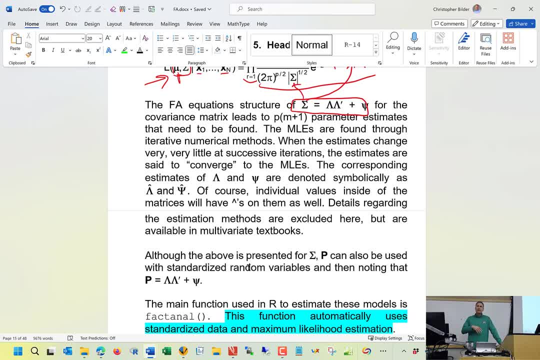 Then, Okay, I must have found Where that Maximum of that likelihood function occurs. I'm going to use this new set Of lambdas in size As my maximum likelihood estimates. If they are not Close, Then I'm going to keep on doing this iterative process. 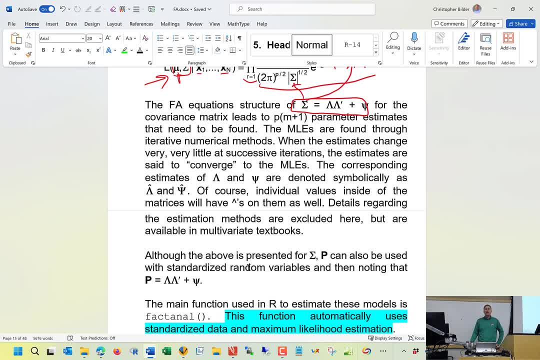 Over and, over and over again To improve my estimates, To find where that maximum Value occurs. Now there might be, And There might be, cases where you're doing this many, many times And eventually You know you get to a point where 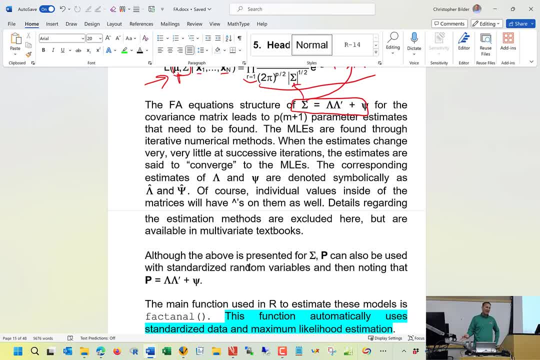 Okay, I'm just going to have to give up. I'm not. I'm not Finding it, And that can happen. So When you do find These maximum likelihood estimates, Meaning for successive iterations, The lambdas and the size, 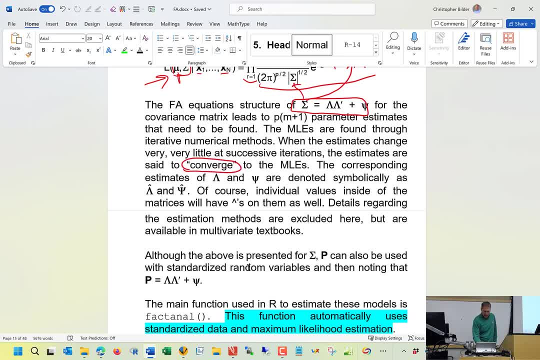 Are very similar to one another. You have The numerical iterative procedure. Has what's called Converged? It has Come to a point Where Things Don't Change anymore If you keep on Doing them, Okay. 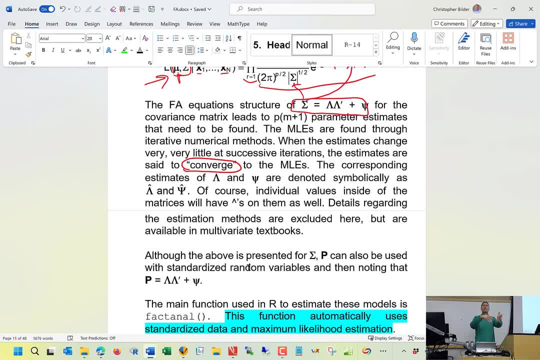 The. If you keep on doing these iterations, Again These parameters Are not Converged. Okay, So Now I'm going to. These programs Are not going to change. You have reached convergence. The factor analysis. 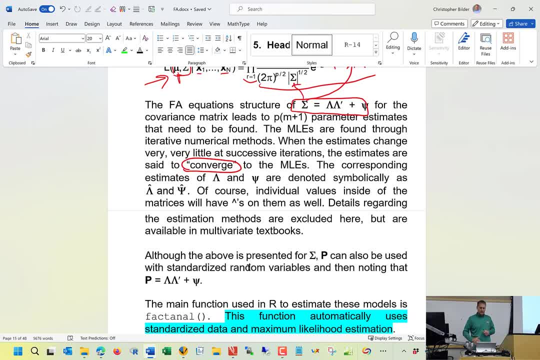 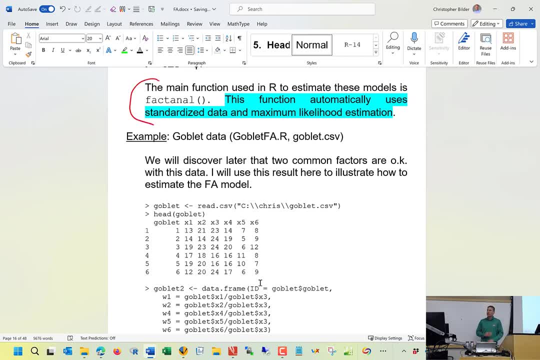 You're not guaranteed To actually reach Convergence. Okay, Now, Finally, After all that, We get To take a Look at an actual Data Example, The main R function that people use To do To estimate these parameters. 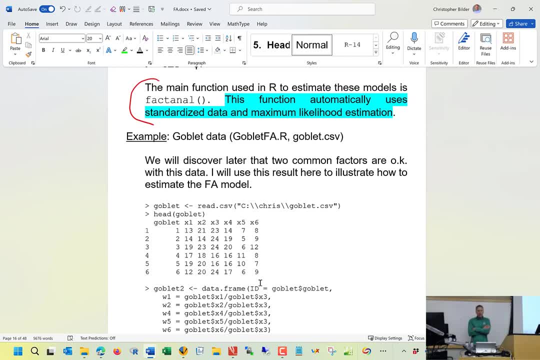 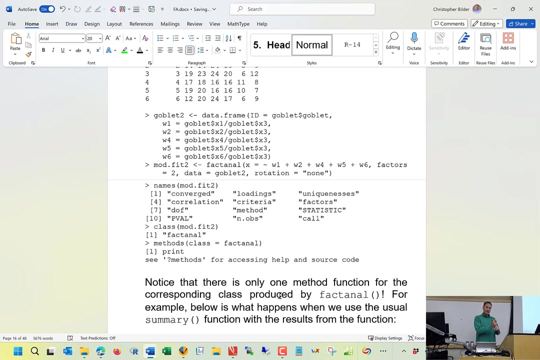 And do other stuff With factor analysis, The main functions Called fact Analyzer. Okay, this function automatically always uses standardized data, so you, you don't have to pass into it the standardized values, it will automatically standardize the data for you and it will automatically. 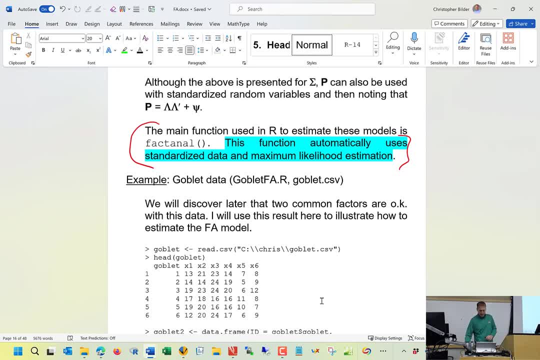 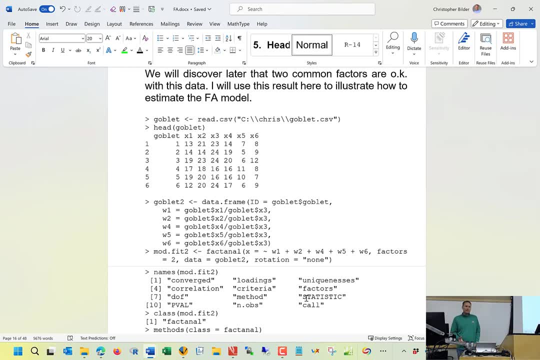 use maximum credit estimation. okay, so let's go to the goblet data. what we will find out later with this goblet data is that two common factors are okay, and so I'm going to use two common factors now and again. later we'll talk about how I 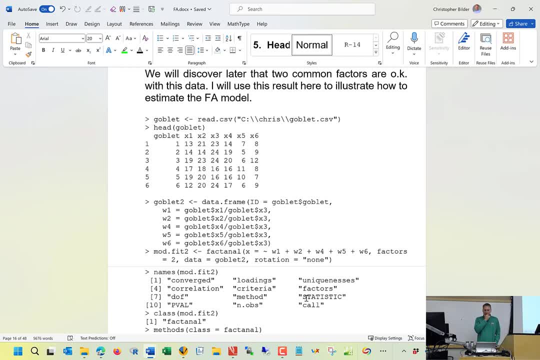 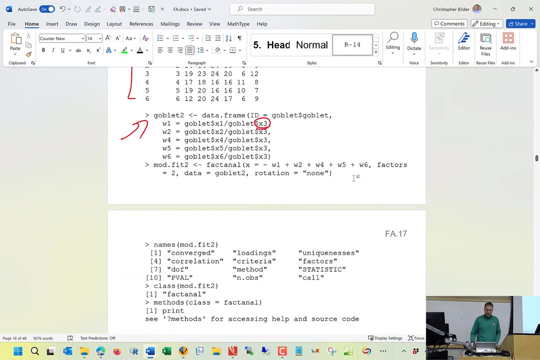 came up with that decision. so I read in my goblet data, as we've done before. I make a little adjustment to it to count for the overall height of the goblet data as what we've done before and now to actually estimate the factor analysis model, I use the fact annul. 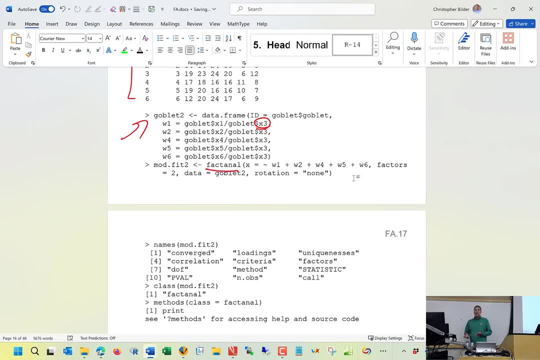 function. the syntax for it is similar to what we saw with print comp. if you remember, print comp would say formula equal tilde, w1, w2 and so on. here, instead of using formula, that first argument is X. it's just what the authors of the function shows. 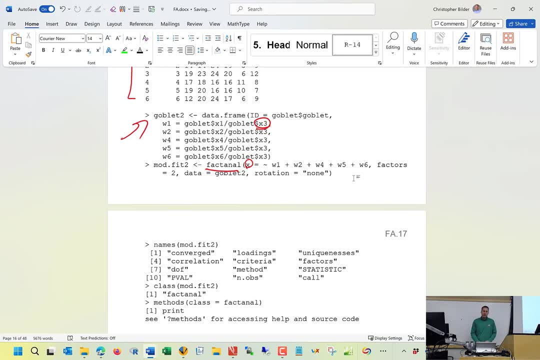 so I say X is equal to tilde w1 plus meaning and w2 plus w4 plus w5 plus w6. there's an argument called factors. that's where you specify how many common factors you want. you can also specify where your data is. and there's a last. 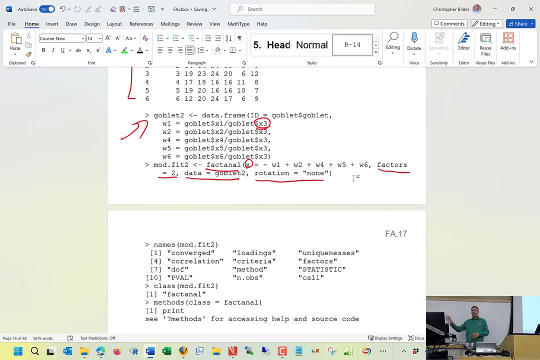 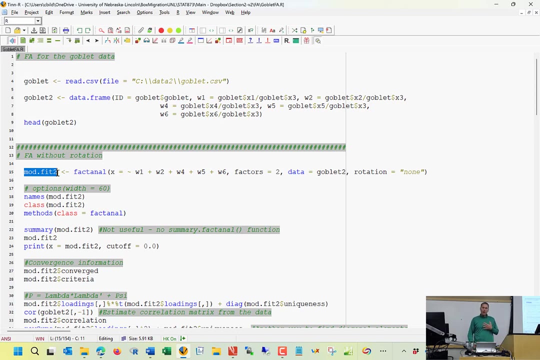 argument called rotation. I will explain that more later. for now, let's just use this particular value called none and I'm going to use this particular value called none. okay, I'm going to put the results from running this function into an object called modfit2. where does this name? 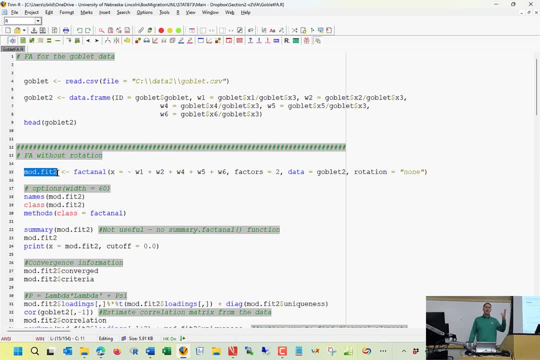 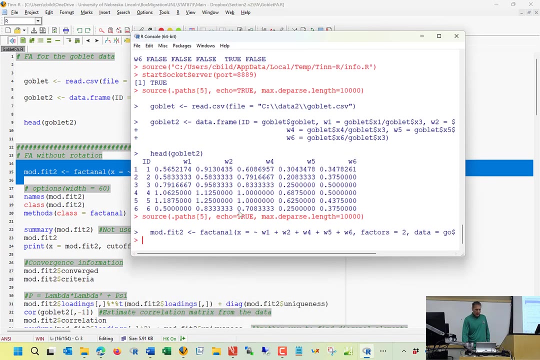 come from model fit, two common factors. that's why I chose it. I could have chose some other naming name if I wanted to. okay. and so now, whenever you again approach a new or use a function that you really haven't used before in R, one of the first. 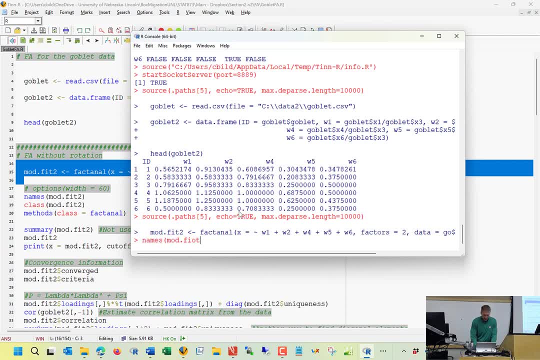 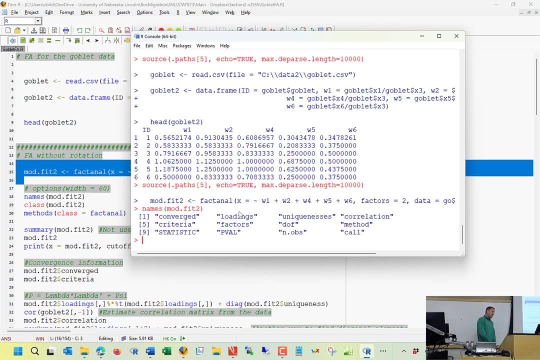 things that you should do is to use the names function with it so that you can see what's actually stored inside there. modfit2 ends up being a list in terms of R's terminology, and so we see some names of stuff in there. that kind of. 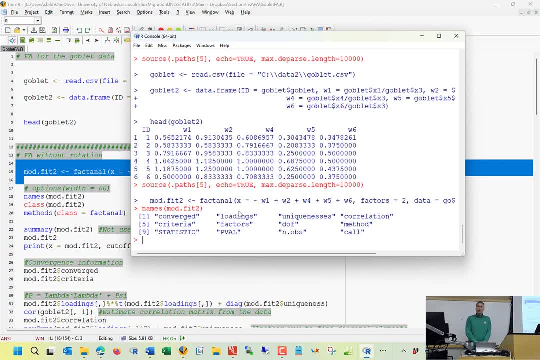 look familiar to us. so, converged, this will tell us, hey, did my parameter estimates converge? I have information such as loadings. remember the lambdas? the formal name for them is the factor loadings. ah, there's that. you name uniqueness. remember the specific variance? another name for it is: 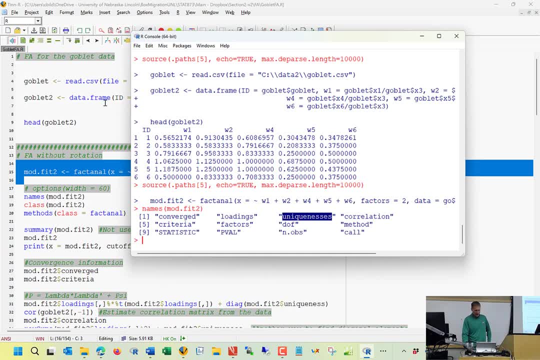 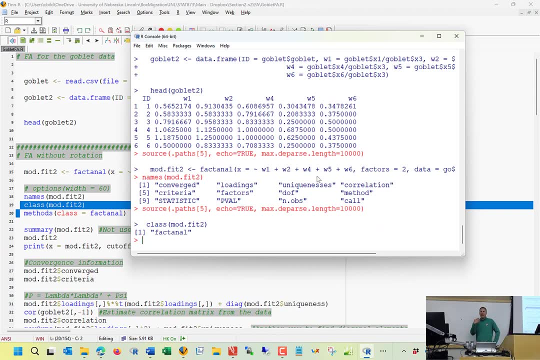 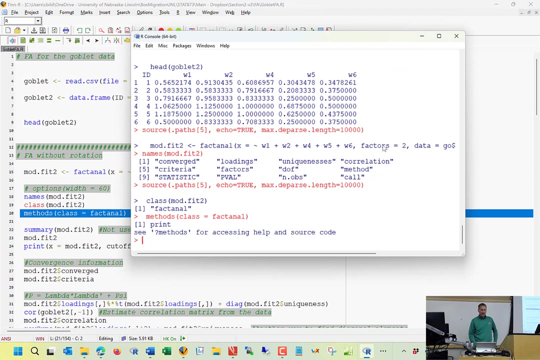 uniqueness correlation as well. we can also use the class function here to see: well, what's the class of this object? the author's decided to call it exactly the same name as the name of the function itself, and so with that then I can say: methods, class, equal, fact, animal and I. 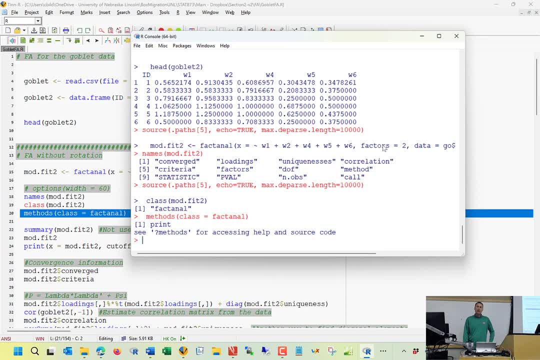 can see all the corresponding method functions with us. when we did principal component analysis, we had more method functions. here we only have one print. we'll look at that shortly. and then I think this is kind of disappointing how the authors decided to to structure this, and so you might you know if you 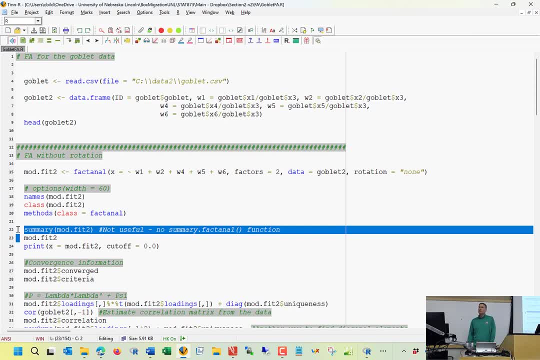 remember with print comp we had a method function called well, did you know the method? we had a method function for summary. so what that means is, if I did said summary, parentheses the results from print comp and parentheses, I get a nice summary what's going on. but here we didn't see summary as one of 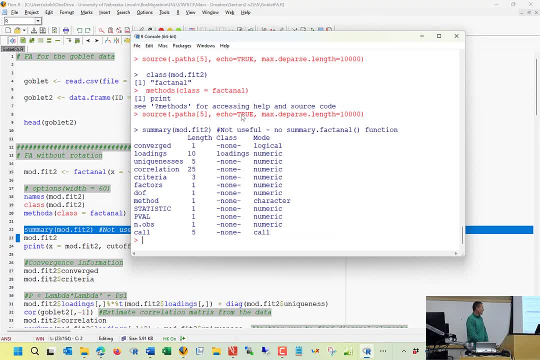 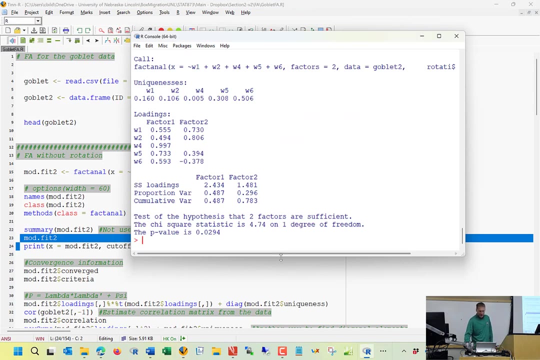 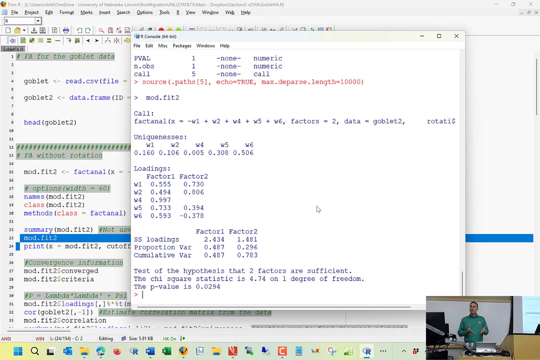 those methods functions, and so if I apply summary to that, you really don't get anything much really useful. but instead what I need to do is just simply type modfit2 and this is then what I get. I don't get everything that's inside of what modfit2 has I get. 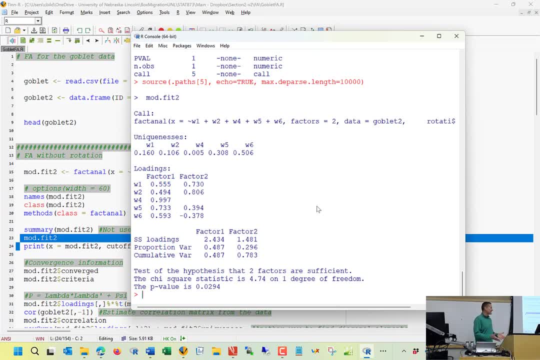 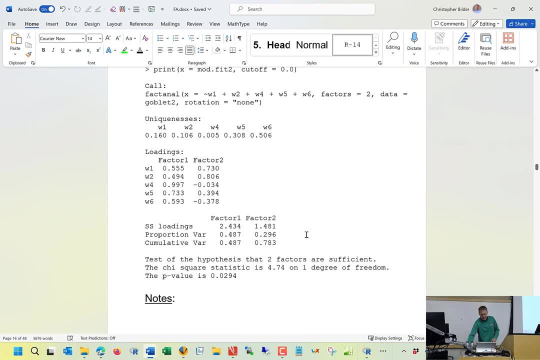 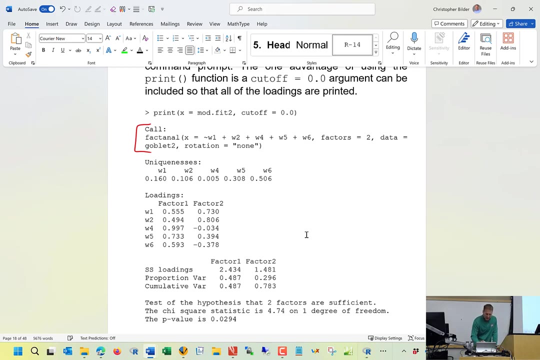 essentially my summary that you might expect. let me actually go back over here to my notes. I can write on this. so we have information that says: okay, how was this implemented in terms of the actual code? here's my uniqueness. so psi hat one. the estimated specific variance for the 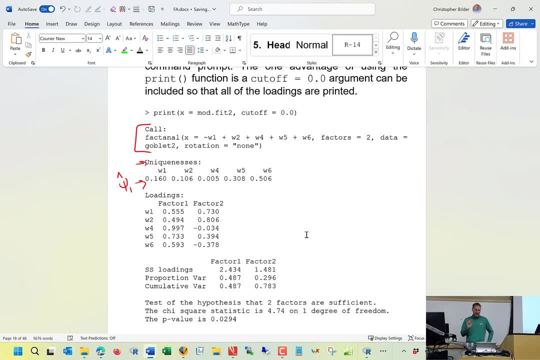 first common concept for the first specific factor is 0.16. I have a table called loadings here. here's my lambdas. so, for example, this is a lambda 1: 1. I'm going to put a hat on it because these, these are actual maximum, like the. 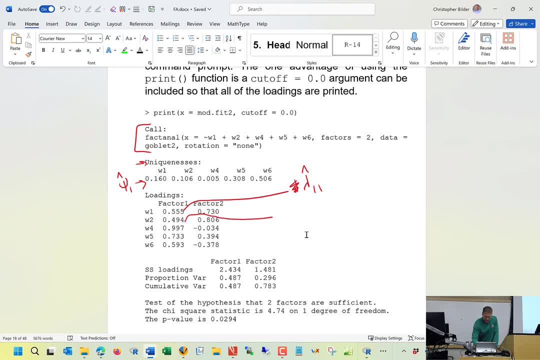 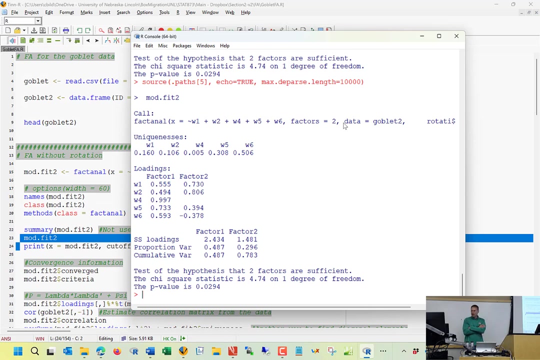 decimals. here is lambda 2: 1 hat 0.494. I didn't skip over something. I apologize right here. so if I just said modfit2 here, this is what I get, which looks very similar to what we just saw. there's one difference, notice. there's 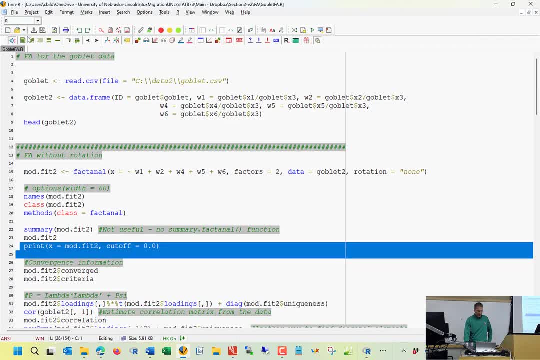 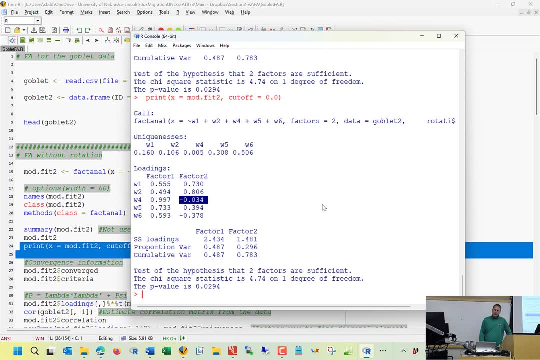 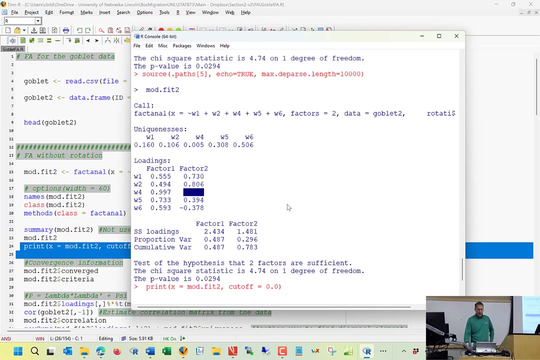 nothing there, but this was actually what was displayed in the notes. I do have something there. okay, so by default, R will not print some of the some of the factor loadings, these lambdas, if they're close to zero I don't really think it's a big deal, just just print it off, I can. 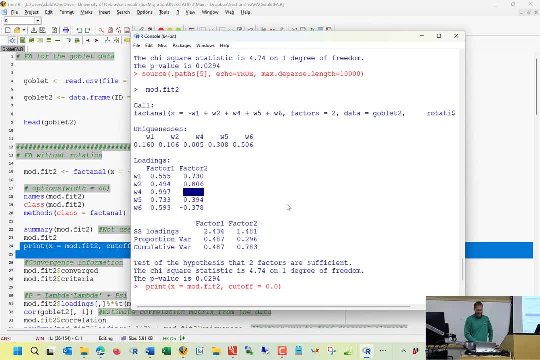 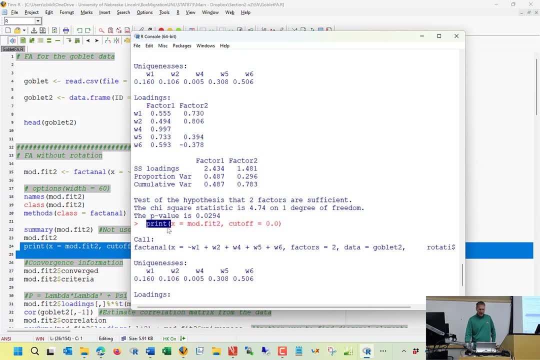 see that it's close to zero. you don't need to hide it from me, and so a way to deal with that- and this is what I always do- is I take advantage of that method function for print that we saw. I think print first argument is X mod that fit. 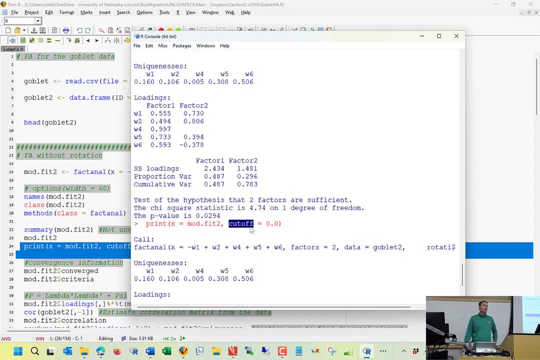 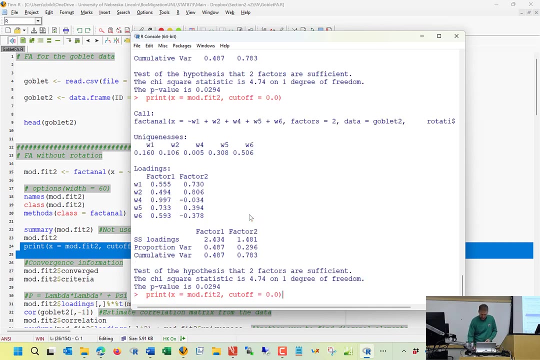 too. and then I added argument called cutoff 0.0. so that means essentially it will print everything, even if it's very, very close to zero. if instead I did this just to show you how that works, suppose I put cutoff 0.1 there. now we can see how that one value 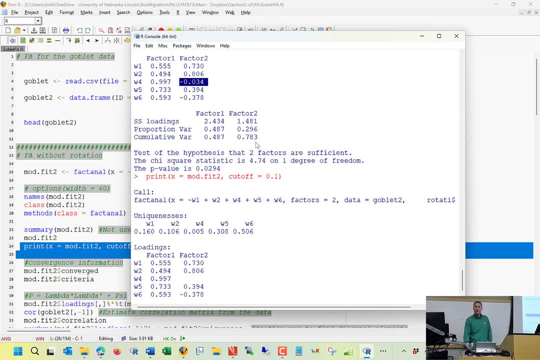 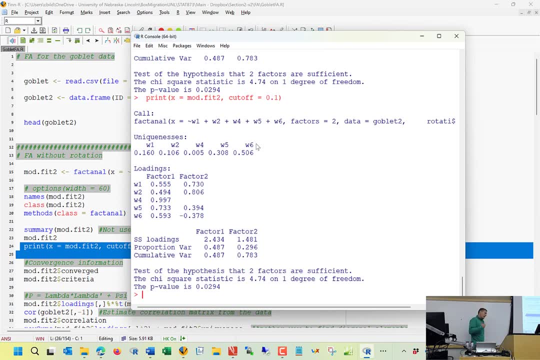 was hidden because the value was negative: 0.034, so it was within point 1 of 0. now, just so that you understand how R works here. basically, whenever you are doing this, you will get to an object name, and I'm going to do this by type an. 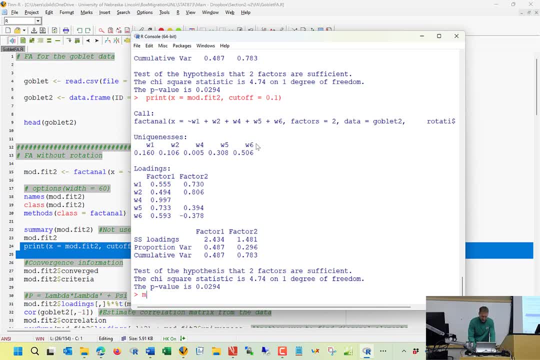 object name in the R console here like mod, that to. or, let's say, if I estimated a regression model from, let's say, using the LM function and I typed, let's say, if I called it, mod dot fit, whatever I type, that what are is going to do is all. 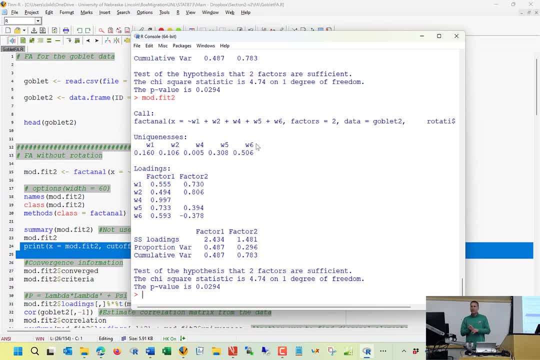 Is there a corresponding print function, print method function for it, and it will automatically implement that. So even if I type modfit2 here, what R is going to do is look: is there a print function? And if there is, it's going to actually implement it and run it. 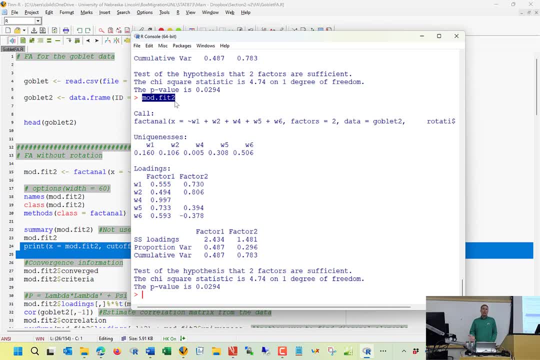 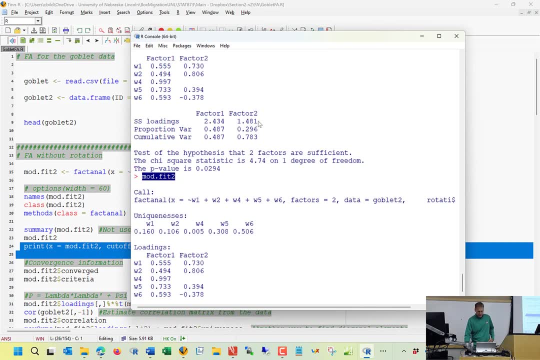 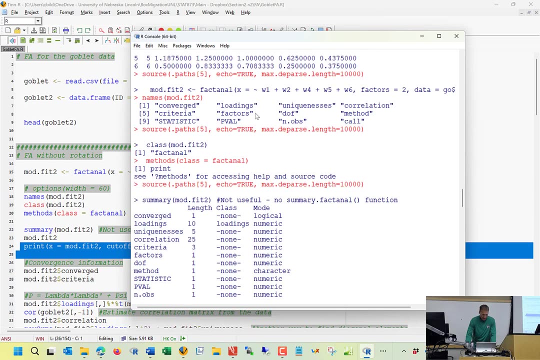 It's just kind of a weird way that this is how R works. If there wasn't a print function, what will happen is- and perhaps I'm getting a little bit farther than what we need to know, but what will happen is this, with a list, 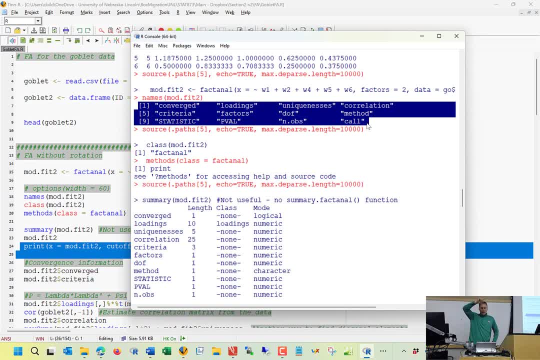 It will actually print off the value for converge, print off the value for loadings, print off the value of uniqueness. print all those values off. It will print every single value that's within that list If there wasn't a print function. 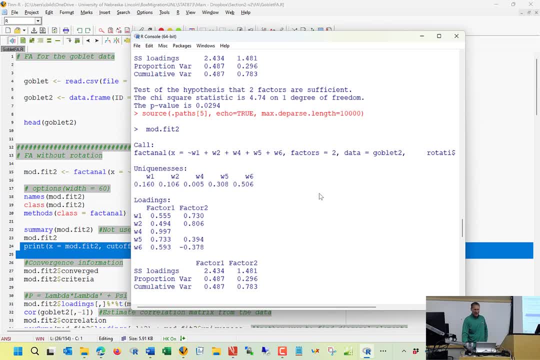 What? That's a good question. Do you want to say that more specifically in terms of what the Because use? I mean, we saw that there were only one function and that was print, Yeah, so Okay. So this gets into, you know, my introduction to R and R2.. 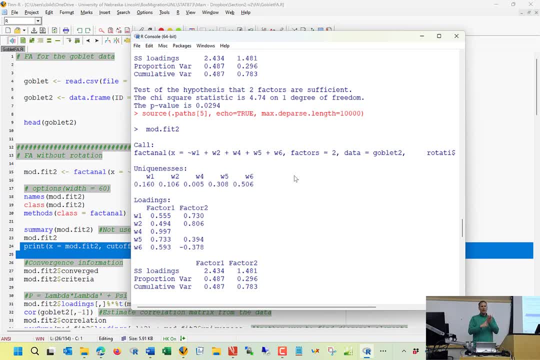 It's that R is an object-oriented language, Depending upon the class of the object. that's how R is going to, let's say, run particular functions associated with it. So you know, there are generic functions, There are method functions. 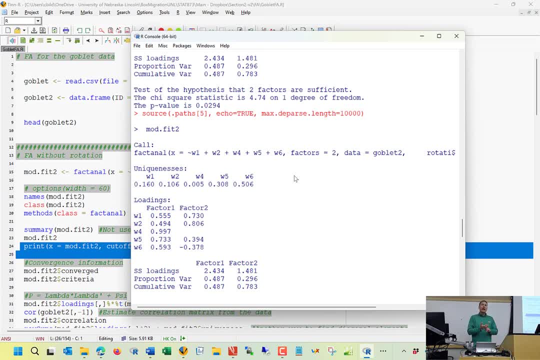 A generic function is like summary, like print. A method function is like: in this case, there should be a method function called printfactannal. Okay, And so when I run The print, and so when I looked at, when I looked at this, I saw that there happened. 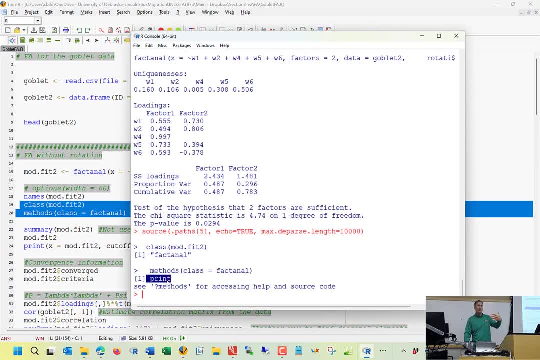 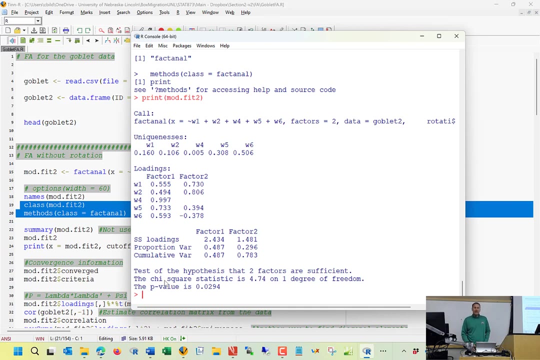 to be only one generic function that's associated with this particular class And so when I actually now run that generic function with modfit2, it finds a function called printfactannal and it actually runs that Now in general. now I think this is maybe getting at your question. 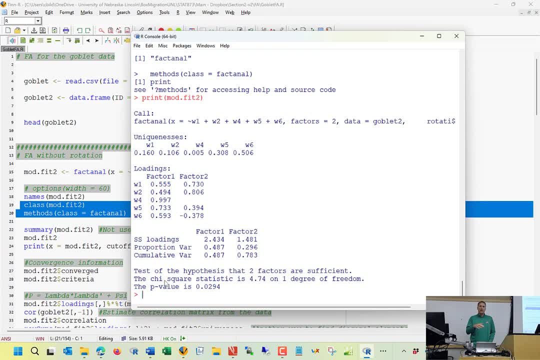 In general. now for how R operates. again, it will look to see if a particular object has a method function associated with it, associated with a generic function. Okay, Okay, If it doesn't, it will actually run, What, in this case, would be printdefault. 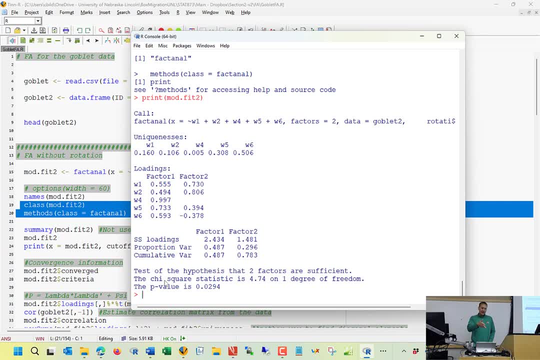 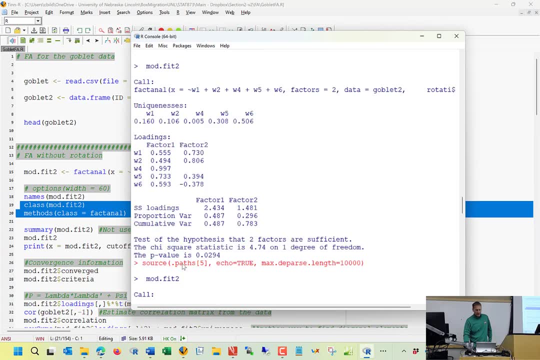 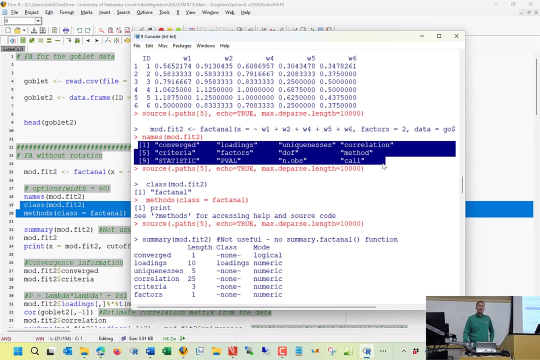 And what will happen if, let's say, this print did not exist? it will actually list off all the numerical values corresponding to the 12 different components of this list. Okay, Okay, Go ahead. Sorry, Do that printfactannal and it will be the same as this. 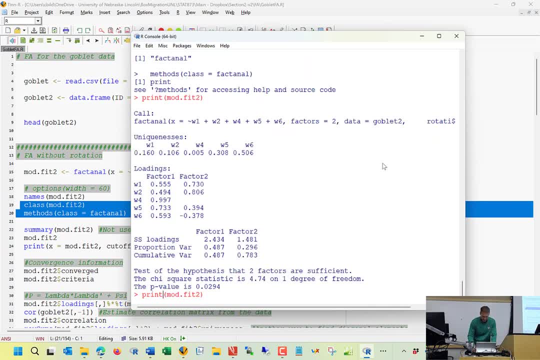 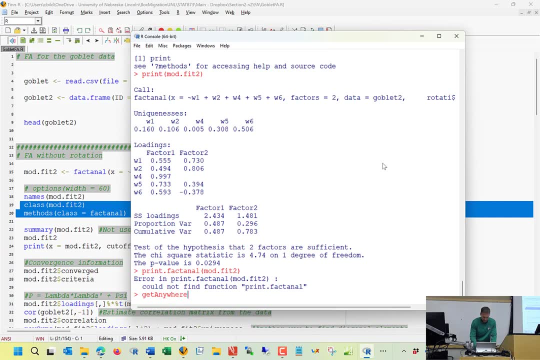 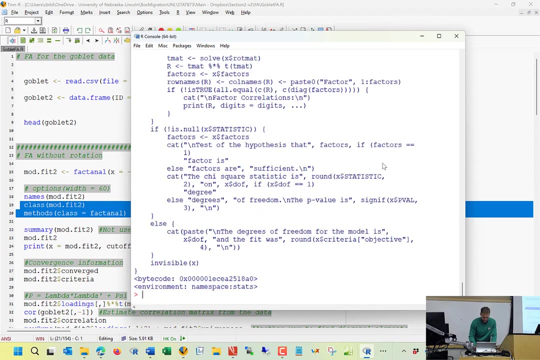 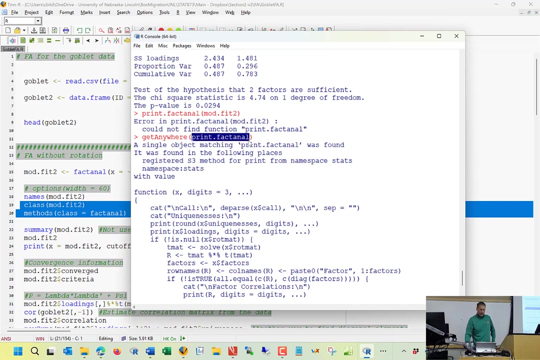 Yes, Okay, So we can see that there's a function called getAnywhere. It helps me find where that function is, and we can see that it exists. When I actually tried to run it, it did not work, And this happened about 15 years ago. in R. There are ways to limit your access to particular 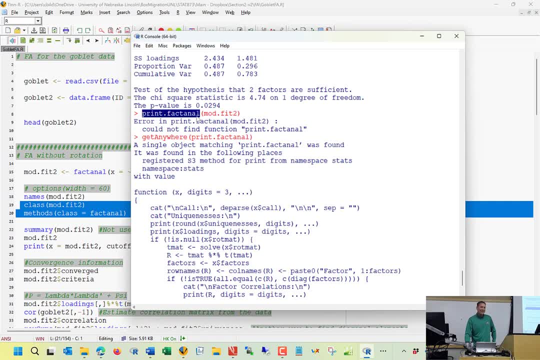 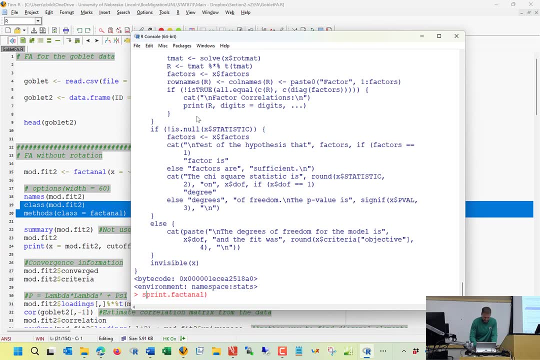 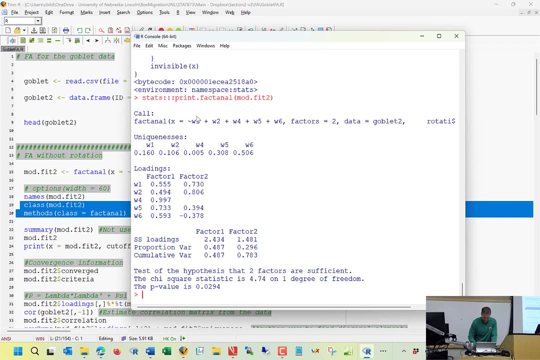 functions, because you know why. would someone want to run this directly? Well, you don't, And let's see if I can get it to work. Okay, So there's a little bit of a trick here, and most people don't see this or haven't. 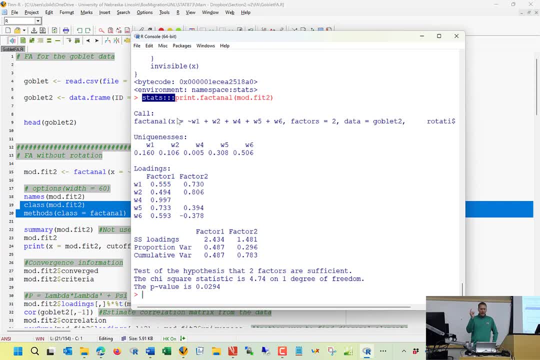 seen this, I bet. So the factannal function actually exists in the stats package And so, because of that, you would expect corresponding method functions to be able to run this, And so you would expect corresponding method functions to be able to run this. 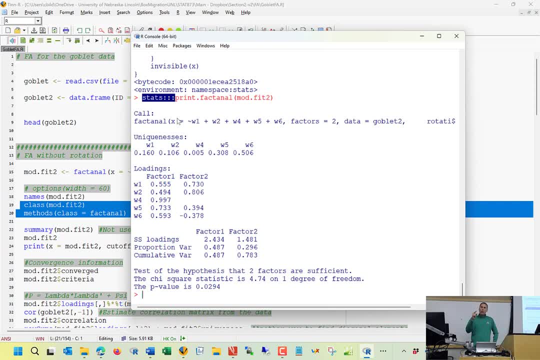 And so you would expect corresponding method functions to be able to run this, And so you would expect corresponding method functions to also exist in that same package. So if you ever wanted to specifically say I want this function from this particular package, the syntax is you put the package name: colon, colon, colon, the method function. 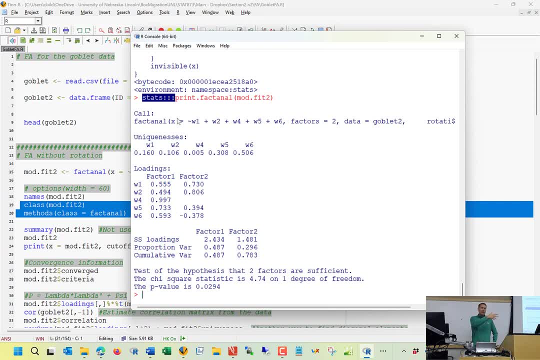 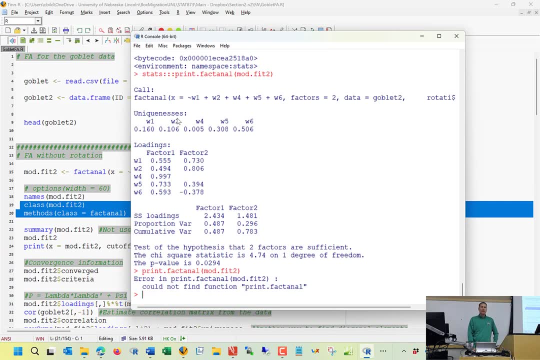 And that's why I was able to get it to work there. For some reason, it was set up so that if I only do this, it doesn't work. Now why? Why does R give you this kind of an option? You could have, let's say, multiple packages that are loaded in what's called your search. 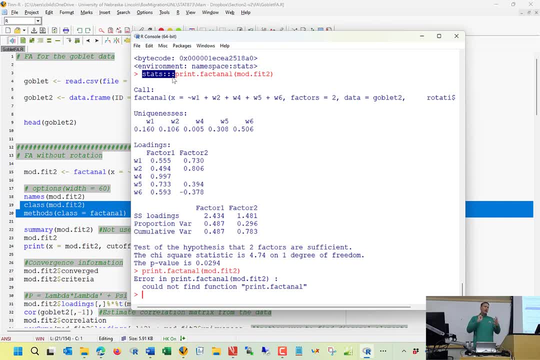 path, meaning that R says: okay, I can look in this package, I can look in this package, I can look in this package for a particular function. These packages may have the exact same function names in them, even though they do different. 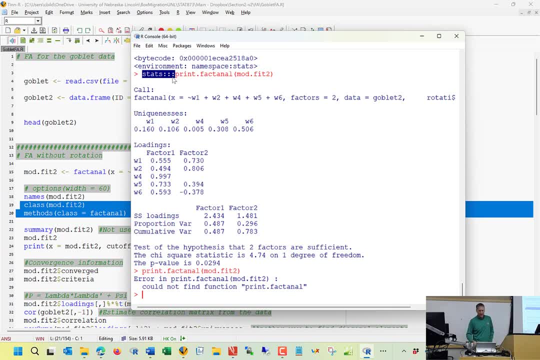 things, And so that's why R gives you an option like that to be able to specify it. So You know, I guess what I've talked about now for the last few minutes is a little bit more beyond than what we need to know, but I like to talk about it here because I understand. 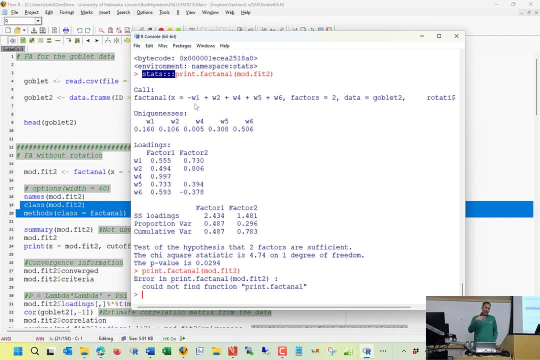 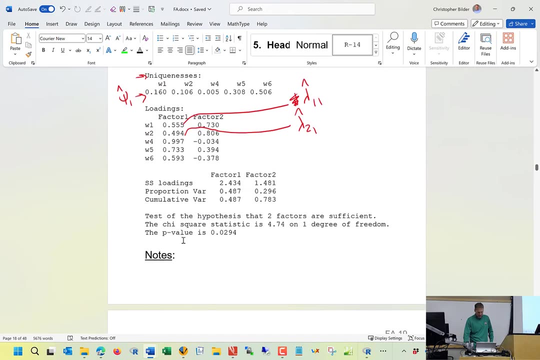 that many of you are maybe new to R or don't have a whole lot of experience with it. Any other questions about that? Okay, let me come back here to the notes. Let's see here. Yeah, just to make sure I didn't. maybe I didn't explain this to you. 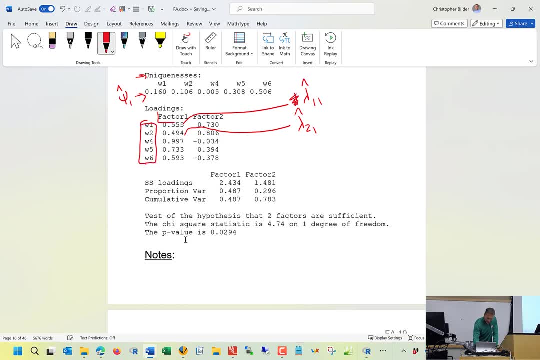 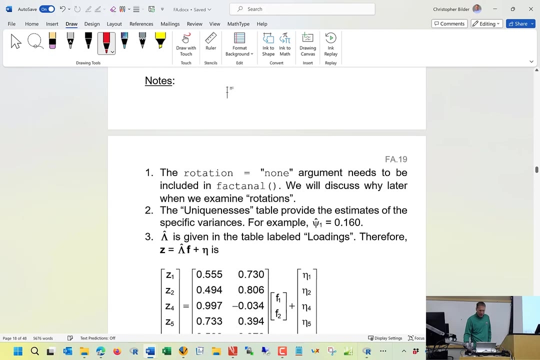 So obviously we can see those are the original variable names and notice how we have factor one, we have factor two there. That's how I knew where which lambda was with what. Okay, So a very hopefully easy question that I would put on a test would be okay, go find. 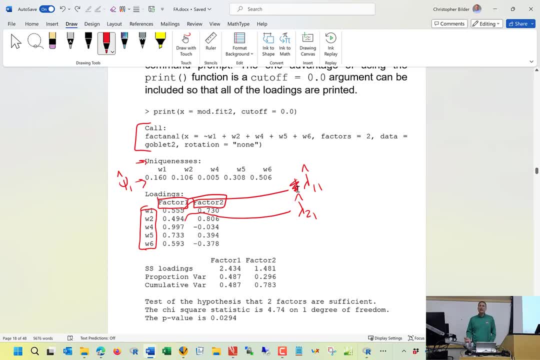 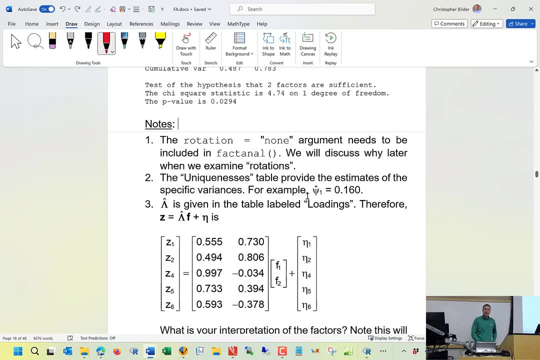 the factor analysis model for this data. Write out the estimated model. So what is the estimated model here? Unfortunately, I can't get this all on one screen, So I write out the z's. Here is my lambda hat one, one that I pointed out before. 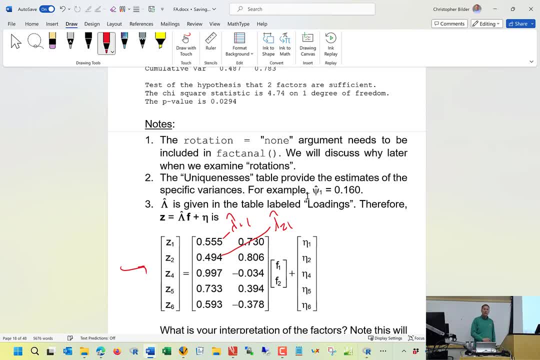 Here's my lambda hat two one. I'm writing it all out. Here's my f vector. Here's my a vector. Here's my z vector. If you wanted to, instead you would just simply write this out as z. one is equal to .555 times. 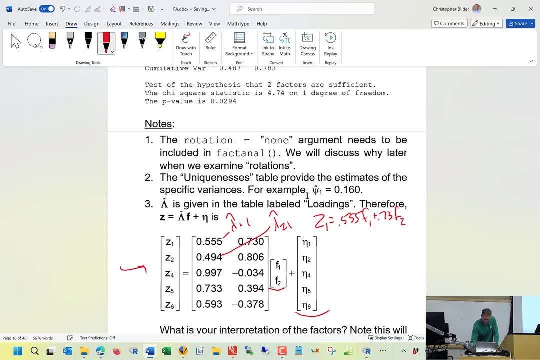 f one plus .73 times f two plus eta one. Z two is equal to .494 times f one plus .806 times f two plus eta two. You could write it out like that too, So you simply call it estimated. This is the estimated model. 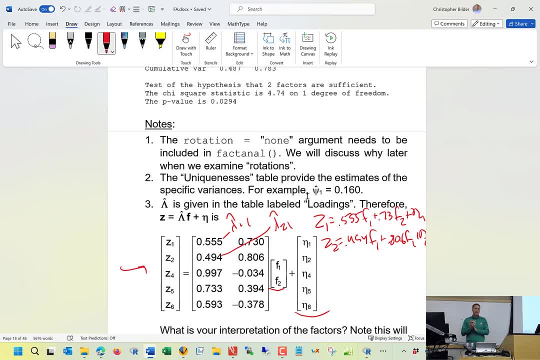 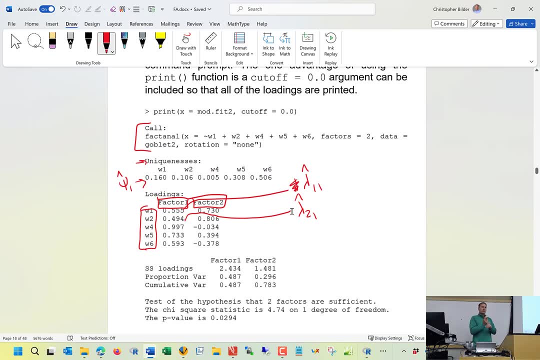 And we have to just write it in, for we cannot get the answer from R. Well, well, I mean, yeah, from R. but So on the test, I might say: okay, here's a data set. Go, estimate the model. 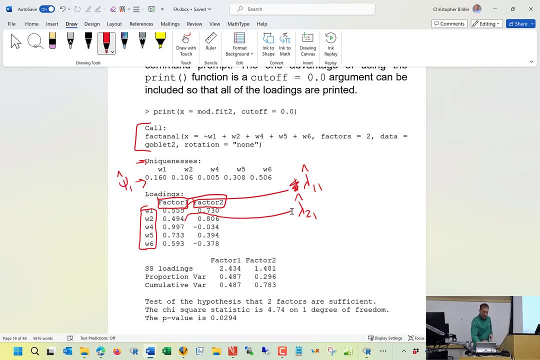 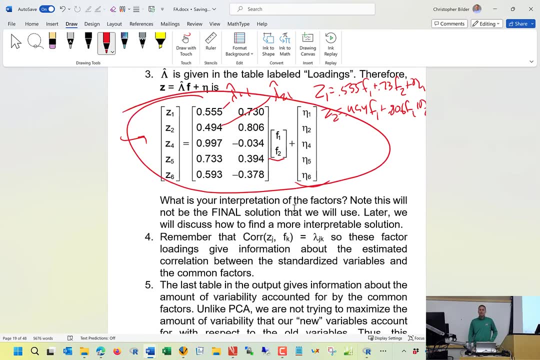 Write out what the estimated model is. And so you would do, you know, the fact analysis step. You would do this step And then you do this step, And the reason why we want to be able to write it in is because we want to be able to write it in. 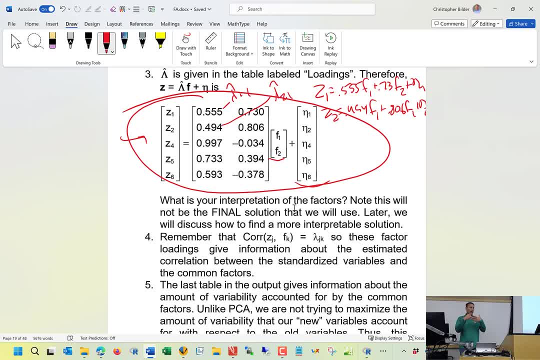 And we want to be able to write it in, And we want to be able to write out the model like this so that we understand. okay, this is how factor analysis is saying that Z one comes about, how Z two comes about. 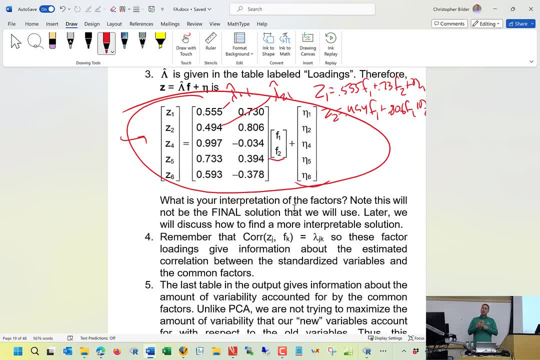 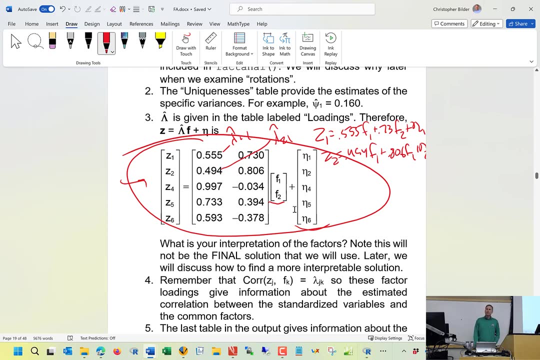 But also now we can start thinking about how can I interpret f one and f two. So let's see here. So what would you say that f one is essentially representing here? Relative to, Relative to the goblets. So let me actually get that goblet. 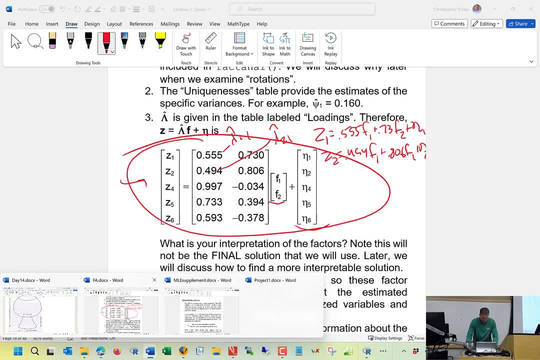 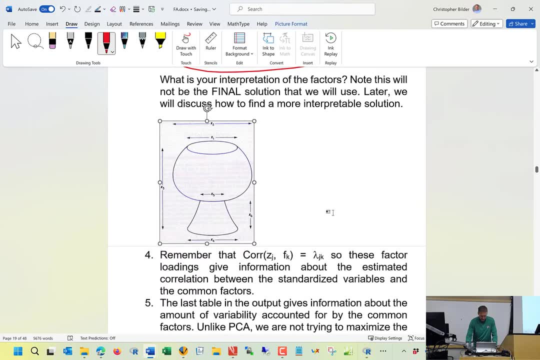 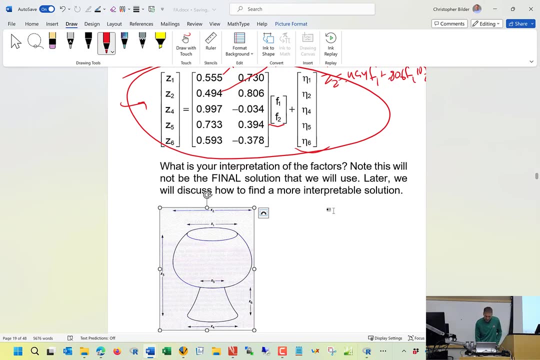 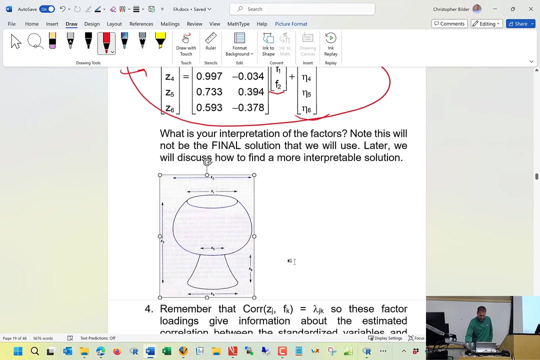 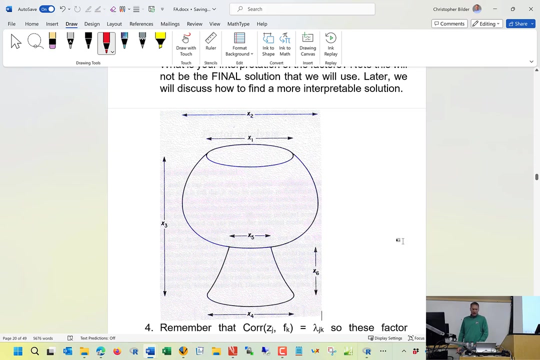 There we go. Yeah, it's kind of small. So x one and x two Are Are at the top of the goblets. Let's actually just blow it up: X four and x six are at the bottom of the goblets. 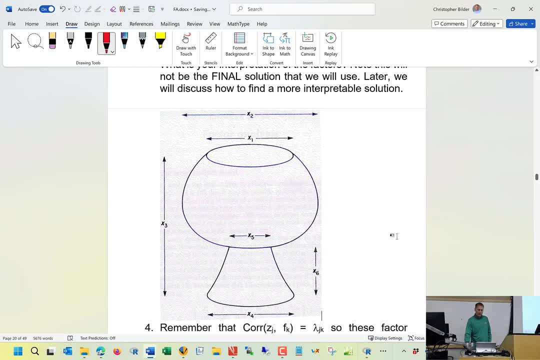 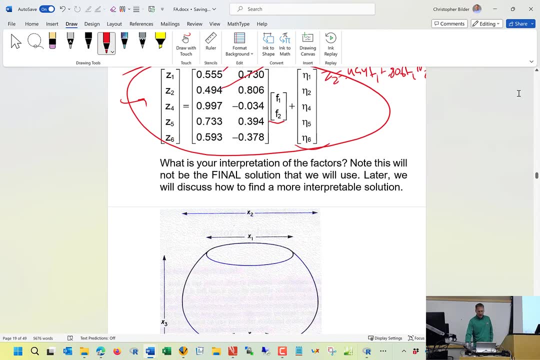 And x five is the connection between the two goblets, Or parts of the goblets. So what would you say, then that the first common factor is representing? Think about it, Think about what we have for principal component analysis, How we would, how we interpret the first principal component. 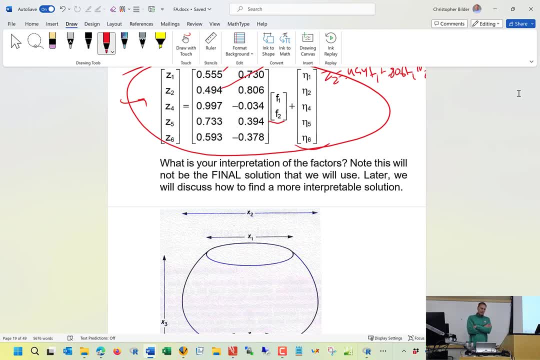 The connection of the goblets x five- Say that one more time, please- Will be the connection x four and x five. with how like the bigger value? Yeah, yeah, so so x, x, four, z four, obviously. 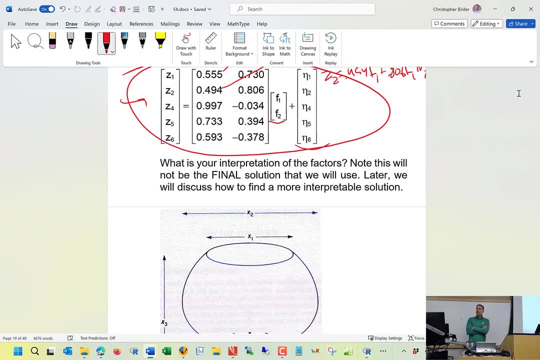 is strongly related to the first common factor And, remember, these are essentially correlations, So that's playing a huge role. The other variables are playing an important role as well, And so you could just kind of say this is maybe just an overall measurement of the size of that goblet. 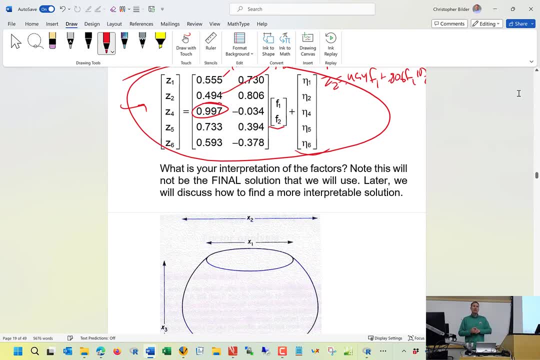 Where there's essentially more weight on that component And that connection. that connection is very important. Let's look at the second common factor. Notice that the z one and z two have corresponding factor loadings that are positive. Z five and z six are negative. 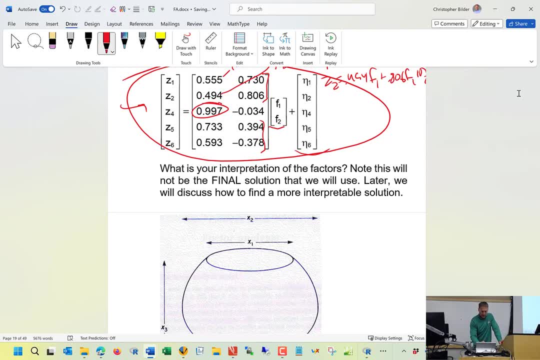 And they're a little bit smaller. in terms of that, what that correlation represents, Z four itself, Now, it's not representing much at all. And so now here I would say: okay, I know, one and two, z one and z two represent the top. 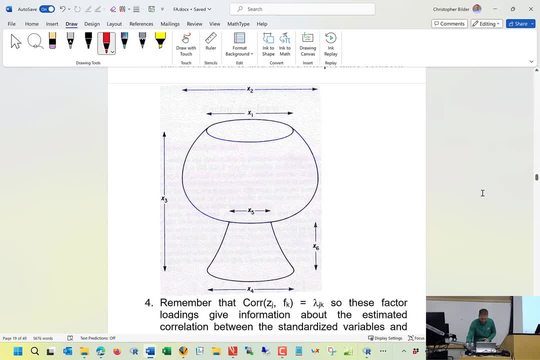 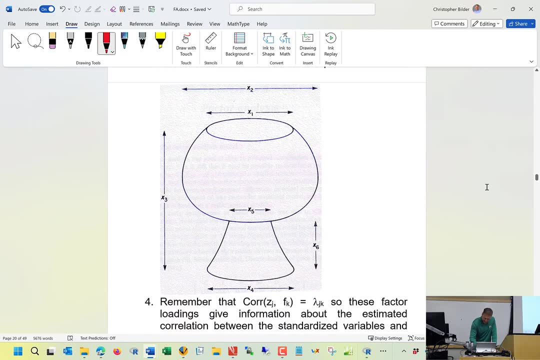 Five and six represent the bottom. Just verify that. I'm sorry, Excuse me. Four, excuse me, Maybe I misspoke before. Four is the width of that base. For some reason I thought it was this one here, But no, I was wrong. 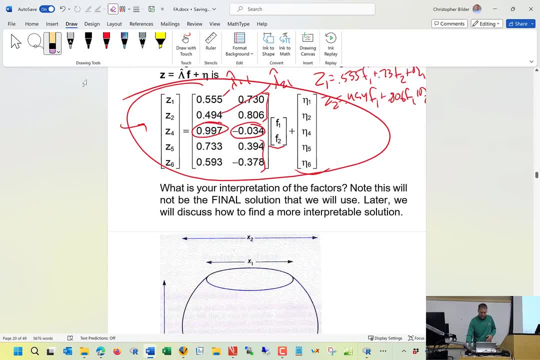 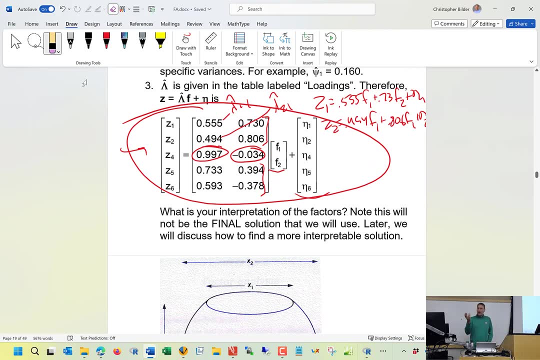 So four is the width of the base, And so basically, what common factor two is representing is a contrast or comparison between what's happening with that very top part. You know, in terms of the opening, how big the opening is, how wide the total cup part is. 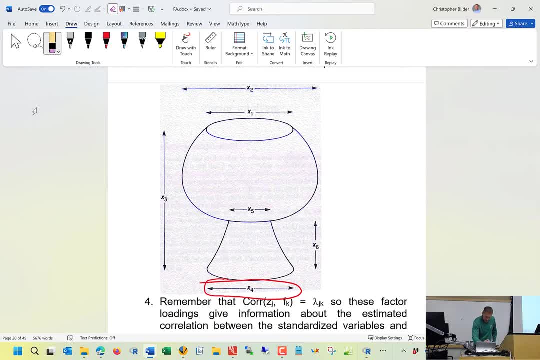 In comparison to Five and six, which is, I don't know, I guess you could say some measurements of the base. It's leaving out one measurement, But you know, if I was an archaeologist, maybe this might make some sense relative to my understanding of the science behind this. 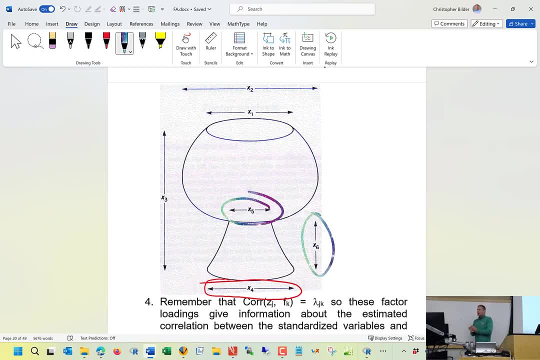 Now you might be wondering: well, wait a second, Chris, Aren't we looking at factor analysis? because we have, Because you said We can come up with better interpretations of our dimensions, of our data, and that's true. There's going to be one thing that we're going to be starting to look at after this example that allows us to actually change what those lambdas are, those lambda hats are. 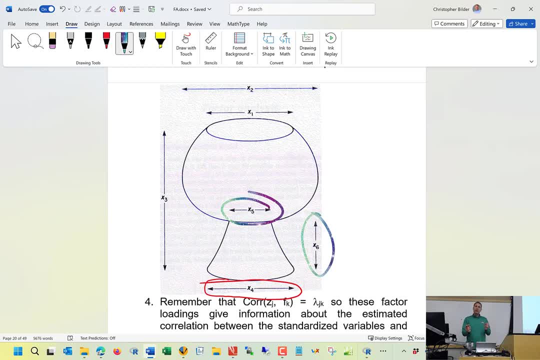 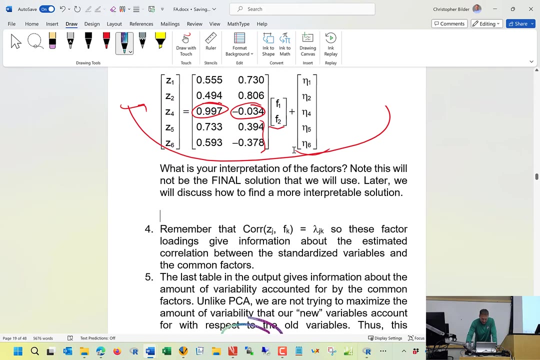 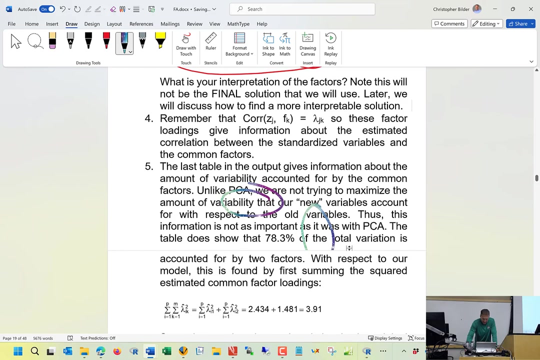 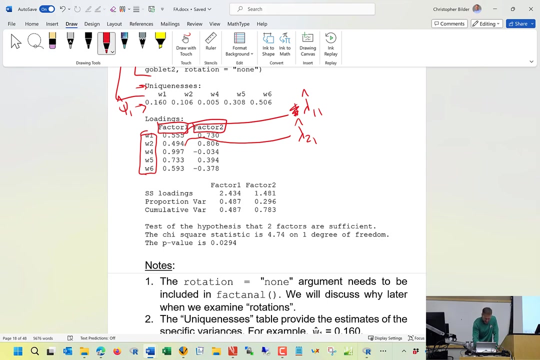 And if we can change those lambda hats, perhaps then we can come up with an easier interpretation And maybe what we have here, Okay, Okay, Let's look back here in the output some more. We have some parts of the output that look familiar to us relative to what we have for principle. 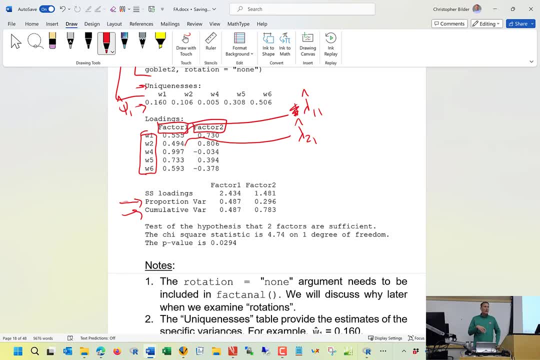 So, for example, we have some parts of the output that look familiar to us relative to what we have for principle. So, for example, we have some parts of the output that look familiar to us relative to what we have for principle. Proportion var. 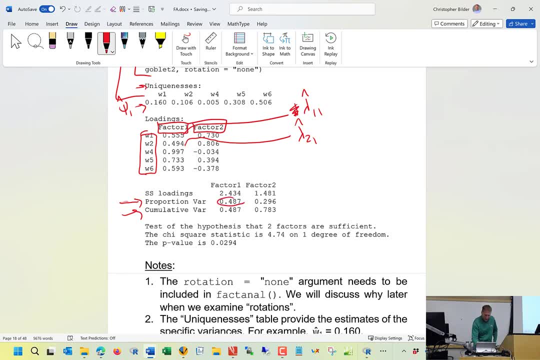 The proportion of variance that common factor one accounts for. Then cumulative var is the cumulative proportion. So two common factors account for 78% of the total variation in our data. Now for principle component analysis. we really really focus on that. 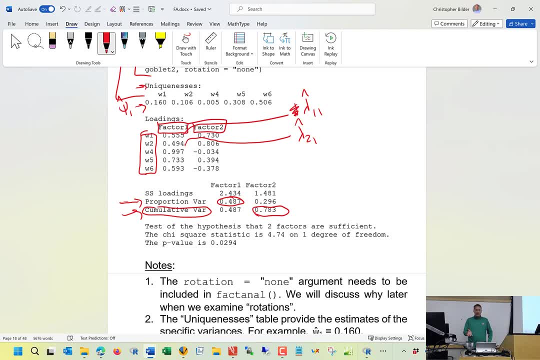 For factor analysis? actually we don't. It's interesting to know that And I give some information in the notes about how these calculations are actually made. But in the end in factor analysis you typically don't focus on that. We are going to focus on some other measures that help us make a judgment about okay. 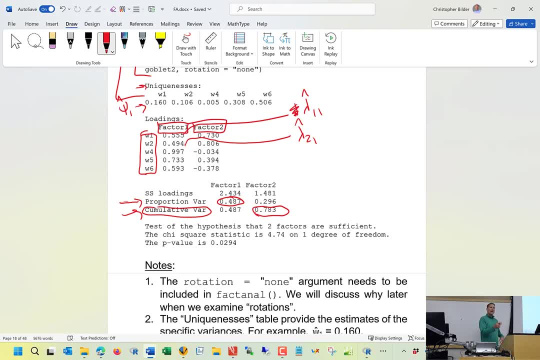 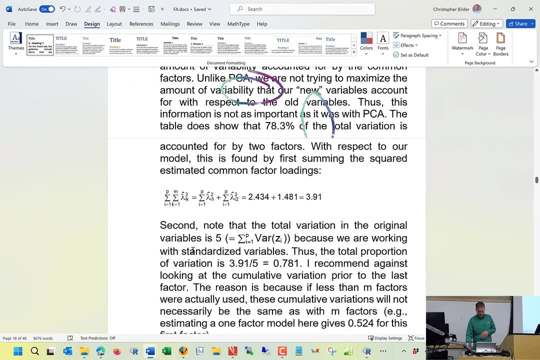 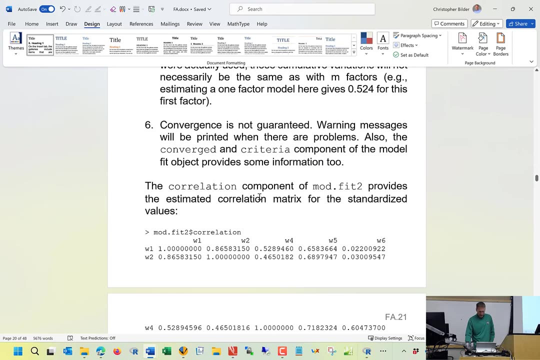 is this factor analysis model really accounting for most of the information in our data? So stay tuned for that. Is that a reason why you know, like you know from the model? if you take in the model you use, factor factor has to be equal to two, like because we don't pay that much attention on how much. 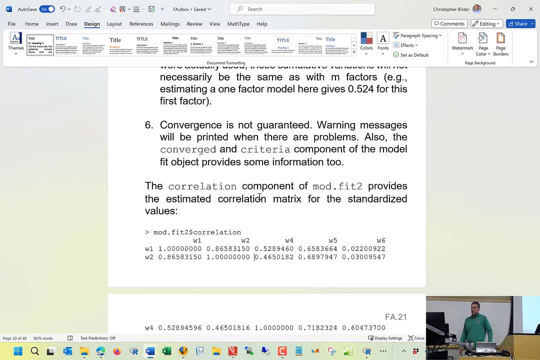 right. So I don't see, I don't think you know the reason for the factor. Well, okay, so I think you're getting at essentially well, why did I use two? Okay, And we're going to be looking at actually a hypothesis testing technique that will help us make that decision, instead of looking at the total variance. 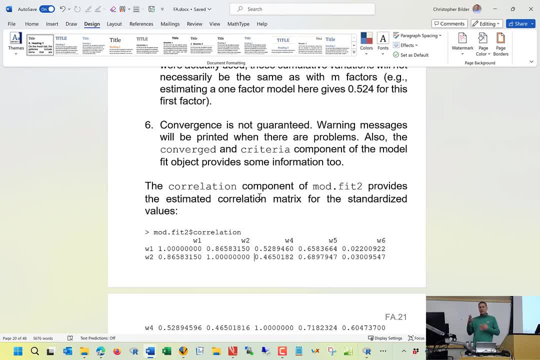 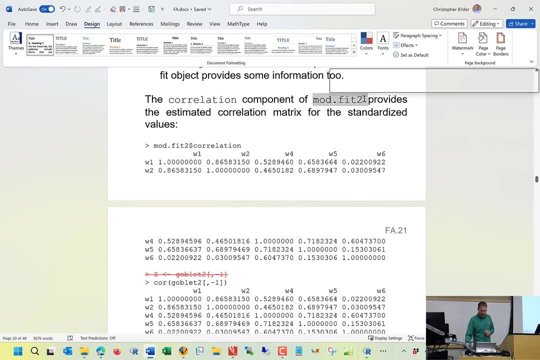 But also you've got to remember that factor analysis is not just concerned about the variances anymore. It's actually also interested in the associations as well. Okay, So that's why it's not necessarily as widely looked upon Now inside of modfit2, we have different components. 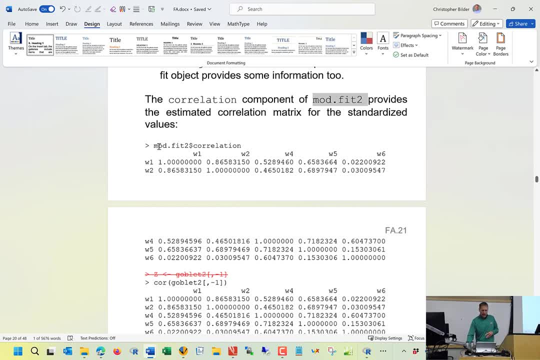 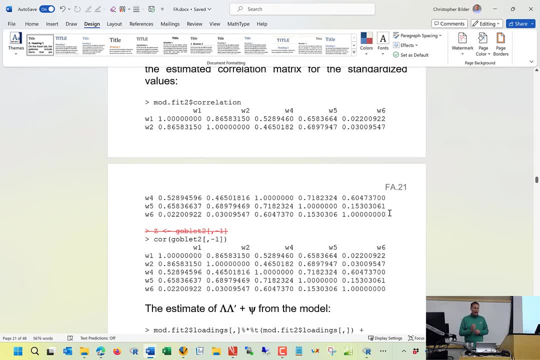 One of them actually ended up being correlation. So if I said modfit2 dollar sign correlation, I get the estimated correlation matrix, which will be exactly the same as if I use the core function itself. Okay, Note that there was a little bit of a typo in the notes. 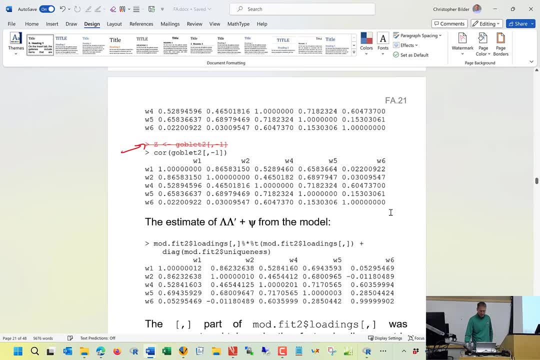 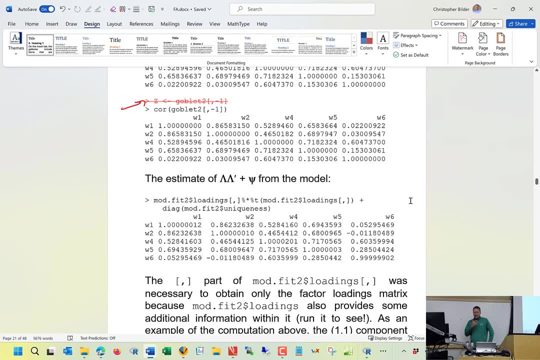 The program was fine, but the notes were not, And so what we might be interested in looking at, then, is as follows. You know, our factor analysis model says the correlation matrix should be equal to lambda. lambda prime plus psi. 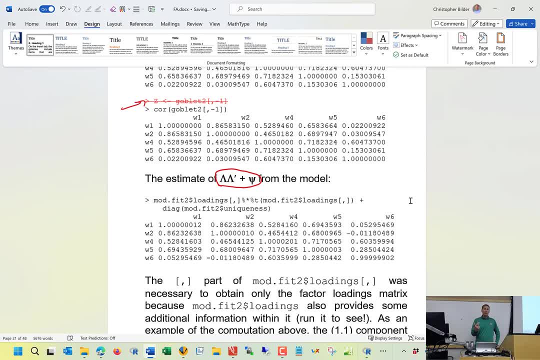 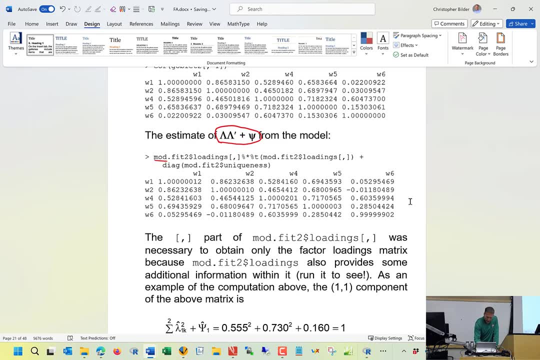 Well, how about we calculate the corresponding estimated values of this? So what I could do is I go to the, I go into modfit2, and if I look at the loadings component, I can pull out my lambda hat matrix. 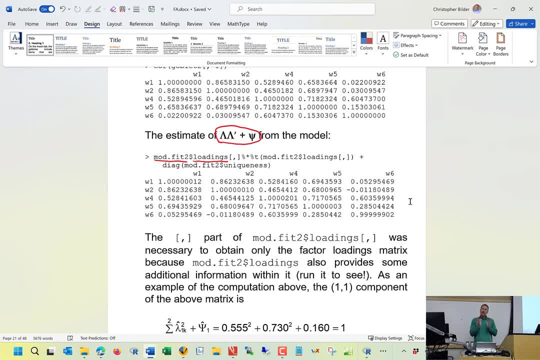 It's a little bit. they structure some stuff in a way that I don't like And if you remember, like if I had a matrix, let's call it A and R, you know, if I did one comma and then put nothing after that comma, inside of square brackets, 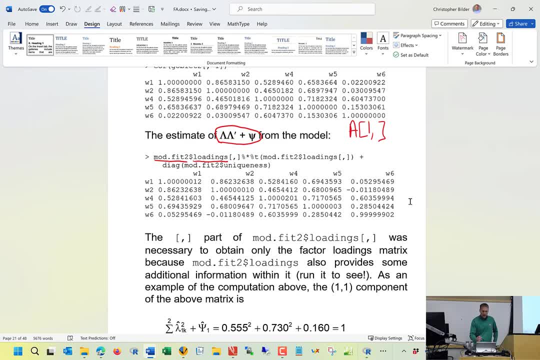 this gives me. this gives me my first call, I'm sorry, the first row. If instead I would have just comma one there, that gives me my first call. ah, comma, My first call If I actually put nothing in there. 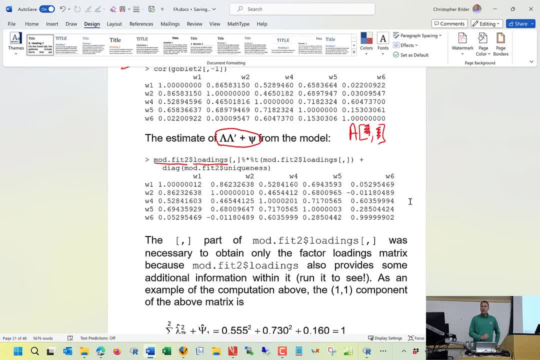 and just put a comma, I get the entire matrix. And you know, I urge you to after class on your own because we're running out of time. I don't want to go through the details, just execute that set of code. 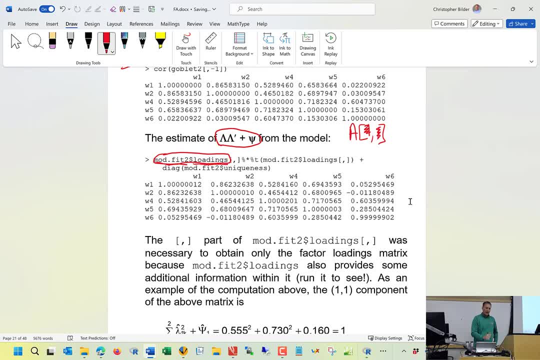 And you're going to get the factor loading matrix and some other stuff That we don't want, And so but if I just say mod dot, fit two dollar sign loadings- bracket, comma and bracket, I just get the matrix itself. 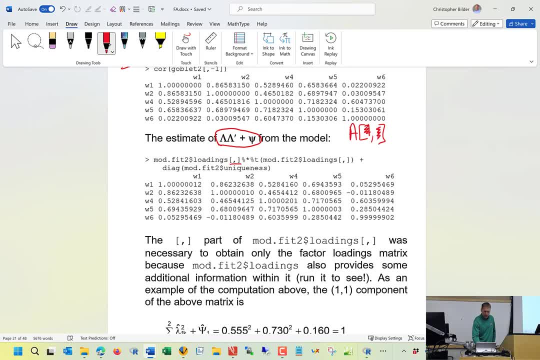 And so if I wanted to calculate lambda hat times, lambda hat prime, I use my matrix multiplication symbol and R to do the multiplication, And then I use the T function for transpose, And then I use the T function for transpose. 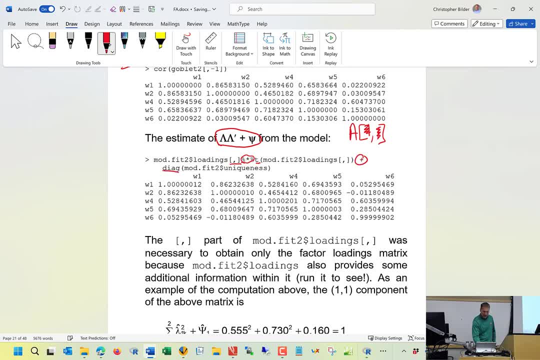 And then I can add to it a diagonal matrix that has all the specific variances. Remember again, uniqueness is a name for specific variances, And so in other words, I'm actually myself, you could say, manually calculating lambda hat times, lambda hat prime. 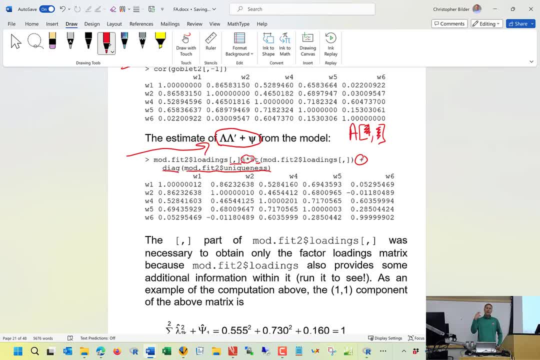 plus psi hat. If my model was perfect and everything that, everything in my data was explained by this, by this model, this matrix that I get in the end should be exactly the same as that. But we can see there are differences. 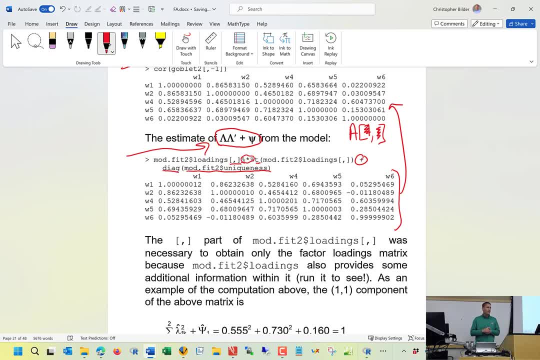 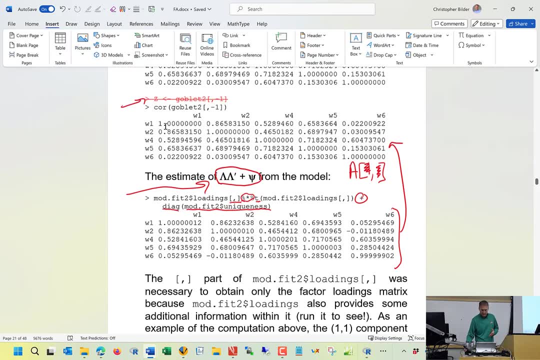 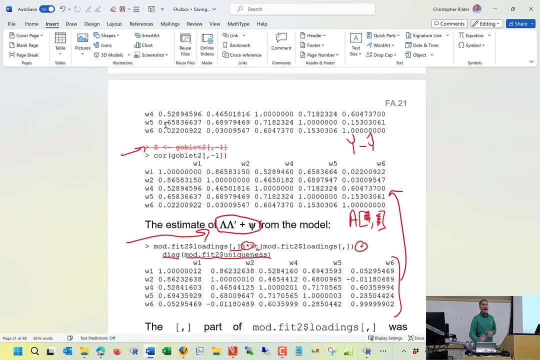 let's say your response variable was y, You would take y minus y hat, where y hat was the estimated value for your regression model And that's called your residual. You know you might have called it e, for example. It's a common notation. 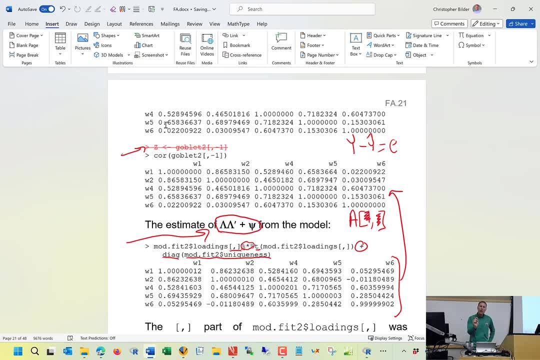 And you wanted those e's to be as small as possible, because that means that your model is fitting the data the best possible. If the e's were large, then that model's maybe not really doing a good job of fitting your data. 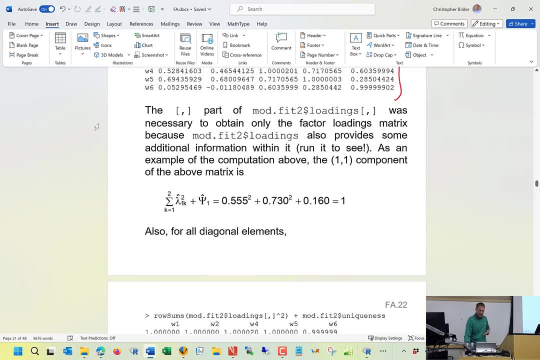 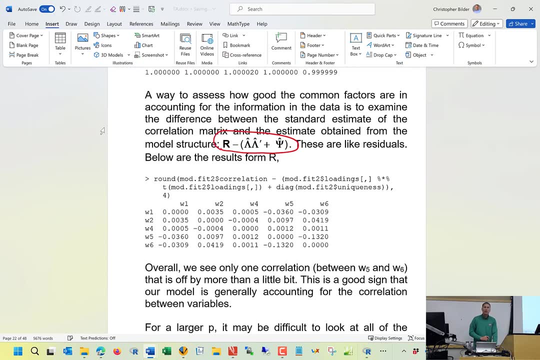 It's just not being predicted, And so what we could do then, in this particular case, is how about we take that estimated correlation matrix that you would normally, the normal way that you would estimate it, subtract off what we get from our model? 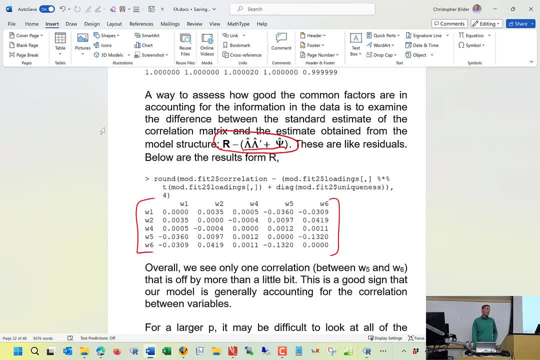 and now we have a version of factor analysis residuals. Just calculate it in a different way, But again, we want these residuals to be as close to zero as possible. The closer to zero, the better the model, And so we can see here that 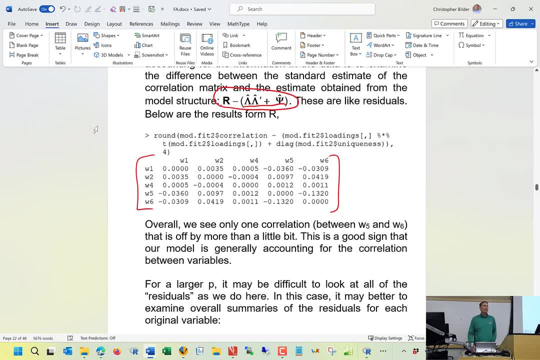 you know these values are fairly close to zero And remember, we're working with correlations here, so we have a numerical scale that we can kind of understand. You know correlations are between negative one and one. All these residuals are essentially close to zero. 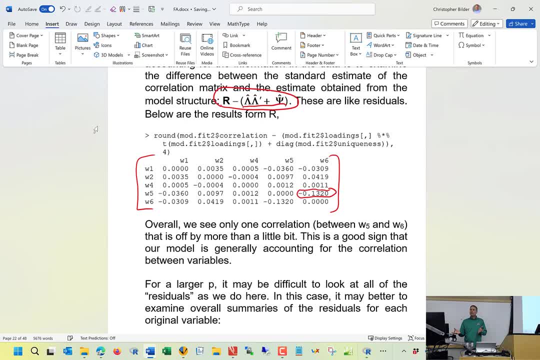 except for maybe one. Now, you know, think of it this way. So you might be thinking well, Chris. well, you know, you're off by negative .036 here for the correlation between W1 and W5.. How do I know if that's too big to? 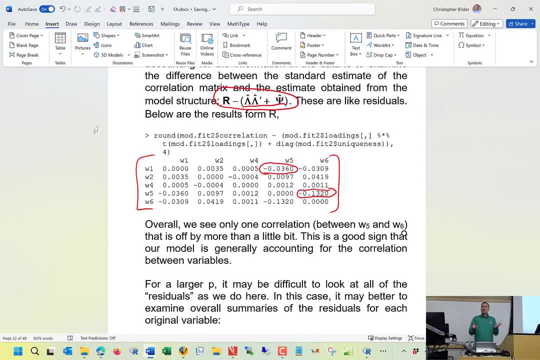 or if it's okay to represent. yeah, this is a good model. Well, you know, think of it, you know. let's say somebody told you the correlation between two things was .5. And then say, oh, whoops. 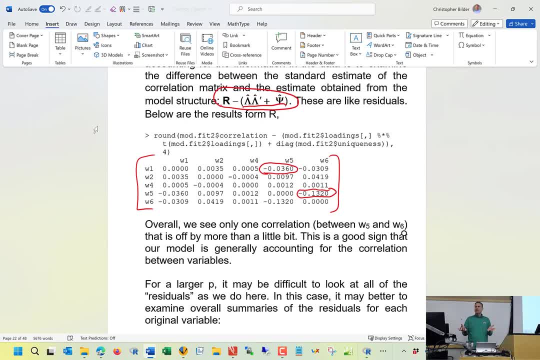 sorry, did that alarm you to see that much of a difference? Probably not. But if I have, let's say, .13,, well now you're, you know, difference between .5 and .63.. Well, okay, that's a little bit bigger. 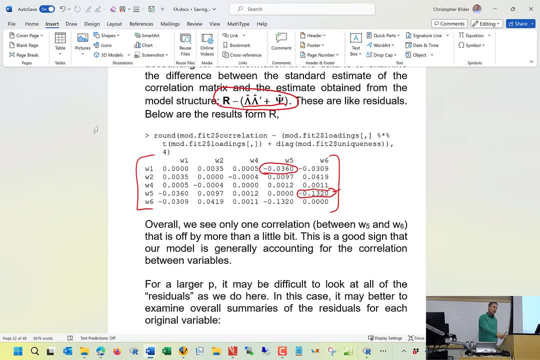 But if I told you- let's say someone said the difference- I told you the first time the correlation was .2, and now, the next time, I said it was .8.. Now you'd be worried. Okay, so think of that in your head when you're. 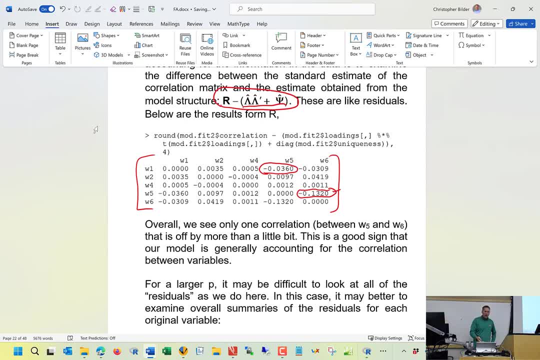 you know, trying to interpret these residuals. So over all here, this model seems decent. My only little bit of concern is that .13.. Otherwise, using this tool, I'm mostly satisfied with this model. Okay, so we're.